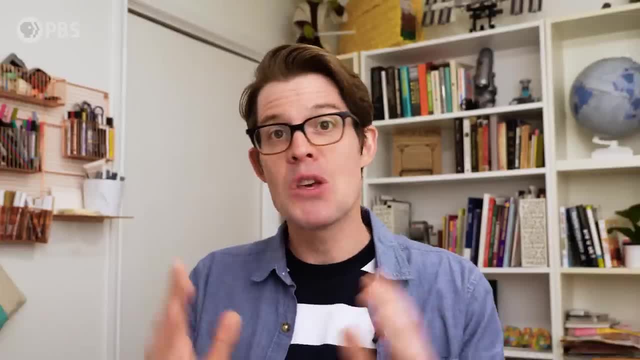 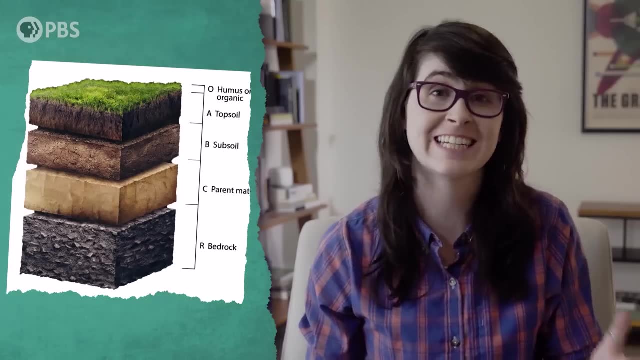 Well, what is the environment? Well, it's everything, and we humans depend on it for our literal existence. so don't you think you should learn a little more about it? In this series of lessons on environmental science, Miriam and I are going to explore. 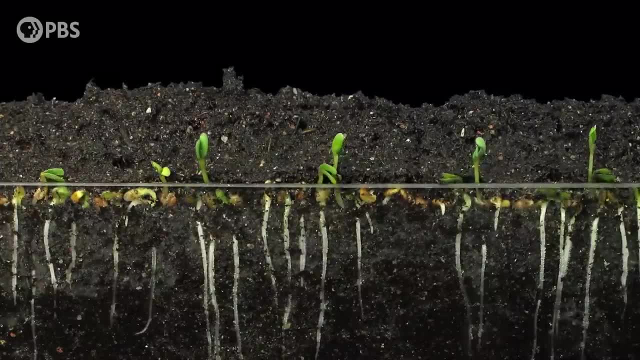 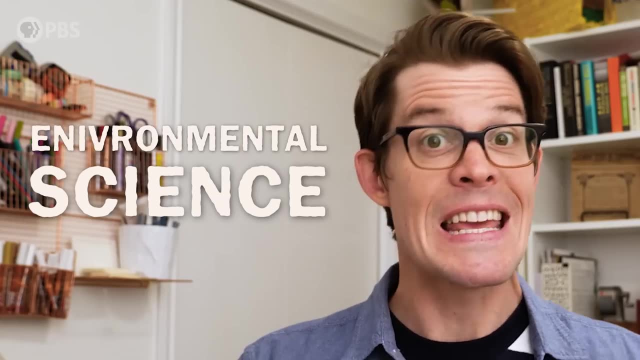 all the ways that humans interact with and rely on the environment. Welcome to the Essentials of Environmental Science. Environmental science is an interdisciplinary scientific field of research that focuses on the environment. Environmental science is an interdisciplinary scientific field of research that focuses on the environment. Environmental science is an interdisciplinary scientific approach to 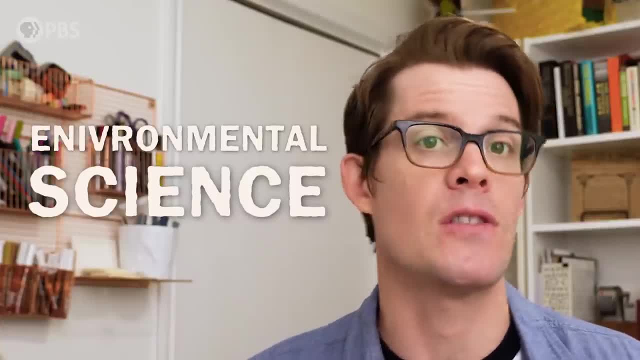 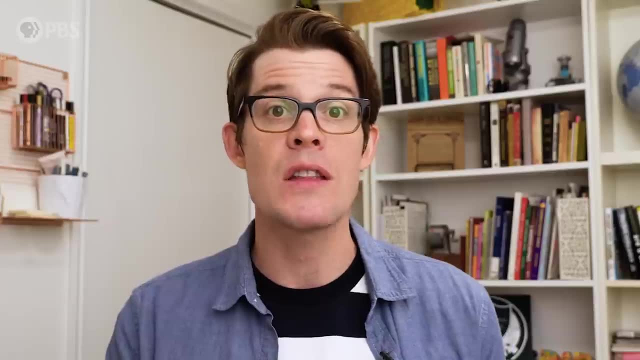 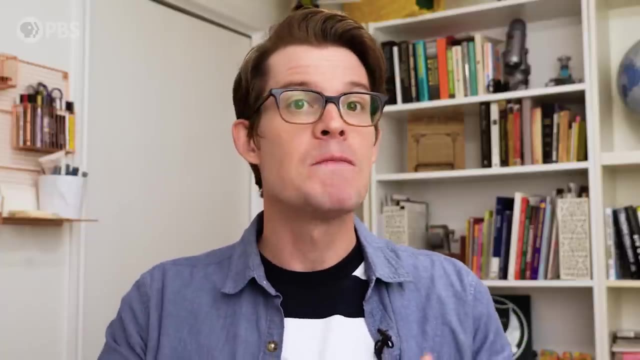 studying the Earth's natural systems, human impacts on those systems and potential solutions to environmental problems. People who work in the field of environmental science draw on aspects of biology, chemistry, economics, politics, human geography, urban planning. the list goes on. 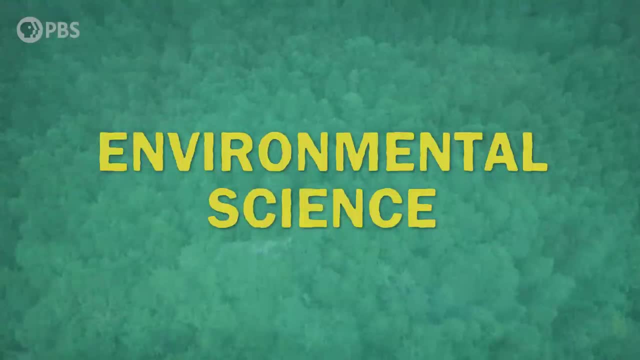 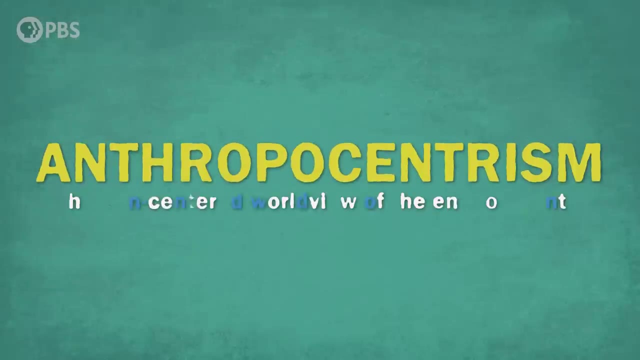 all in their study of the natural world. The scope of environmental science has steadily broadened over the last 100 years, starting from anthropocentrism, a human-centered worldview which has its roots in the European societies from which most modern scientific practices descend, then into biocentrism, which ascribes value to human. 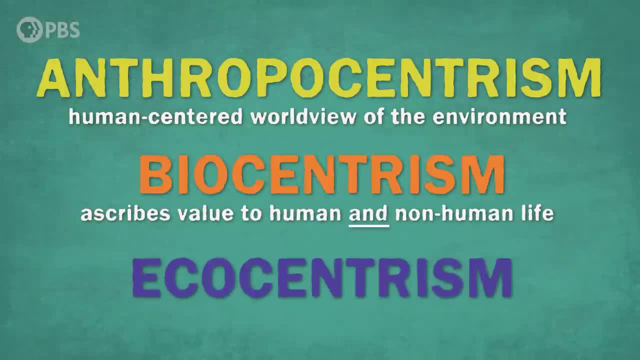 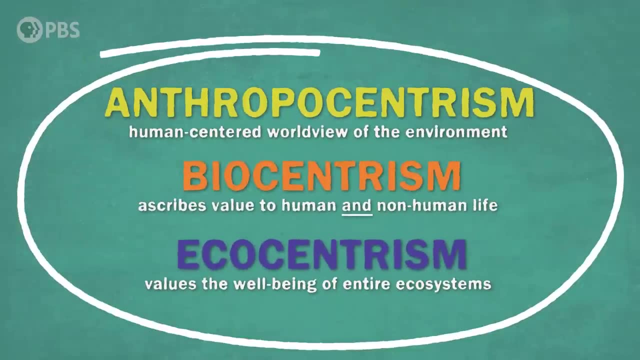 and non-human life. and finally, into ecocentrism, which values the well-being of entire ecosystems, including all the living and non-living elements. These three terms- anthropocentrism, biocentrism and ecocentrism- describe standards of environmental ethics depending on a culture's or a scientist's. 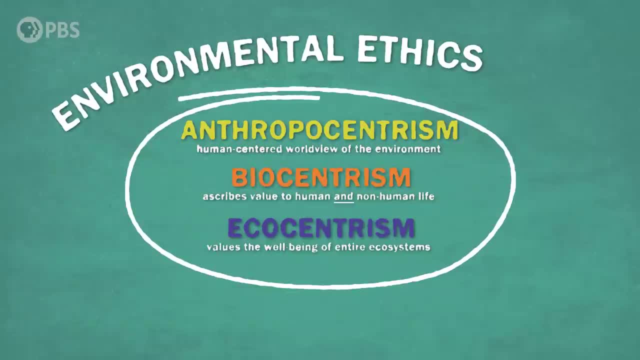 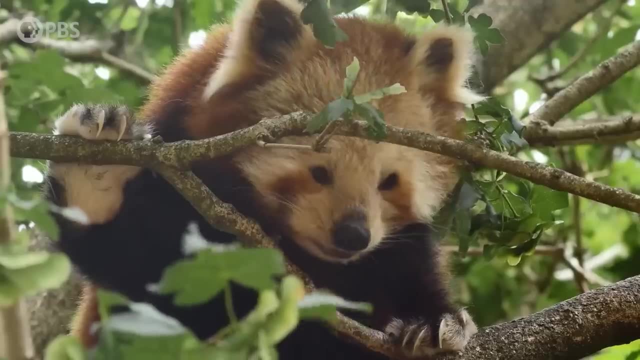 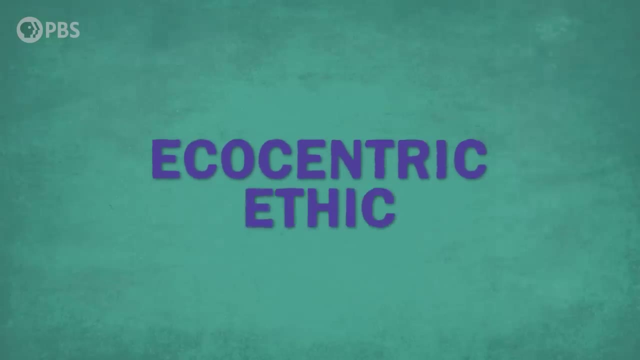 worldview. the environmental ethic will influence what questions are asked and what value we put on the answers. Today's environmental problems, from water pollution to endangered species, to climate change, all require us to look for answers through the broadest lens. the ecocentric ethic. 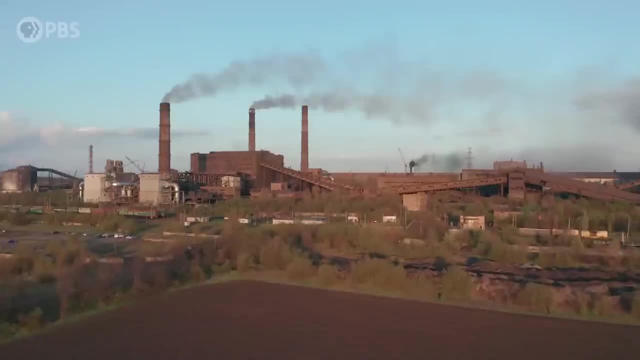 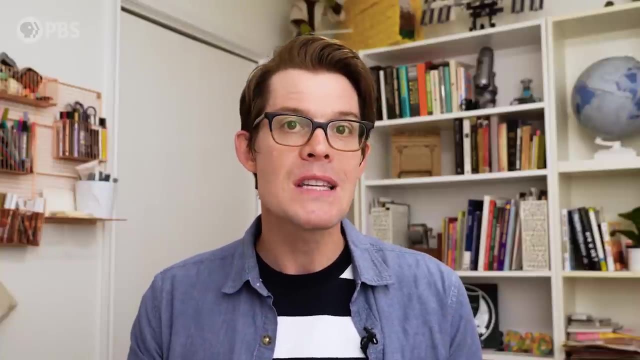 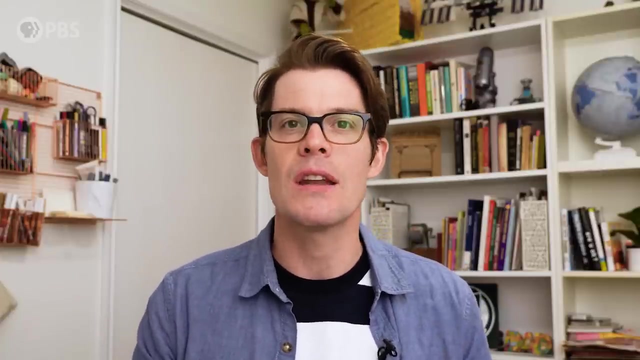 Humans have had a huge impact on our natural world, especially since the industrial revolution. To truly understand environmental systems and human impact, it's important to not simply study an organism like an endangered species or a pollution source like an oil spill, in isolation. 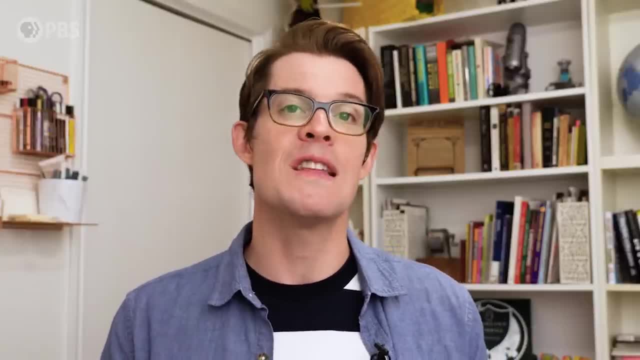 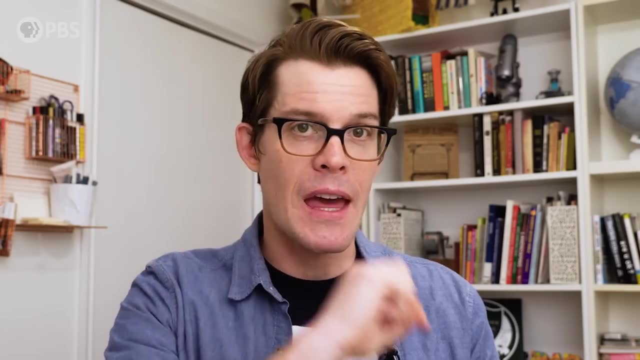 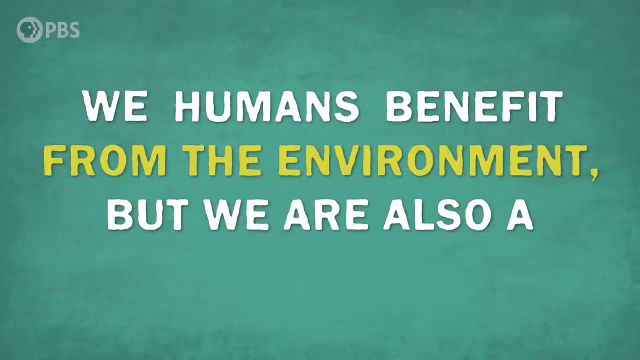 Instead, we should try to understand natural or human-caused disruptions to the environment from an ecocentric approach, by looking at the bigger systems at play. If you learn one thing from watching this series on environmental science, make it this: We humans benefit from the environment, but we're also a part of it. 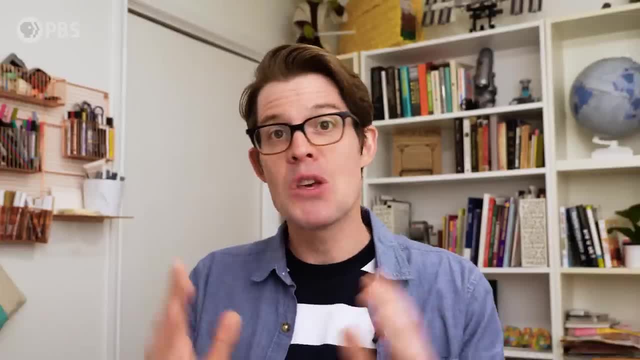 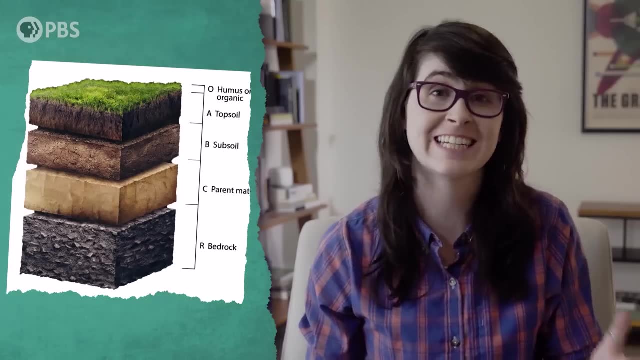 Well, what is the environment? Well, it's everything, and we humans depend on it for our literal existence. so don't you think you should learn a little more about it? In this series of lessons on environmental science, Miriam and I are going to explore. 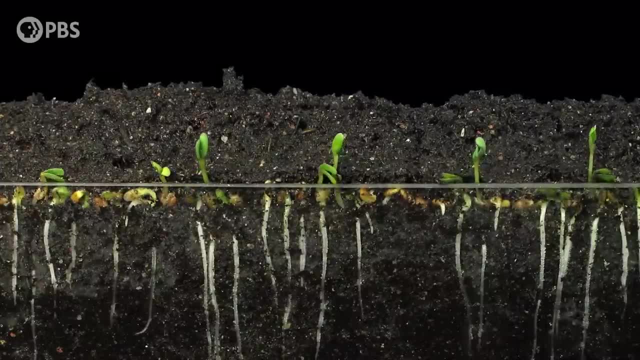 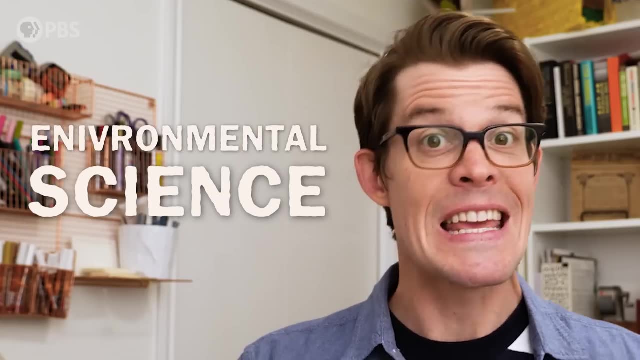 all the ways that humans interact with and rely on the environment. Welcome to the Essentials of Environmental Science. Environmental science is an interdisciplinary scientific field of research that focuses on the environment. Environmental science is an interdisciplinary scientific field of research that focuses on the environment. Environmental science is the scientific approach to studying the Earth's 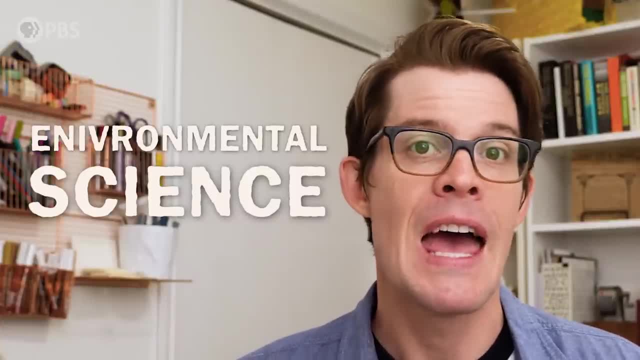 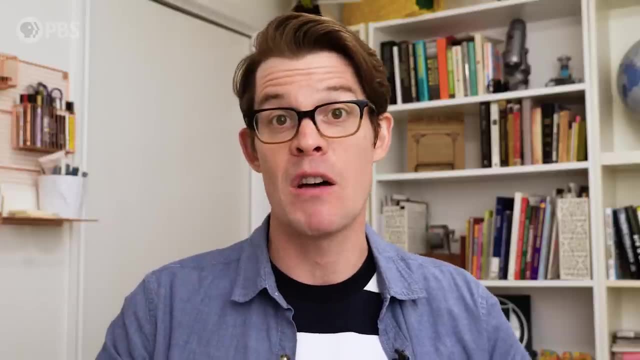 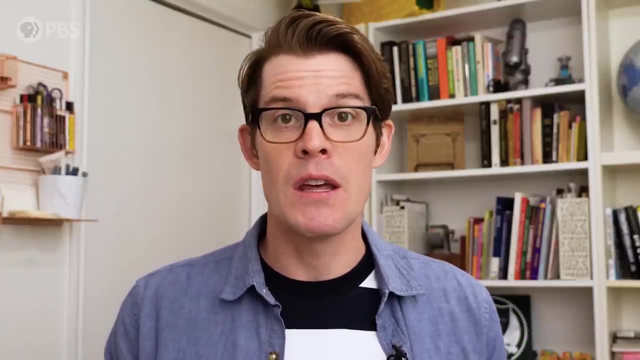 natural systems, human impacts on those systems and potential solutions to environmental problems. People who work in the field of environmental science draw on aspects of biology, chemistry, economics, politics, human geography and urban planning- the list goes on- All in their study of the natural world. The scope of environmental science has 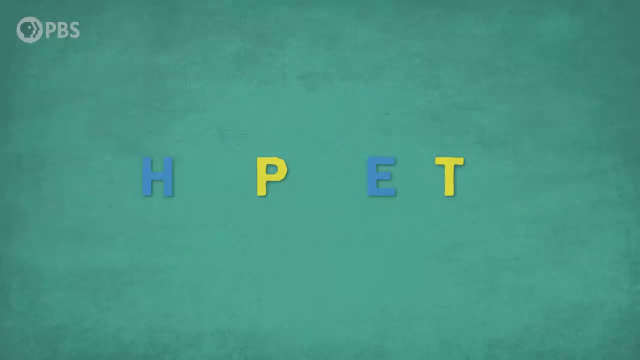 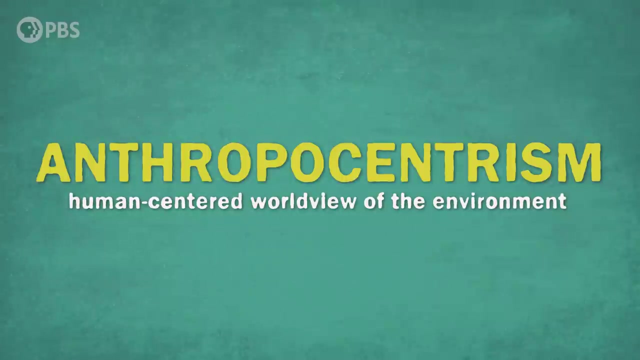 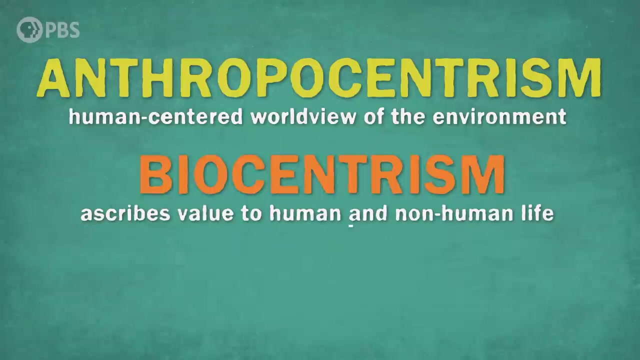 steadily broadened over the last 100 years, Starting from anthropocentrism, a human-centered worldview which has its roots in the European societies from which most modern scientific practices descend, then into biocentrism, which ascribes value to human and non-human life, and finally into ecocentrism, which values the well-being of 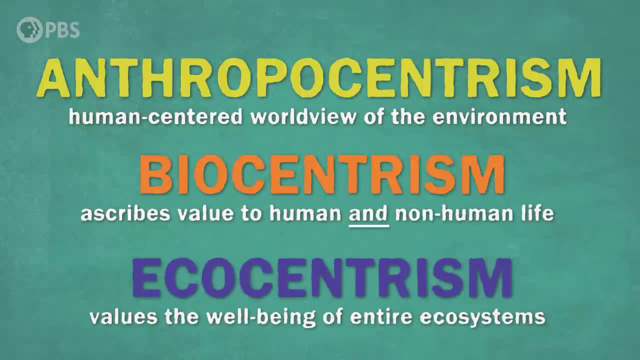 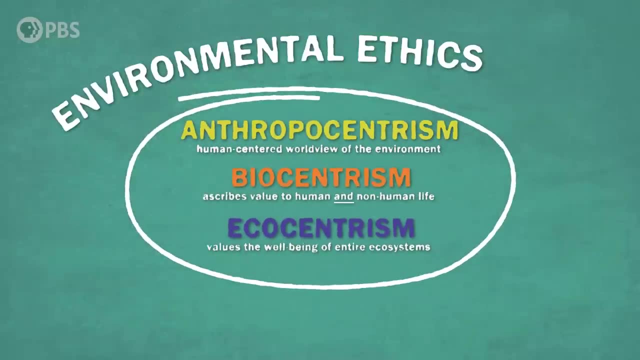 entire ecosystems, including all the living and non-living elements. These three terms- anthropocentrism, biocentrism and ecocentrism- describe standards of environmental ethics. Depending on a culture's or a scientist's worldview, the environmental ethic will influence. 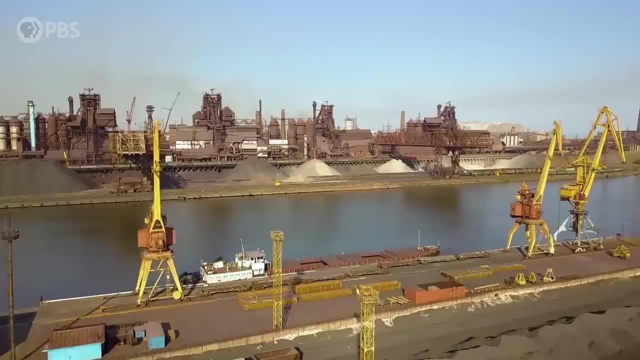 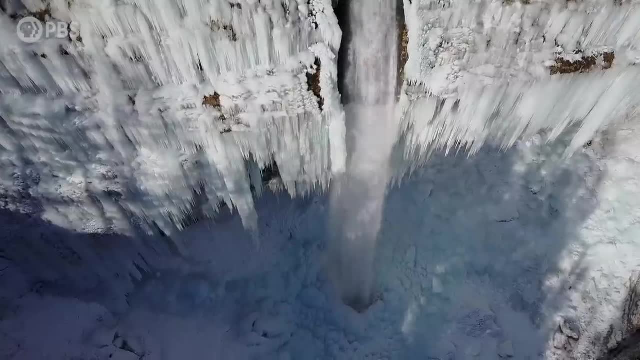 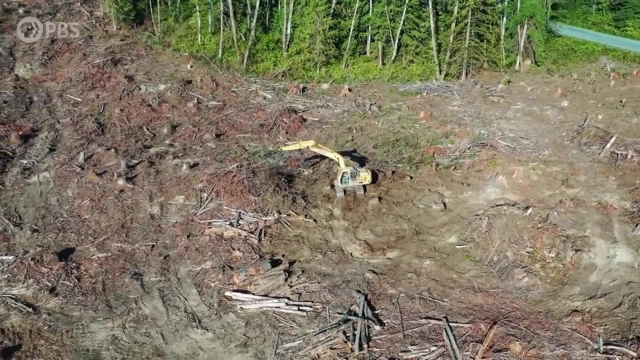 what questions are asked and what value we put on the answers. Today's environmental problems, from water pollution to endangered species, to climate change, all require us to look for answers through the broadest lens, the ecocentric ethic. Humans have had a huge impact on our natural world, especially since the industrial revolution. 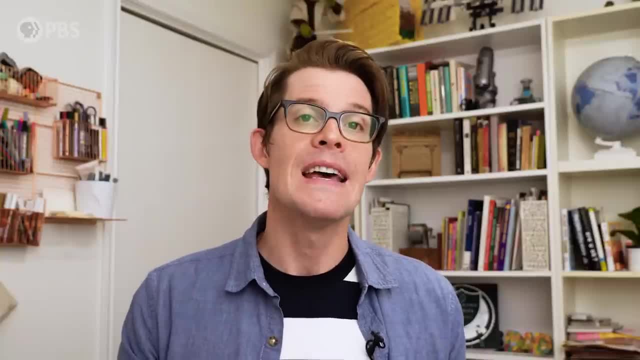 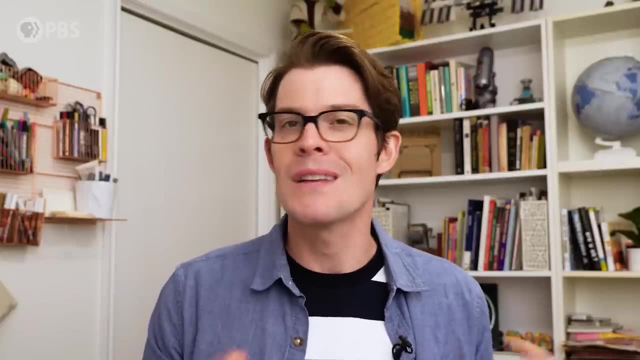 To truly understand environmental systems and human impact, we need to understand the environment. It's important to not simply study an organism like an endangered species or a pollution source like an oil spill, in isolation. Instead, we should try to understand. 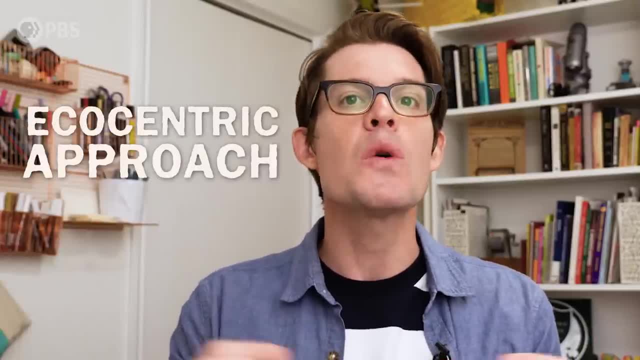 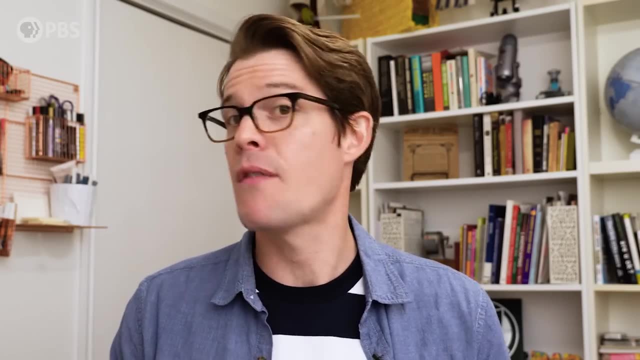 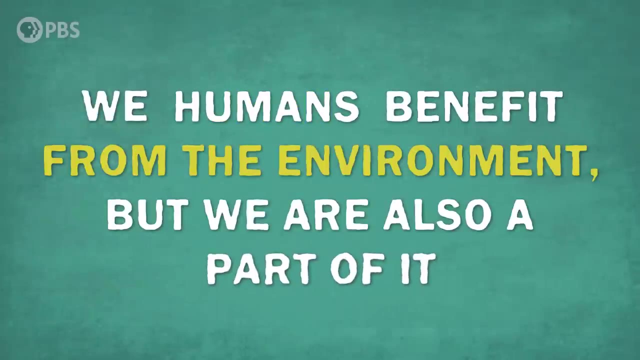 natural or human-caused disruptions to the environment from an ecocentric approach, by looking at the bigger systems at play. If you learn one thing from watching this series on environmental science, make it this: We humans benefit from the environment, but we're also a part of it. That means our. 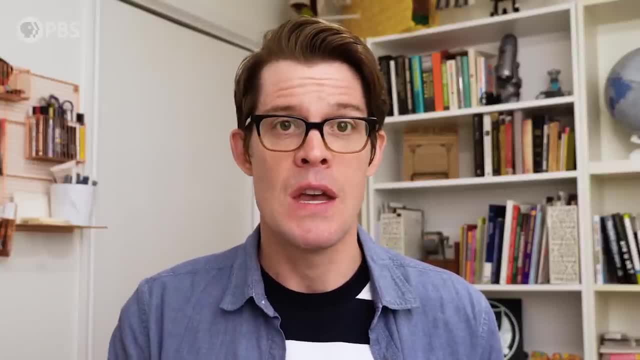 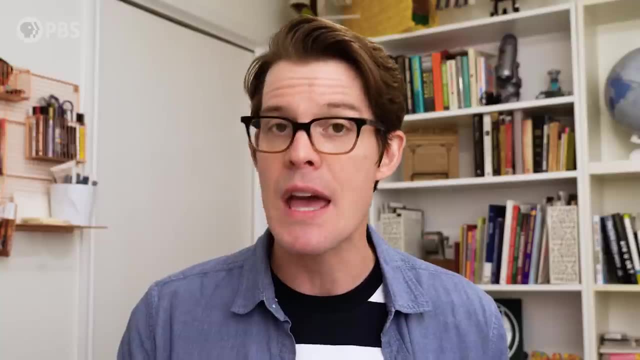 That means our actions can and do affect Earth's systems, So a lot of environmental science focuses on how to protect, preserve and restore the systems that human activity degrades. One way scientists do this is by constructing models to represent natural systems and all of 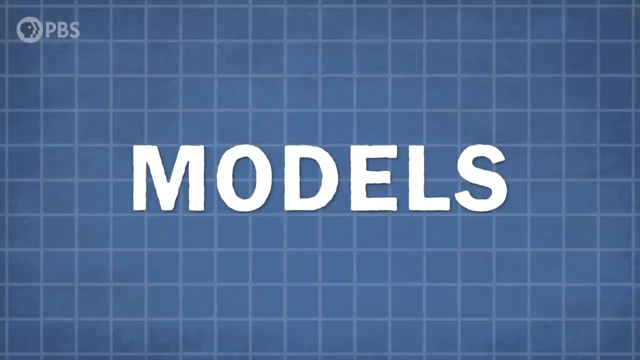 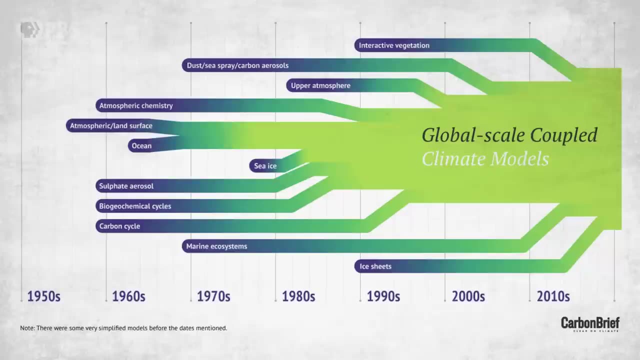 their interconnected factors. Models are powerful scientific tools with the ability to both explain and predict. A model could be code on a computer that recreates the physical processes of Earth's climate, but it could also be a chart or a graphic that represents the carbon cycle. 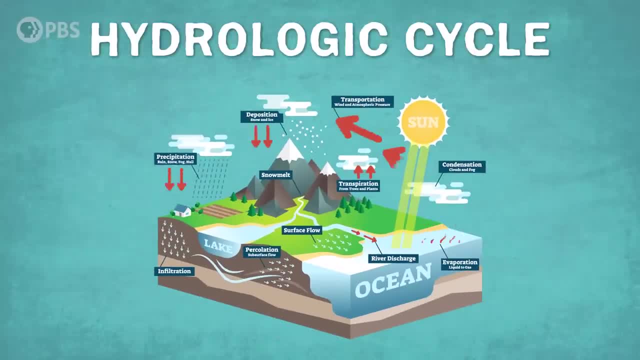 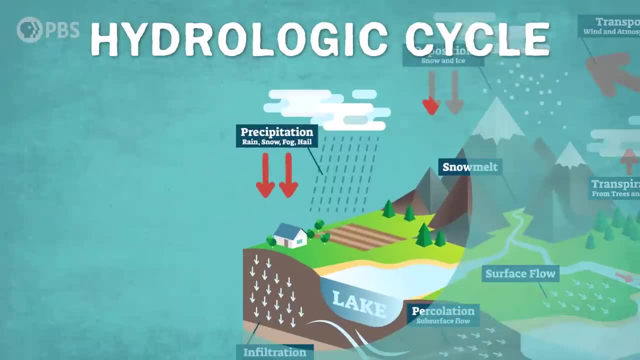 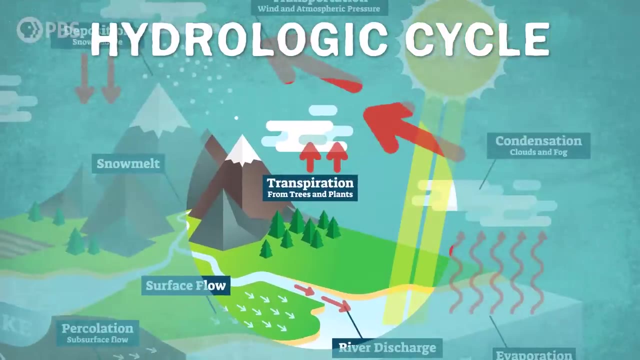 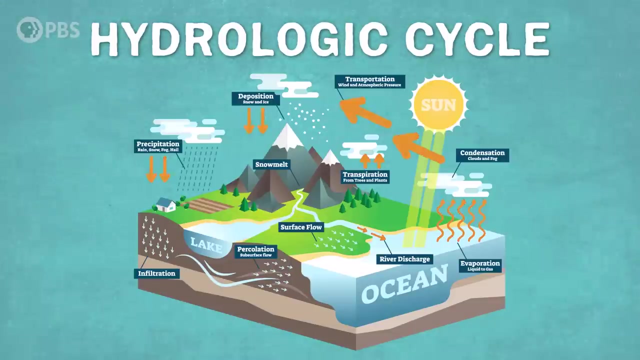 Here's a model of the planet Earth. This model represents all of these actions, with squiggly lines and raindrops. However, like any scientific model, it's not perfect. It cannot possibly represent everything going on at any one time. The only thing that can do that. 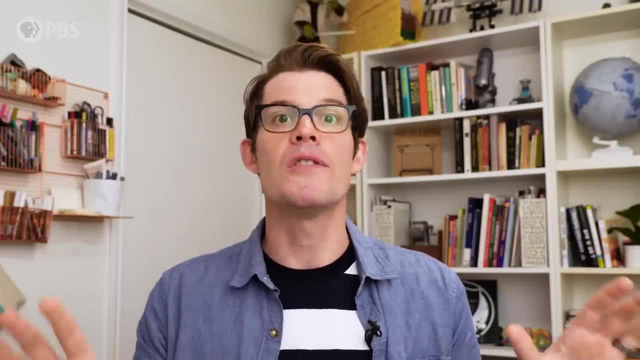 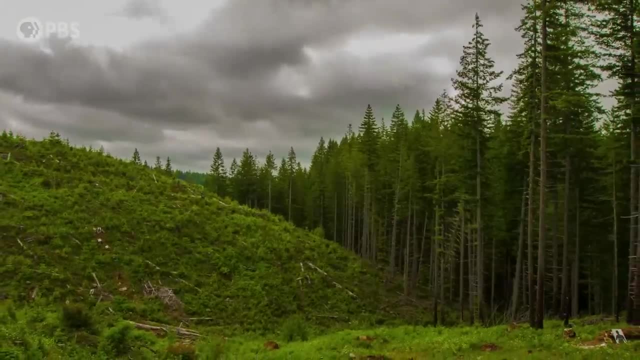 is the Earth itself. But even though we can't run global-scale experiments, a model does allow us to predict what would happen if something in the system changed. For example, if humans clear-cut a forest, this model would predict there will be less. 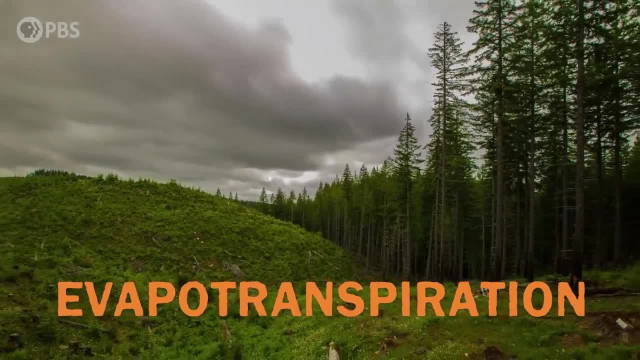 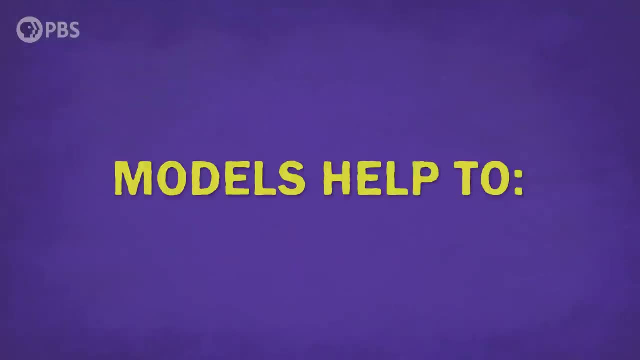 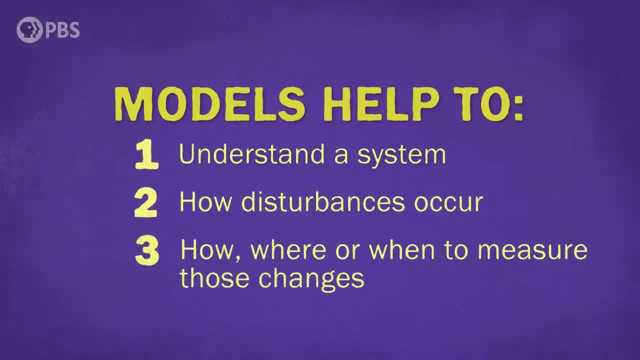 2. how natural the environment is, How natural and human disturbances occur, and 3. how, where or when to measure those changes. It's through this process that environmental science can analyze and address environmental problems. Now I know that I just said that you don't want to look at a single organism. 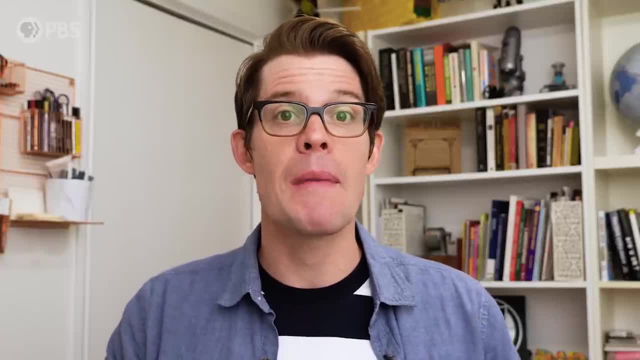 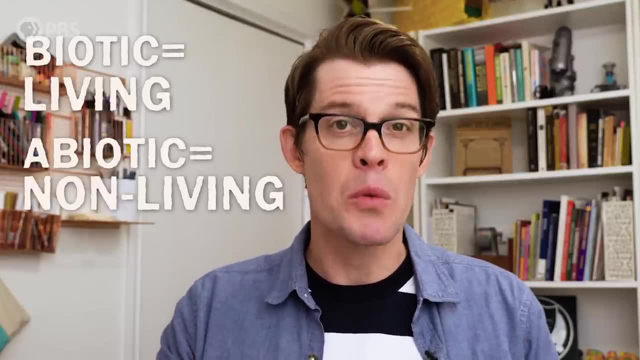 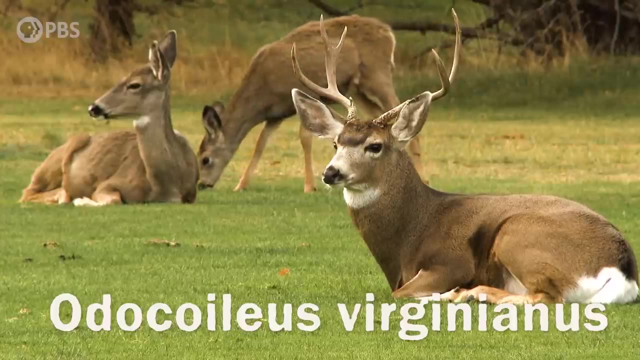 exclusively, but it's probably easier to start thinking about how biotic and abiotic or non-living components fit into a system by beginning with one example. Let's use a single white-tailed deer, a member of the species Otocoileus virginianus, to define some terms and look at how an ecosystem 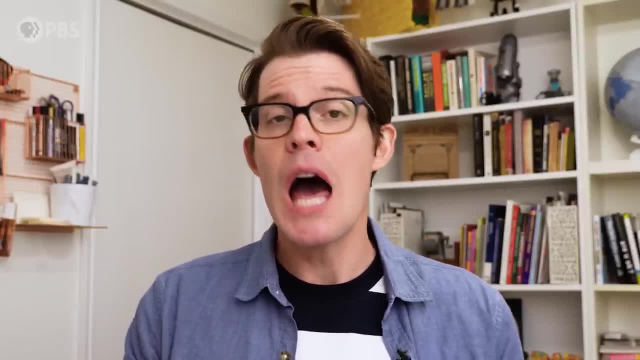 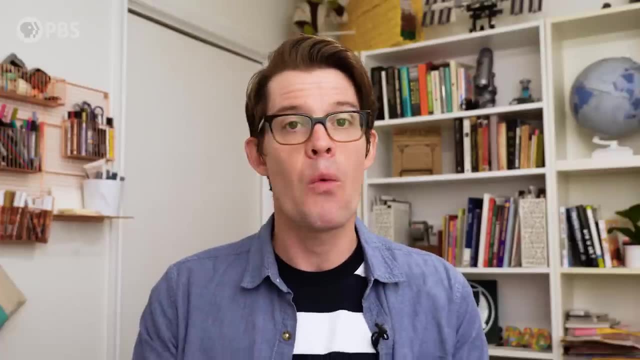 actions can and do affect Earth's environment, So let's look at some of the things that can and do affect Earth's environment. A lot of environmental science focuses on how to protect, preserve and restore the systems that human activity degrades. One way scientists do this is by constructing. 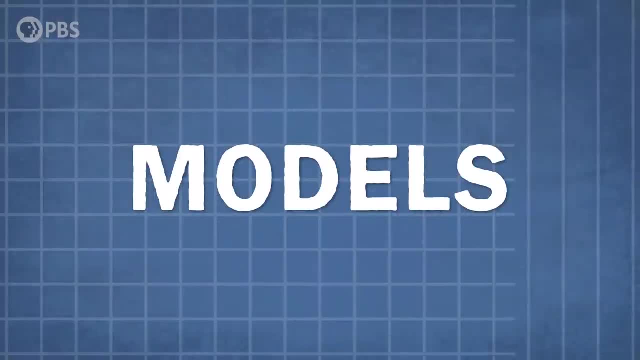 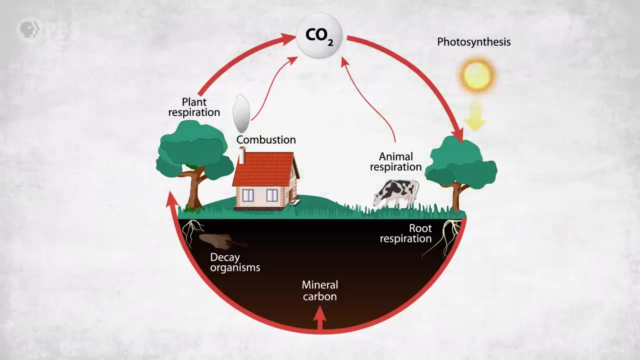 models to represent natural systems and all of their interconnected factors. Models are powerful scientific tools with the ability to both explain and predict. A model could be code on a computer that recreates the physical processes of Earth's climate, but it could also be a chart or a graphic that represents the carbon system. 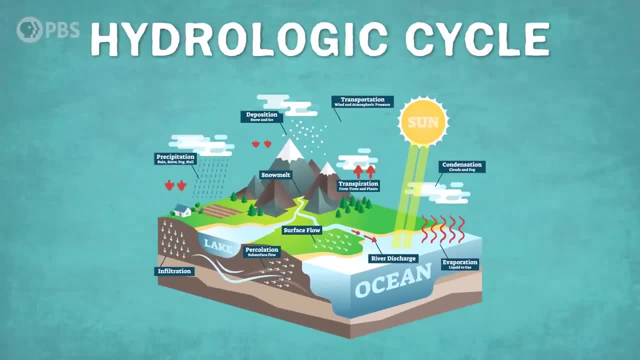 A model could be a graph or a graph that represents the carbon cycle. Here is a model of the planet's hydrologic cycle. Environmental science helps us to understand how all of the living and non-living components are interrelated. Rain falls into the surface. 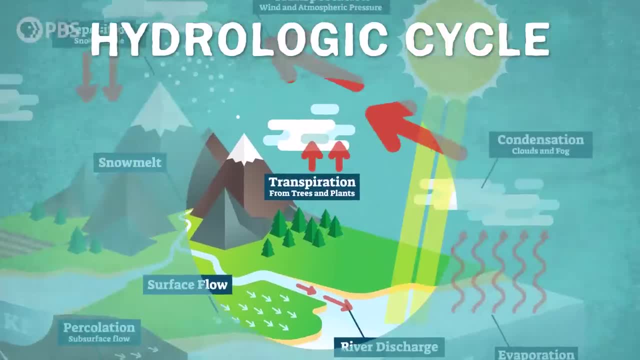 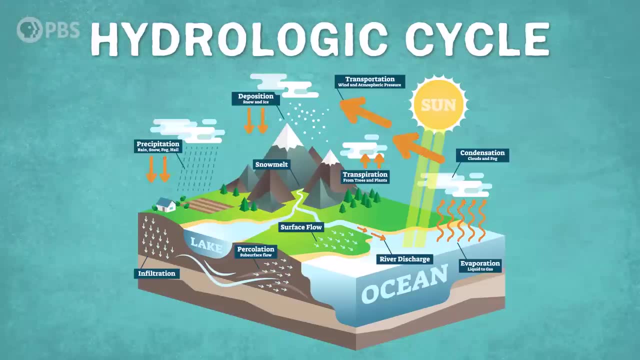 waters or the groundwater, or water can be taken up by plants for photosynthesis. This model represents all of these actions, with squiggly lines and raindrops. However, like any scientific model, it's not perfect. It cannot possibly represent everything going. 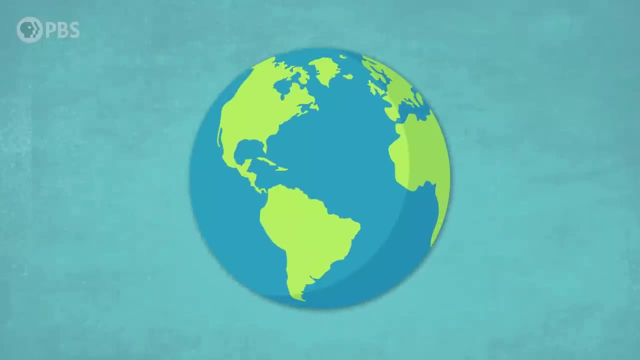 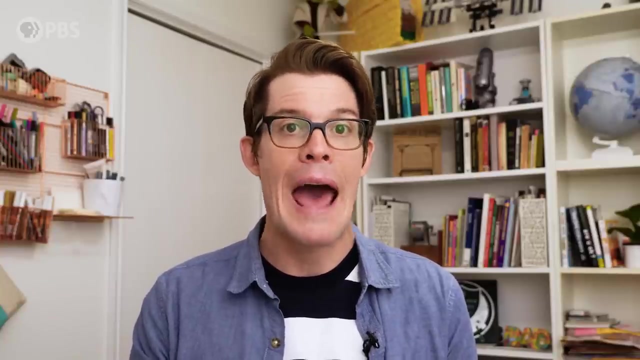 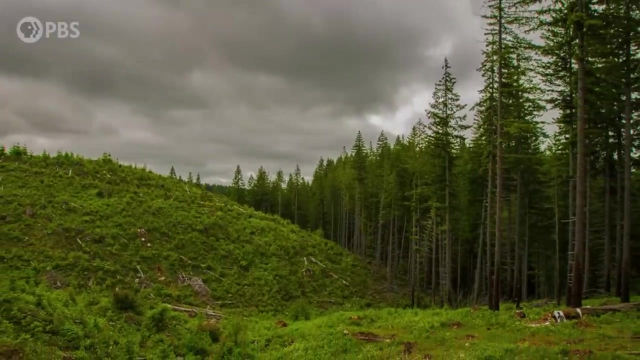 on at any one time. The only thing that can do that is the earth itself. But even though we can't run global scale experiments, a model does allow us to predict what would happen if something in the system changed. For example, if humans clear cut a forest, this model would predict there will. 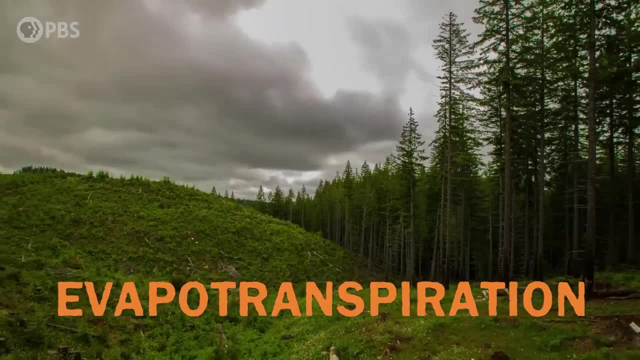 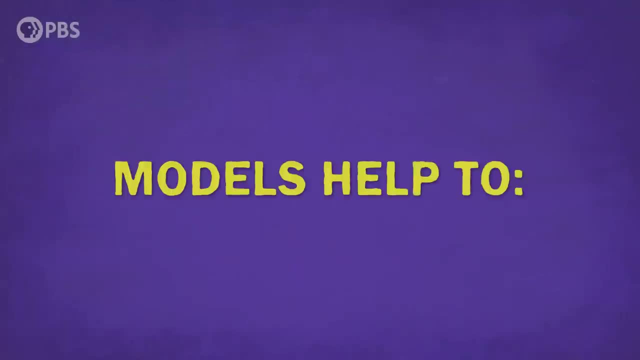 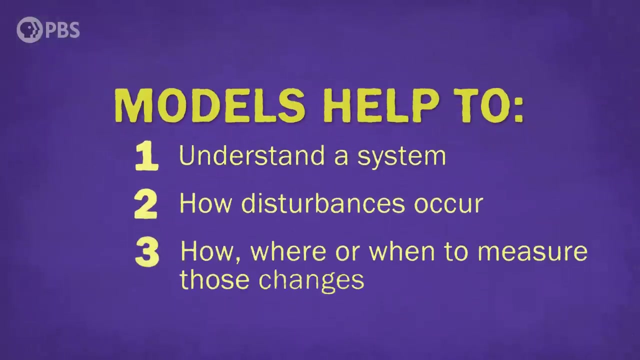 be less evapotranspiration from the trees into the atmosphere. We could then expect to measure less water vapor in the atmosphere around that location. So models help us to understand: one, a system. two, how natural and human disturbances occur. and three, how, where or when to measure. 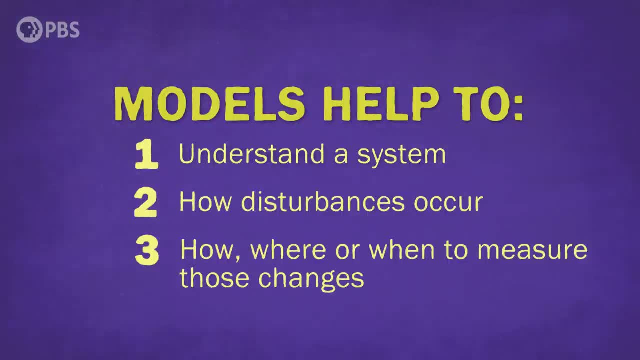 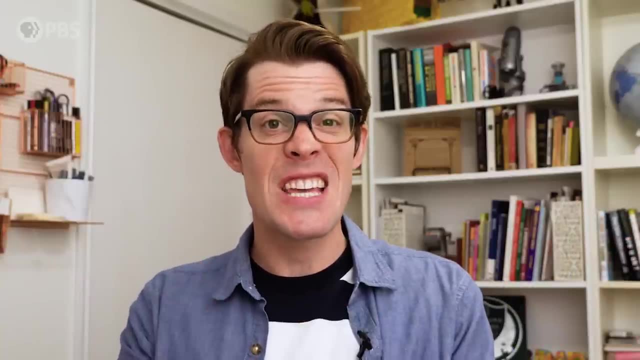 those changes. It's through this process that environmental science can analyze and address environmental problems. Now I know that I just said that you don't want to look at a single organism exclusively, but it's probably easier to start thinking about how biotic 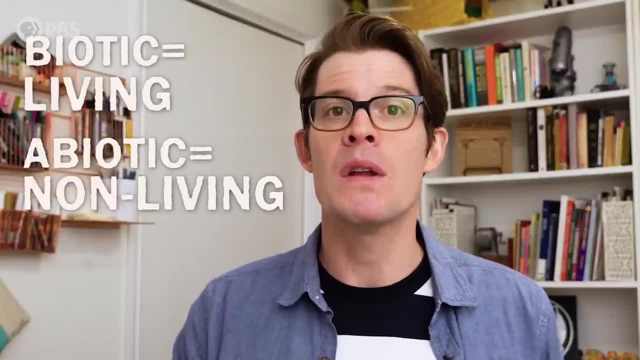 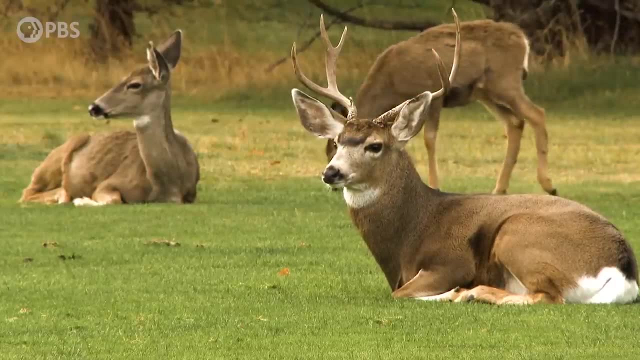 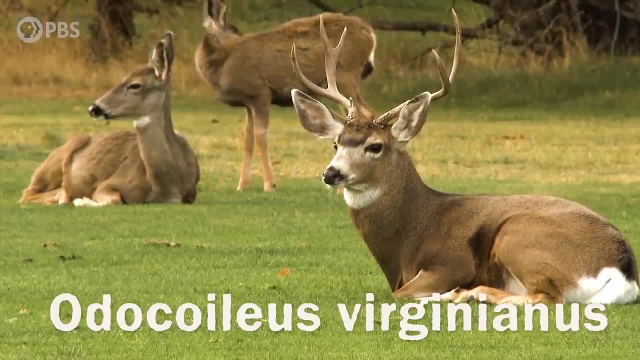 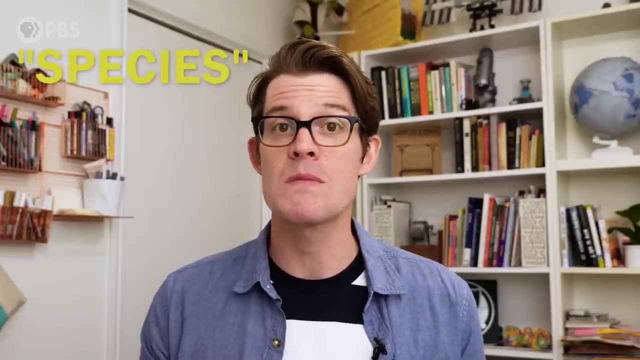 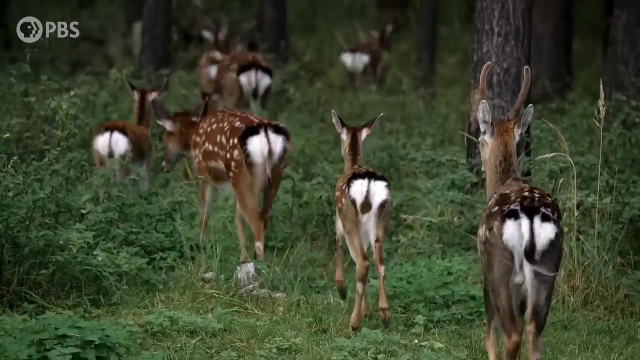 to define some terms and look at how an ecosystem works. Biologists define species in a number of ways, but one common definition of species is a group of organisms that can successfully reproduce with each other, A group of individuals of that species of deer living in a particular area. 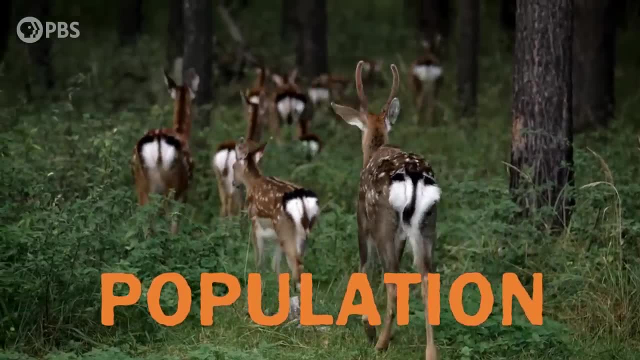 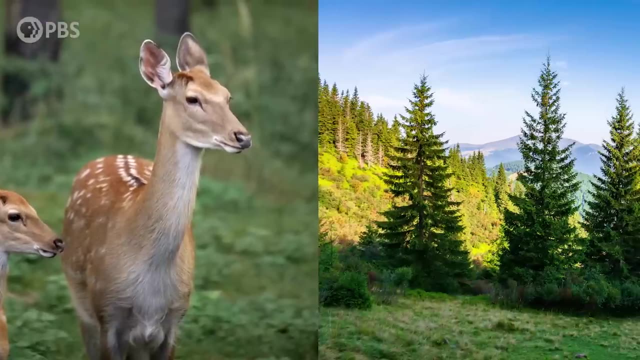 is called a population. But this population of deer isn't alone in some empty void. They're hanging out at the same time, in the same place with lots of other populations like pine trees, fungi, squirrels, bats- all that Together. an ecological community is a group of populations. 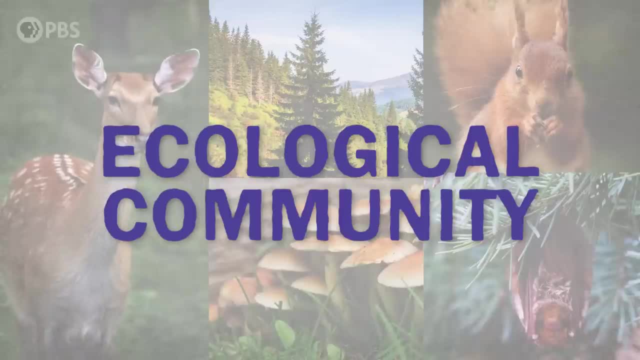 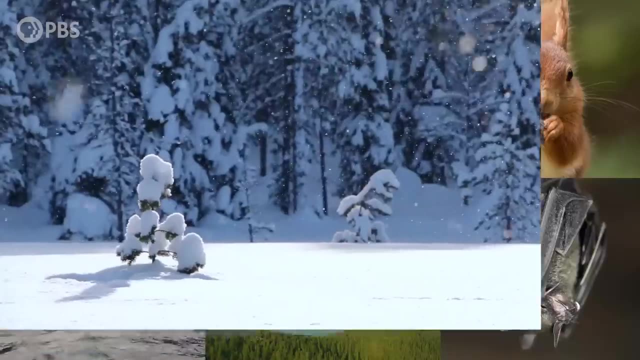 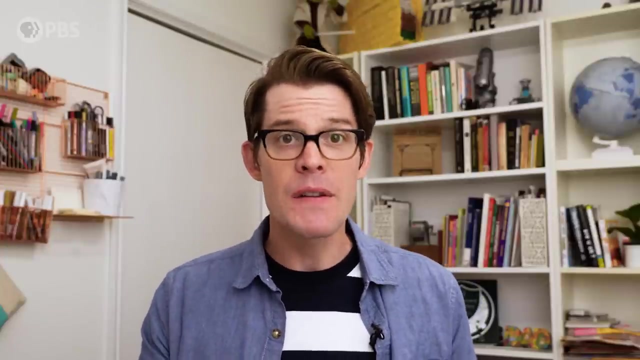 living in one area at a particular time, interacting with one another. If you add in all the abiotic components like the air, the rocks, water, even something like the temperature, then you've got an ecosystem. When studying a single species like a white-tailed deer or an African elephant, 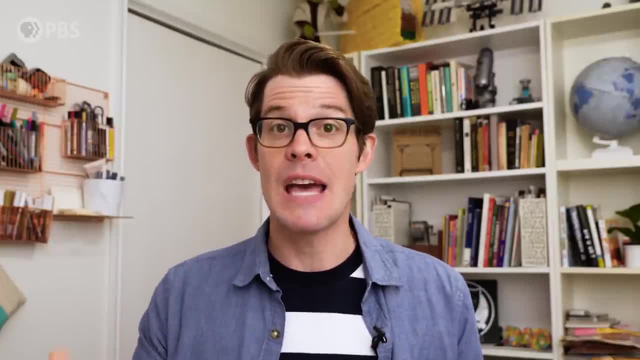 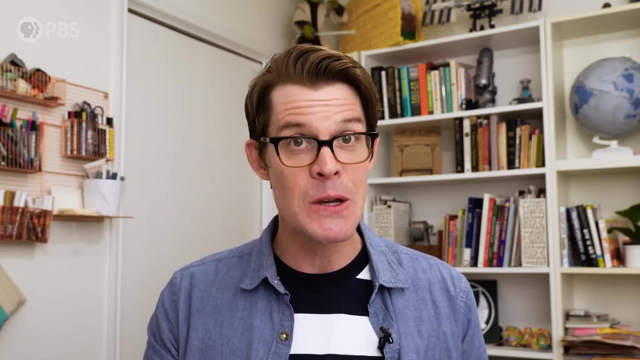 nothing works in isolation. Therefore, we can't study anything in isolation. So researchers need to consider all the abiotic and biotic components of that species and its ecosystem together. Think about it: Organisms in a tropical rainforest have adapted to different 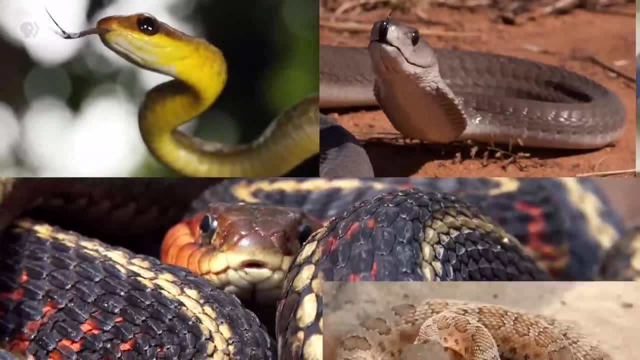 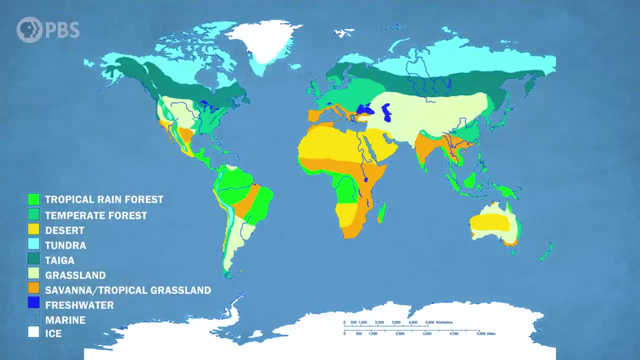 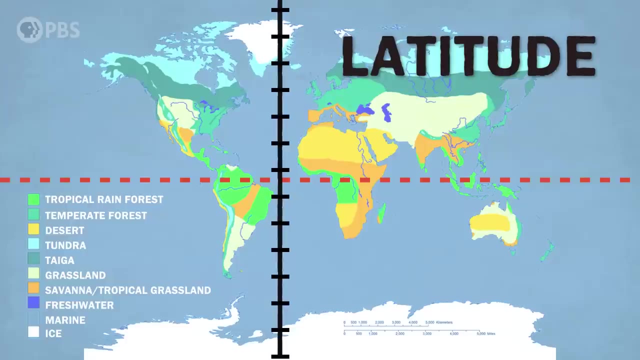 conditions than those in a savanna or a tundra or a desert or in temperate grasslands, We call all of these different broad regions of the planet that are defined by patterns of rainfall and temperature: biomes, Latitude, the distance north or south from the equator can be a really useful tool in determining 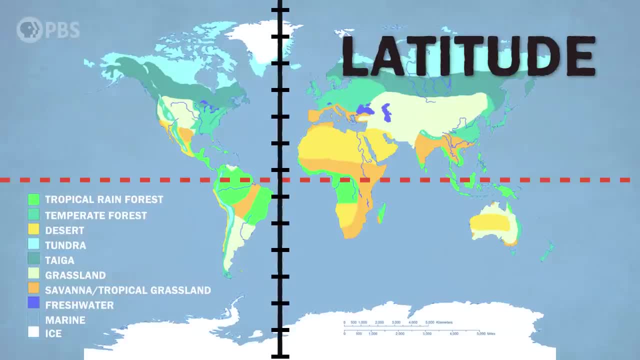 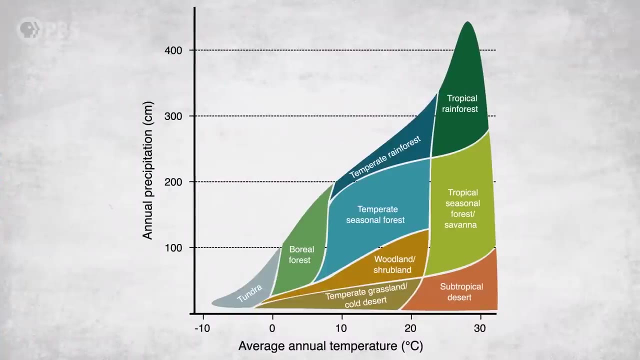 where certain biomes exist. It's no surprise that the hot, humid conditions all along the equator created tropical rainforest biomes around the world. At higher latitudes, the cooler parts of the world, you're more likely to find biomes like tundra or the boreal forest. This graph created 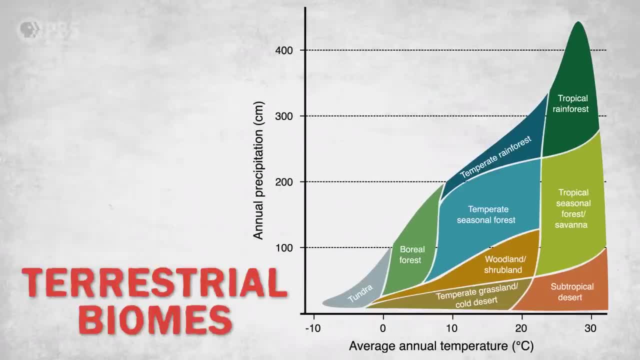 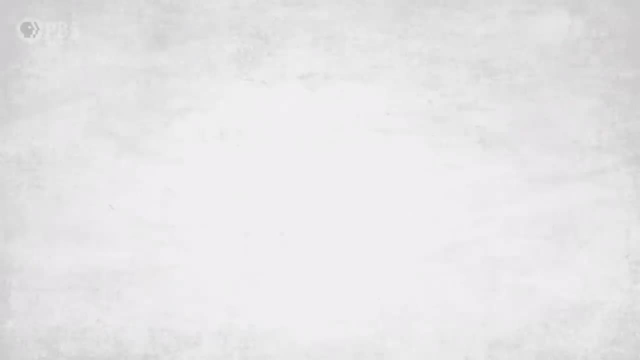 by the scientists represents the different major terrestrial biomes. The y-axis is the average precipitation and the x-axis is average temperature. Whittaker's graph works because terrestrial biomes are mainly defined by their temperature and precipitation patterns. However, this doesn't tell us much about the wide variety of aquatic ecosystems that exist in oceans. 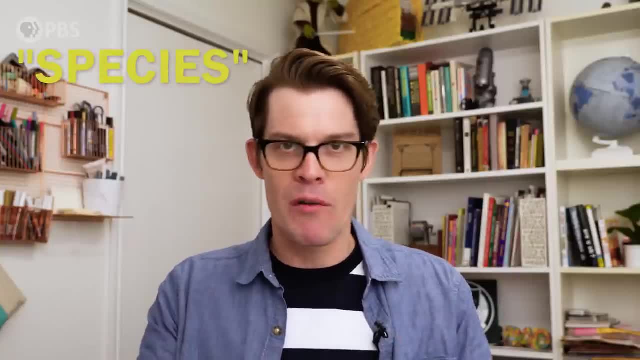 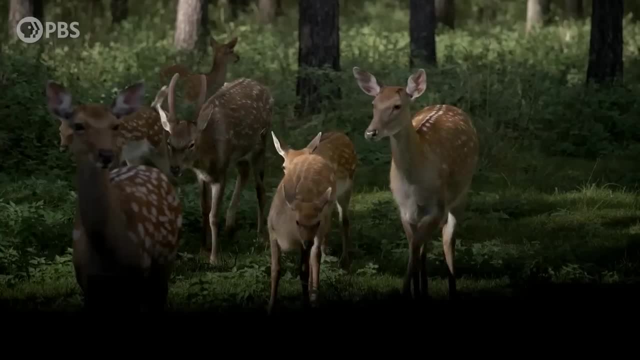 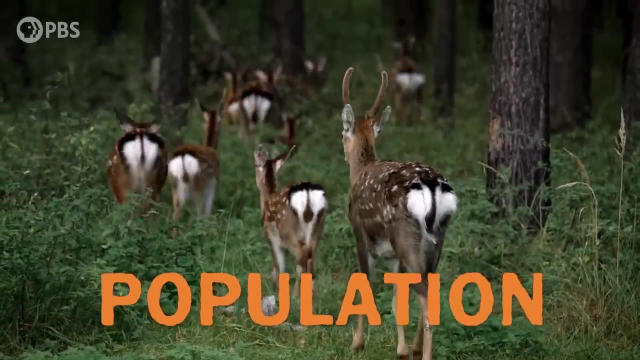 works. Biologists define species in a number of ways, but one common definition of species is a group of organisms that can successfully reproduce with each other. A group of individuals of that species of deer living in a particular area is called a population. But this population 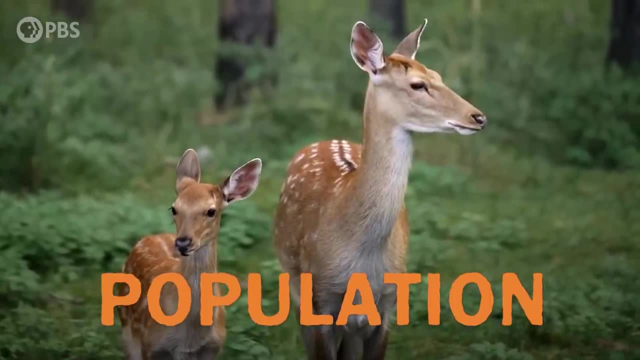 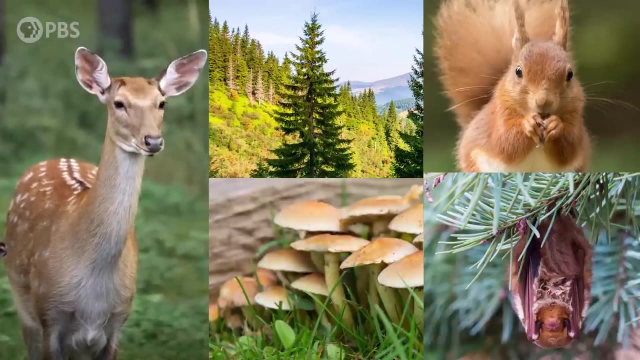 of deer isn't alone in some empty void. they're hanging out at the same time, in the same place, with lots of other populations like pine trees, fungi, squirrels, bats, all that Together. an ecological community is a group of populations living in one area, at a particular. 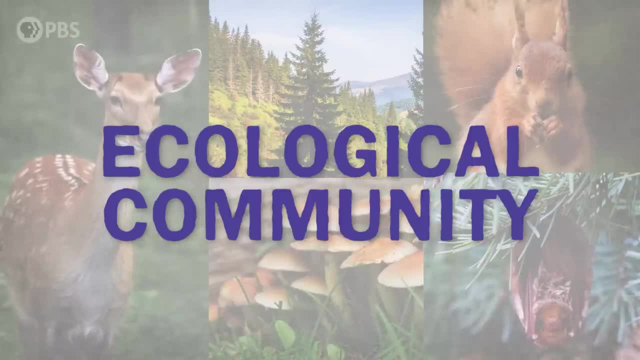 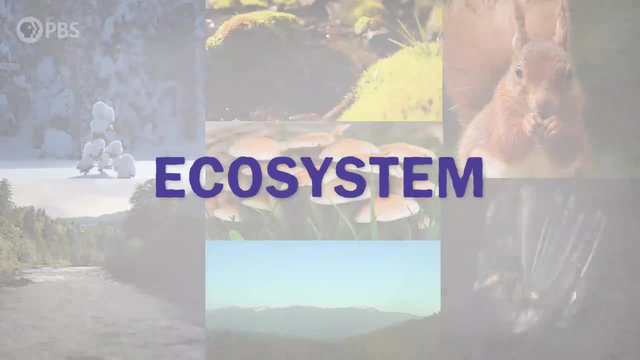 time interacting with one another. If you add in all the abiotic components, like the air, the rocks, the water, even something like the temperature, then you've got an ecosystem. When studying a single species like a white-tailed deer or an African elephant, 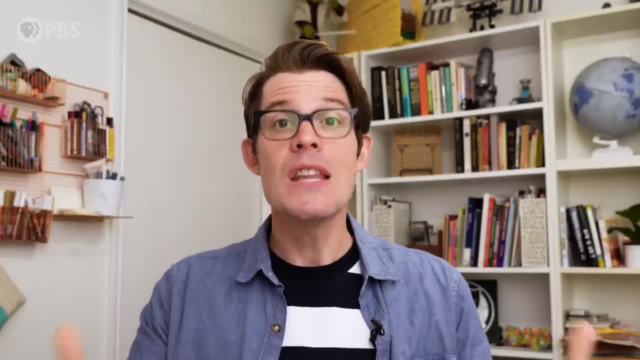 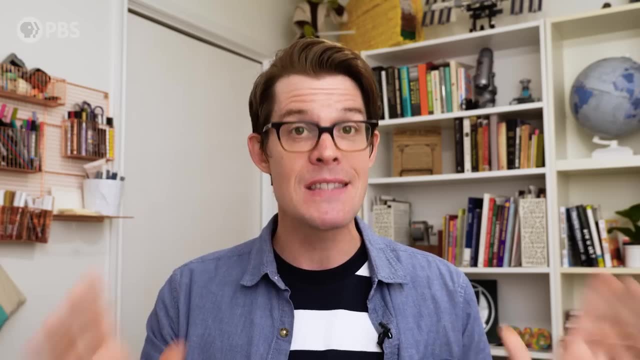 nothing works in isolation. Therefore, we can't study anything in isolation. So researchers need to consider all the abiotic and biotic components of that species and its ecosystem together. Think about it: Organisms in a tropical rainforest have adapted to different 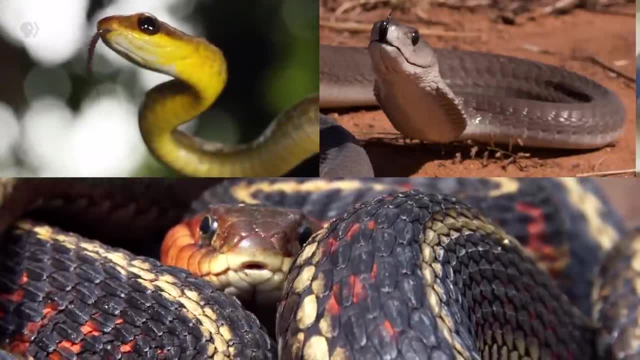 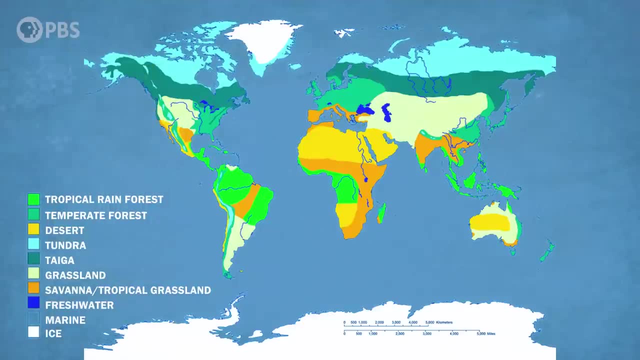 conditions than those in a savanna or a tundra or a desert, or in temperate grasslands. We call all of these different broad regions of the planet that are defined by patterns of rainfall and temperature, biomes, Latitude, the distance north or south of the. 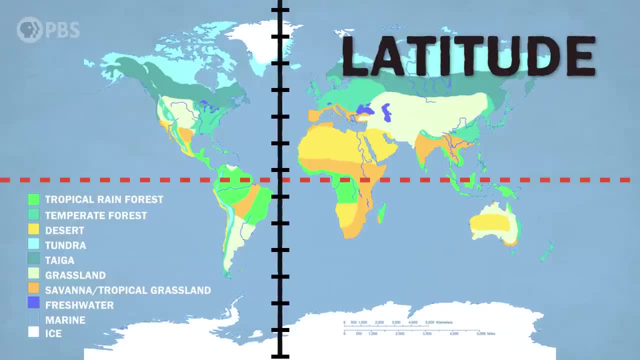 equator can be a really useful tool in determining where certain biomes exist. It's no surprise that the hot, humid conditions all along the equator created tropical rainforest biomes around the world. At higher latitudes, the cooler parts of the world, you're more likely to 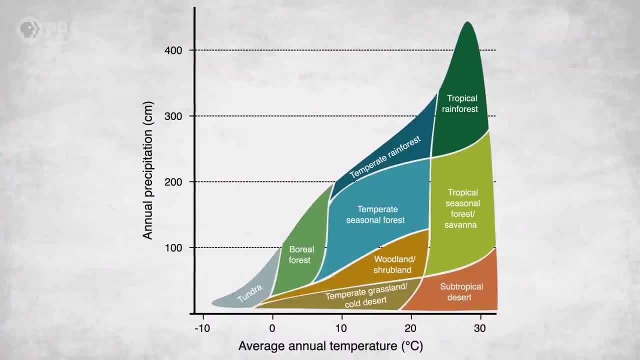 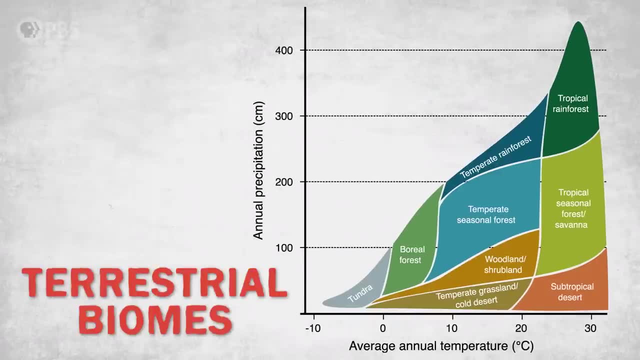 find biomes like tundra or the boreal forest. This graph, created by ecologist Robert Whitaker, represents the different major terrestrial biomes. The y-axis is the average precipitation and the x-axis is the average precipitation. The y-axis is the average precipitation and the x-axis. 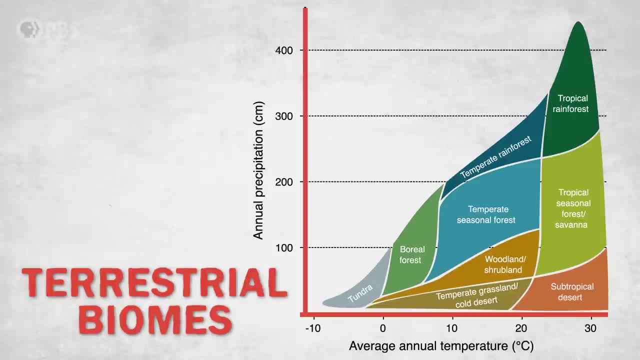 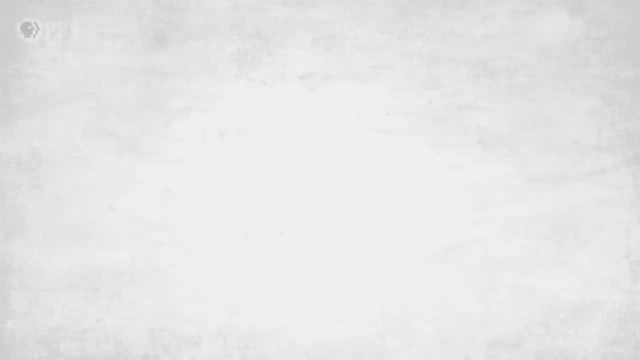 is the average temperature. Whitaker's graph works because terrestrial biomes are mainly defined by their temperature and precipitation patterns. However, this doesn't tell us much about the wide variety of aquatic ecosystems that exist in oceans, rivers, lakes, swamps, coral reefs. 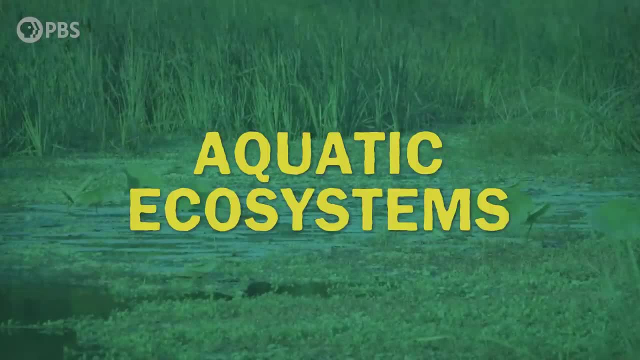 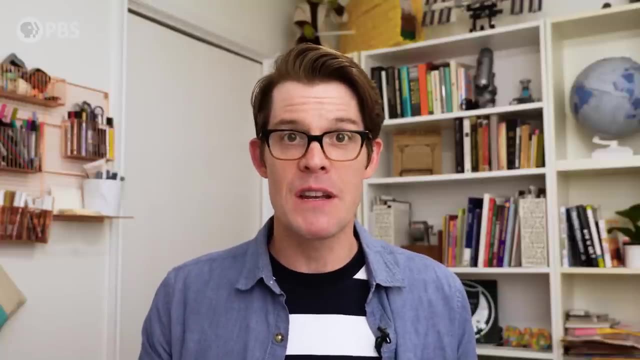 rivers, lakes, swamps, coral reefs and marshes. Aquatic ecosystems are defined by things like salinity, water flow and depth. Now, this all kind of feels like a bunch of definitions, and it kind of is, but they are important to understand because everything from prehistoric to modern life, as 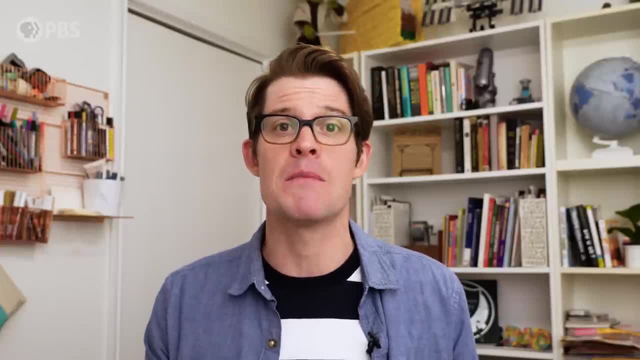 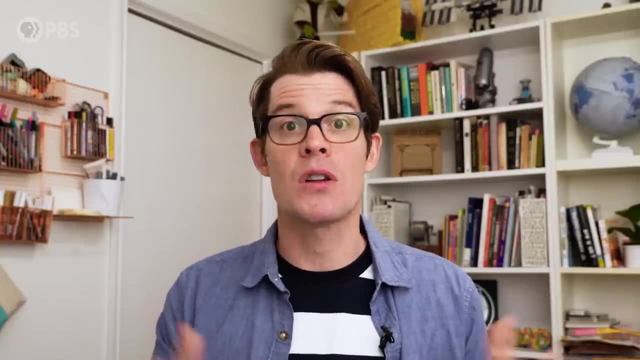 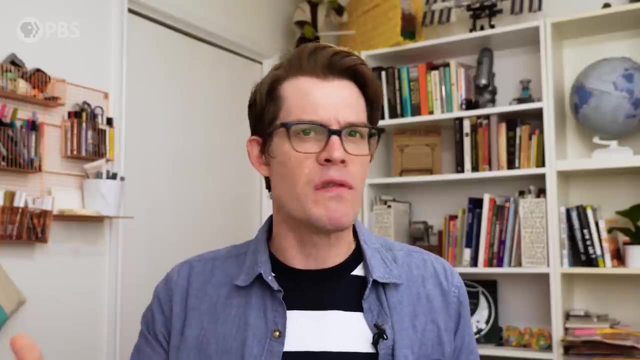 we know it was constructed in and around these natural systems. We humans benefit immensely from all aspects of the natural world. We depend on Earth's systems for clean air to breathe, clean water to drink and fertile soil in which to grow crops. We also place aesthetic and cultural 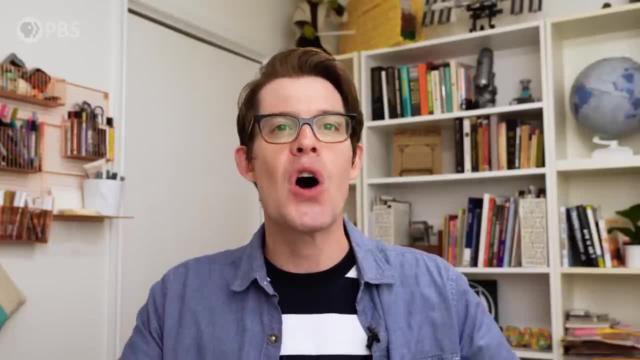 value onto our natural resources through poetry, literature and literature. We also place aesthetic and cultural value onto our natural resources through poetry, literature and literature. We also place aesthetic and cultural value onto our natural resources through poetry, literature, songs and paintings dedicated to and inspired by nature. 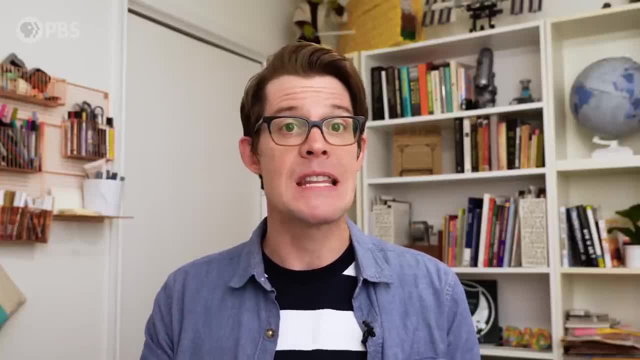 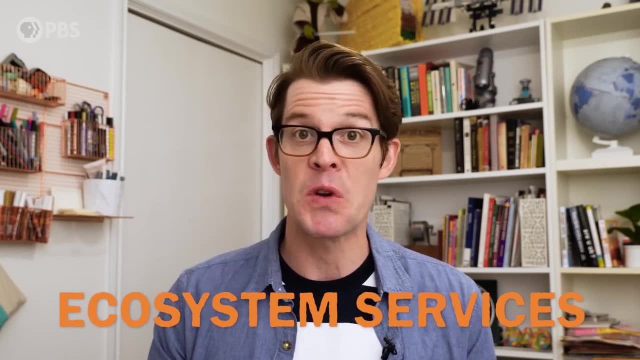 Altogether. this practically endless list of benefits that the natural world provides are called ecosystem services. Here's an example to get your head around ecosystem services. The oceans are full of fish, which is a huge benefit for millions of people around the world. 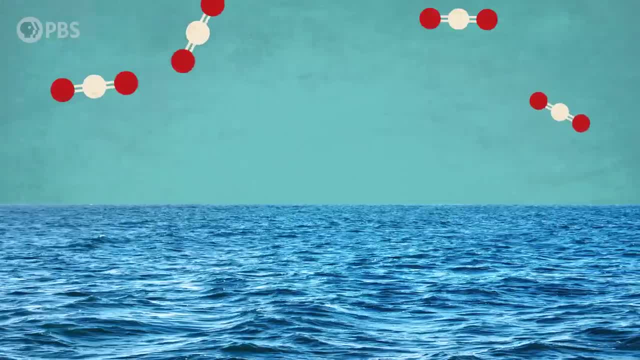 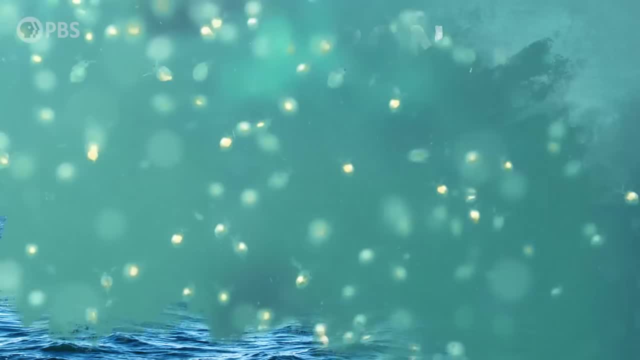 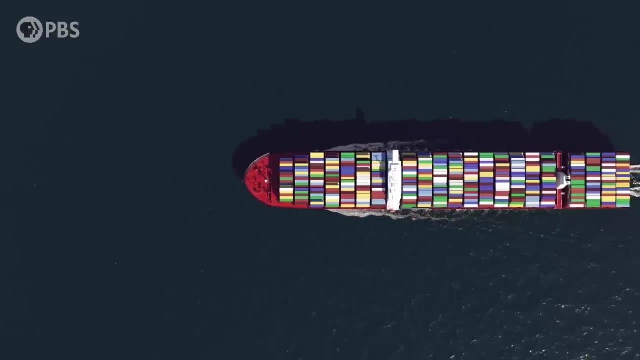 But that isn't the only service that the ocean provides. It absorbs a lot of carbon dioxide from the atmosphere too, helping to regulate the entire planet's climate, And a huge portion of the oxygen that we breathe comes from photosynthetic marine plankton. The ocean also serves as a highway system for transporting goods from 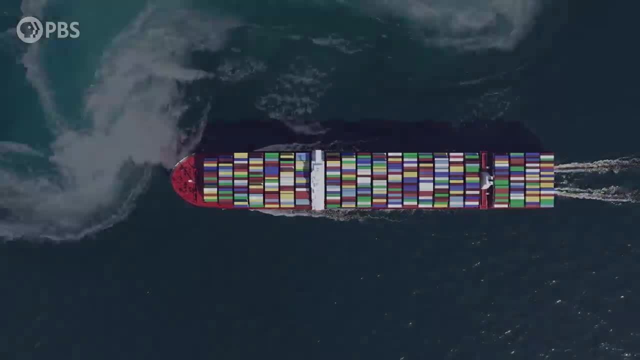 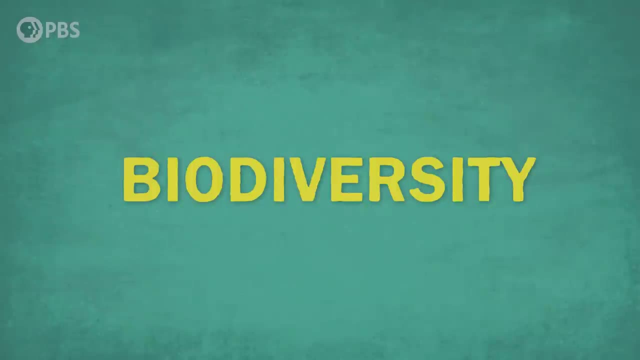 country to country on cargo ships. We even harness the energy of waves and tides to generate electricity. Biodiversity in all its forms is an area that especially demands protection. There are three main types of biodiversity: One: genetic diversity within a population. Two: species richness, species diversity. 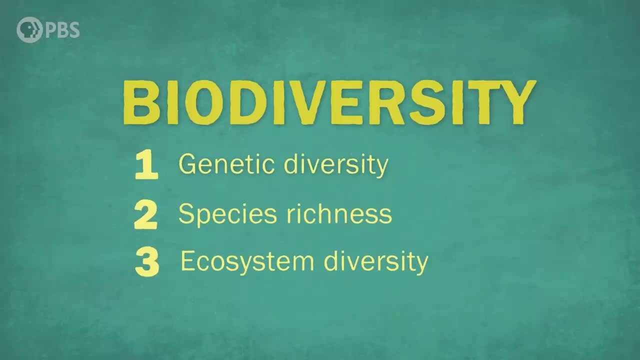 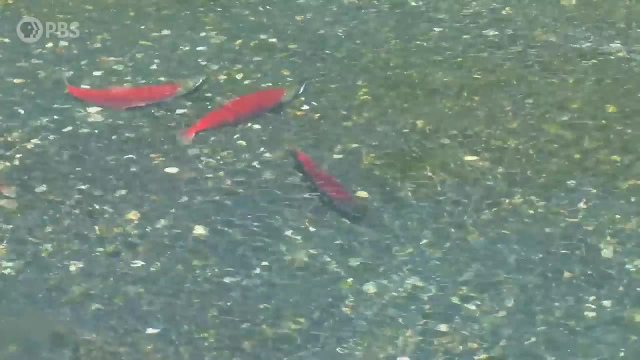 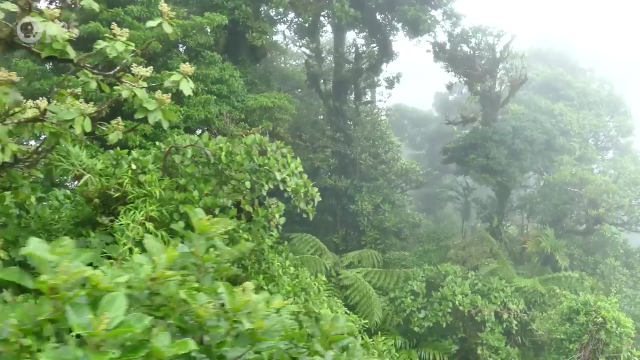 Three ecosystem diversity within an ecosystem And three ecosystem diversity in an area. A population with large genetic diversity has greater potential to adapt to environmental changes, whereas high species richness makes an ecosystem more stable and better able to recover from disturbances. And finally, an area with a rich diversity of habitats and ecosystems. 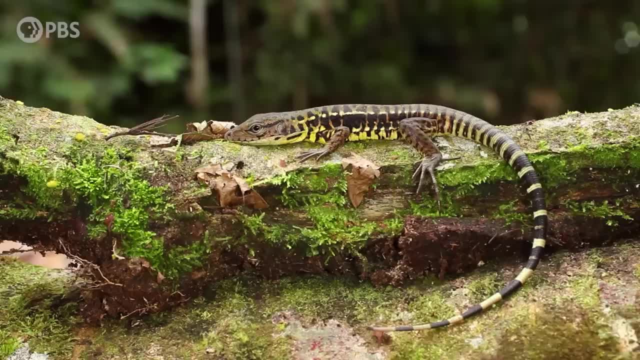 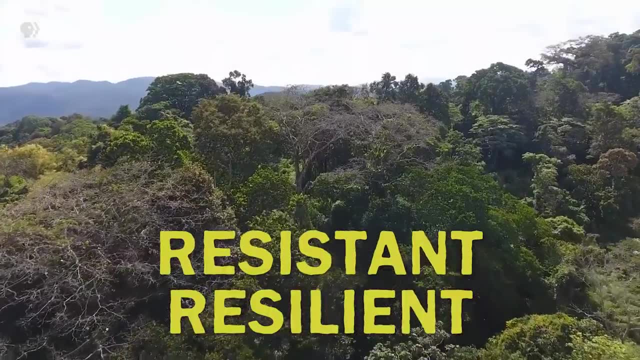 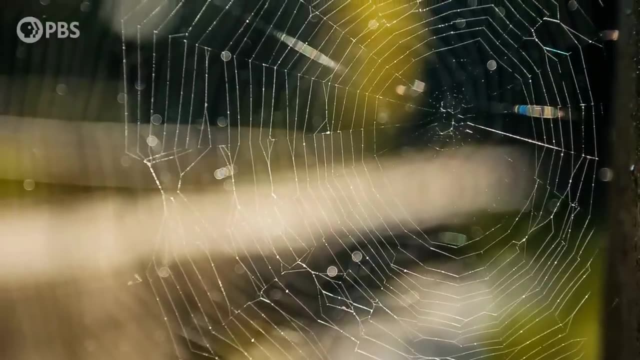 can support a more robust and stable community of organisms. So biodiversity overall helps an ecosystem be more resistant and resilient in the face of environmental changes, whether they're natural hazards or human impacts. An ecosystem with high biodiversity is like a giant, well-spun spider's web. 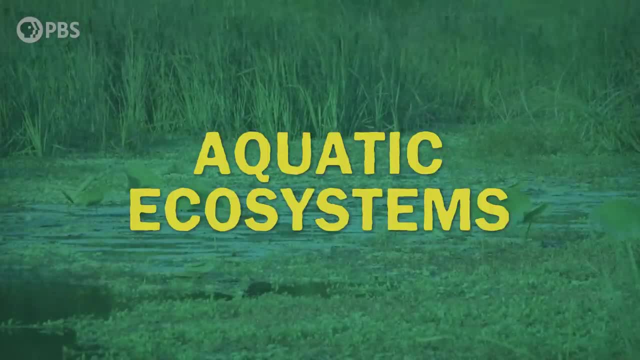 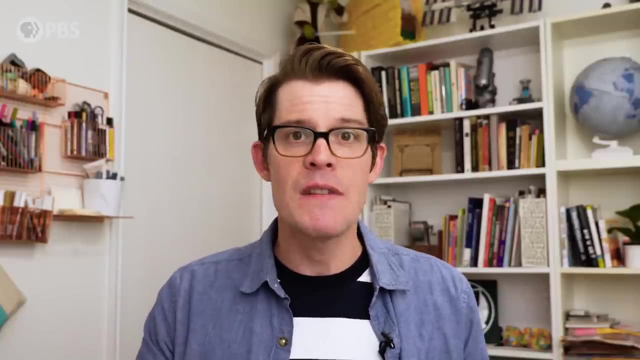 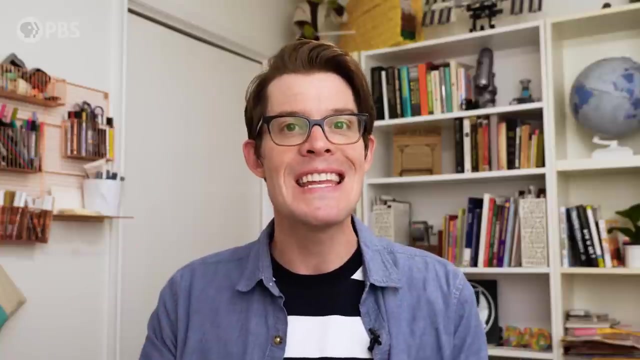 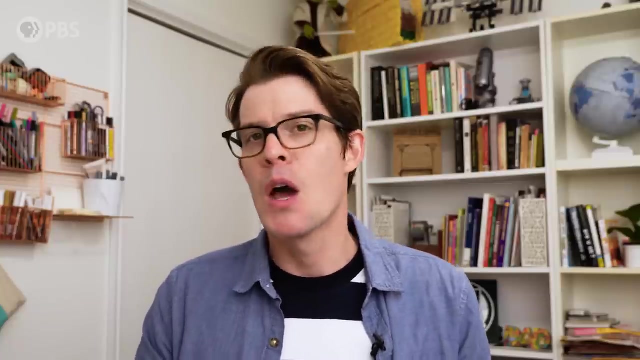 and marshes. Aquatic ecosystems are defined by things like salinity, water flow and depth. This all feels like a bunch of definitions and it kind of is, but they are important to understand. We humans benefit immensely from all aspects of the natural world. We depend on Earth's systems for 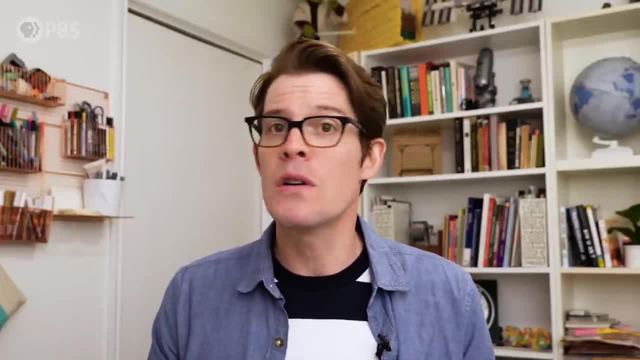 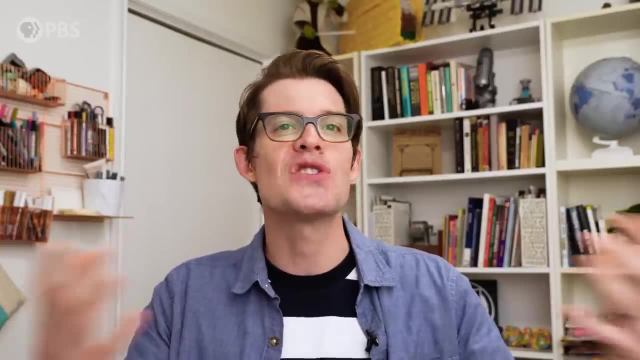 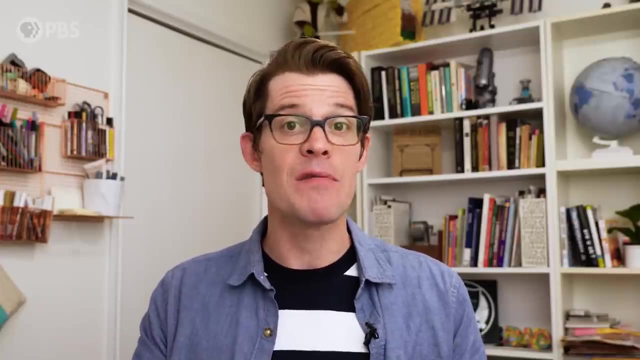 clean air to breathe, clean water to drink and fertile soil in which to grow crops. We also place aesthetic and cultural value onto our natural resources through poetry, songs and paintings dedicated to and inspired by nature. Altogether, this practically creates an endless list of benefits that the natural world provides, called ecosystem services. 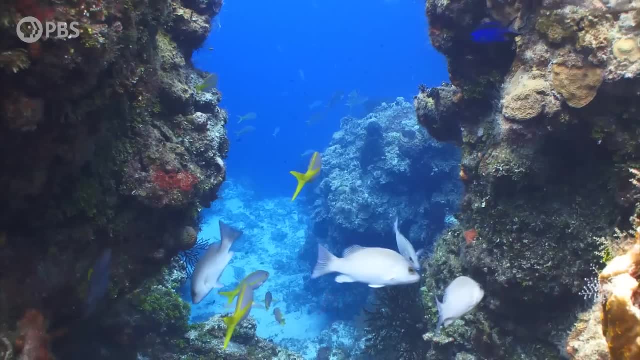 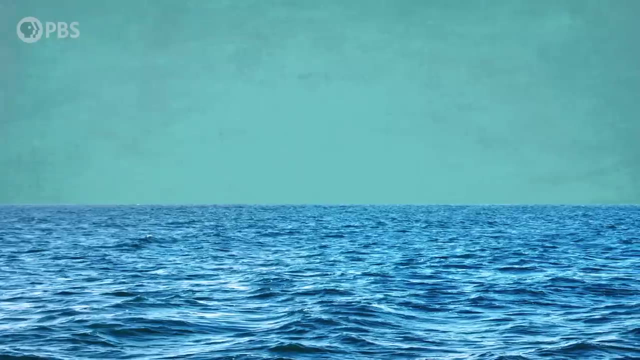 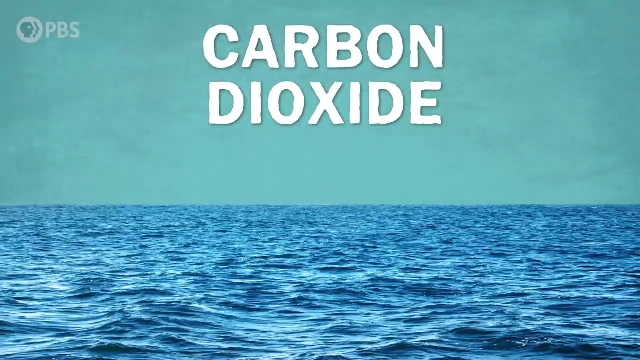 Here's an example to get your head around: ecosystem services. The oceans are full of fish, which is a huge benefit for millions of people around the world, But that isn't the only service the ocean provides. It absorbs a lot of carbon dioxide from the atmosphere, helping to regulate the entire planet's climate And a huge portion of 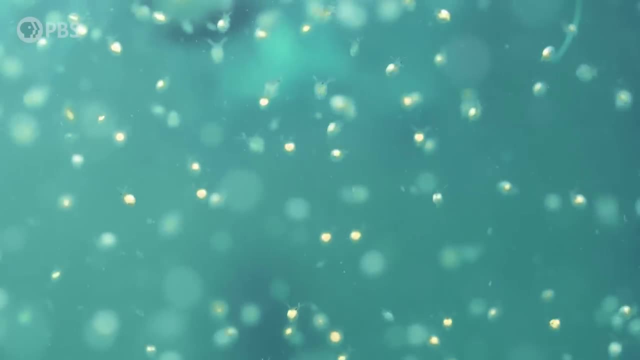 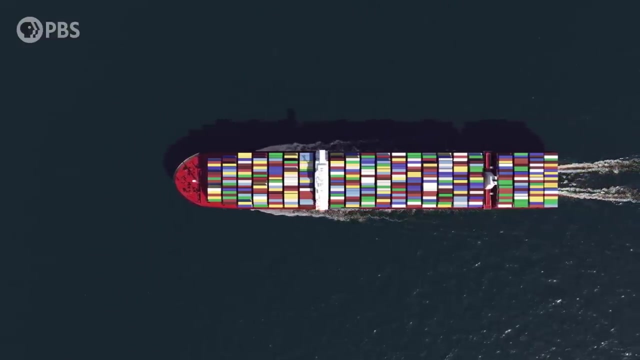 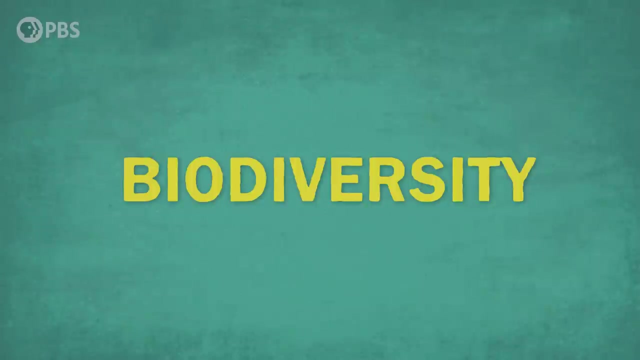 the oxygen that we breathe comes from photosynthetic marine plankton. The ocean also serves as a highway system for transporting goods from country to country on cargo ships, and we even harness the energy of waves and tides to generate electricity. Biodiversity in all its forms is an area that especially demands protection. 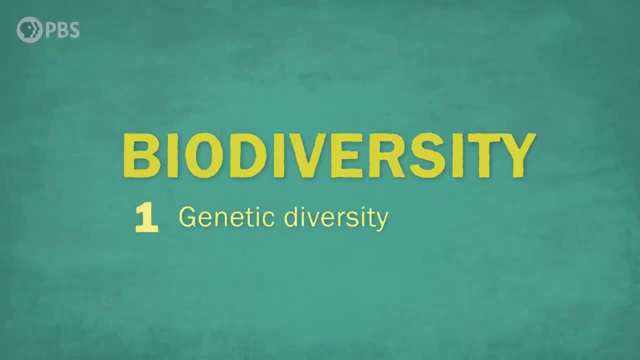 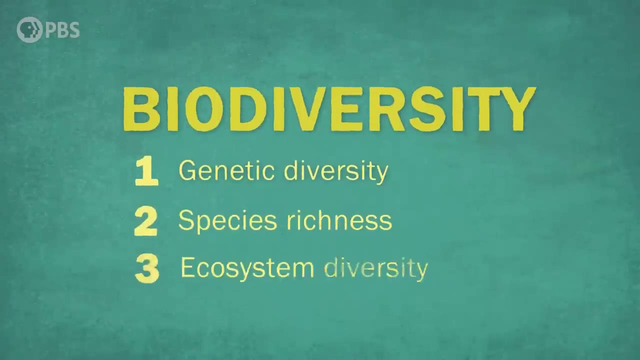 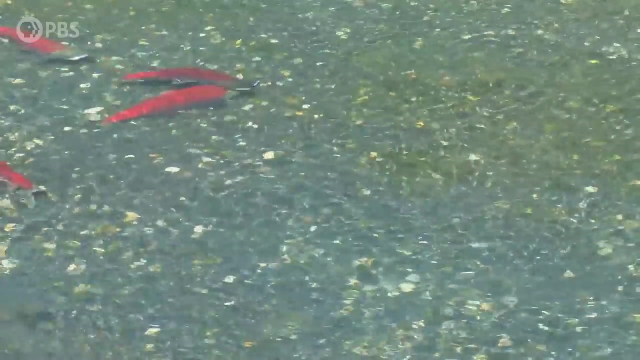 There are three main types of biodiversity: One, genetic diversity within a population, Two, species richness, species diversity within an ecosystem. And three, ecosystem diversity in an area. A population with large genetic diversity has greater potential to adapt to environmental changes. 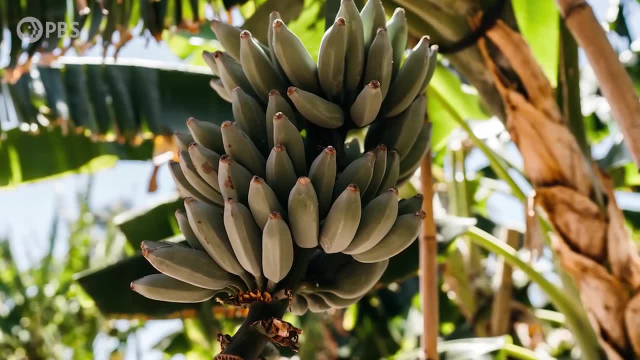 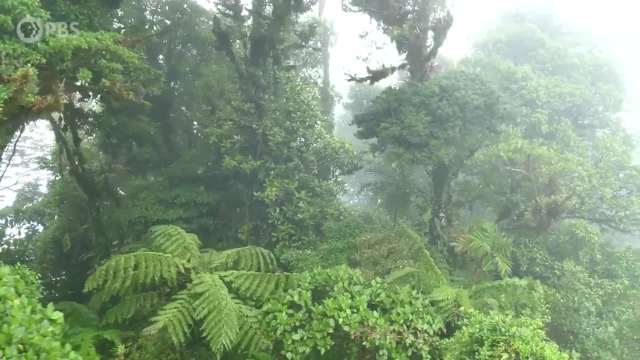 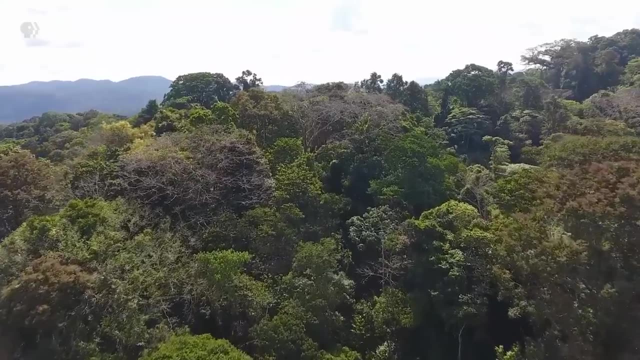 whereas high species richness makes an ecosystem more stable and better able to recover from disturbances. And finally, an area with a rich diversity of habitats and ecosystems can support a more robust and stable community of organisms. So biodiversity overall helps an ecosystem be more resistant and resilient in the face. 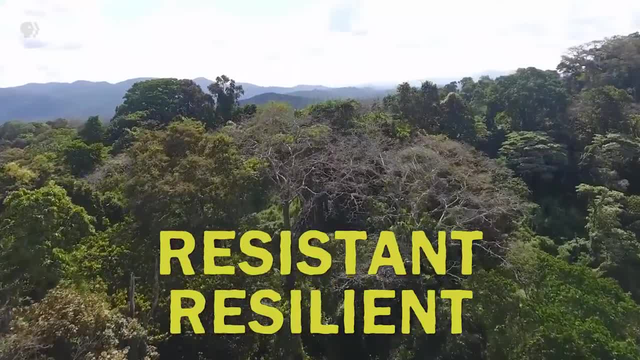 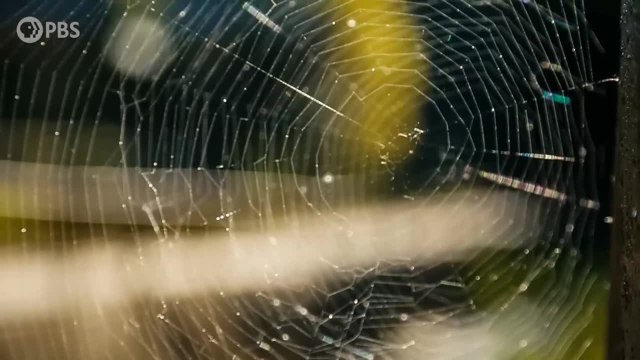 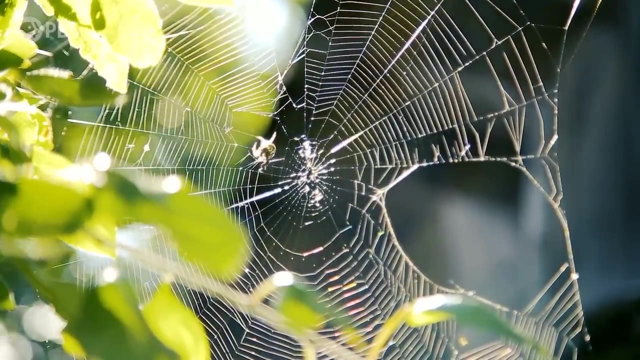 of environmental changes, whether they're natural hazards or human impacts. An ecosystem with high biodiversity is like a giant, well-spun spider's web: Lots and lots of interconnected points. If the web has a little rip in one area, it can probably still function because it's supported and held together by hundreds of other. 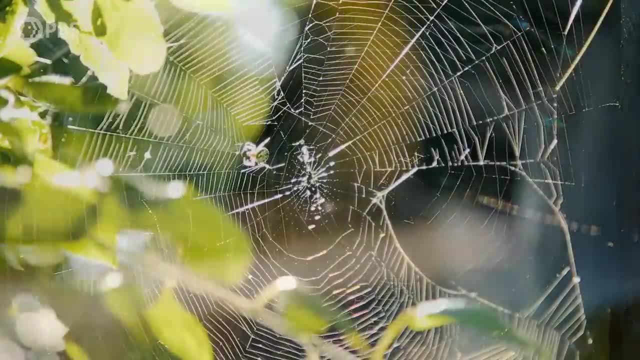 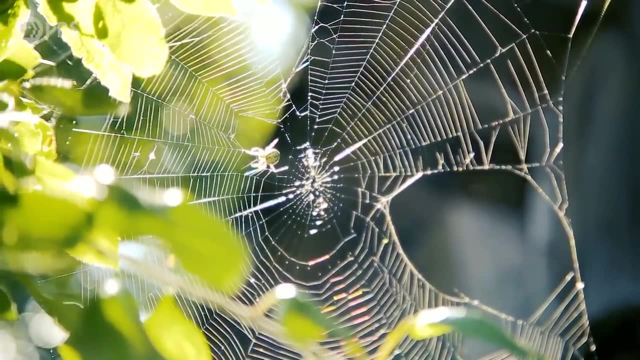 Lots and lots of interconnected points. If the web has a little rip in one area, it can probably still function because it's supported and held together by hundreds of other strands that are woven together. But if the web is only made of two or three strands, 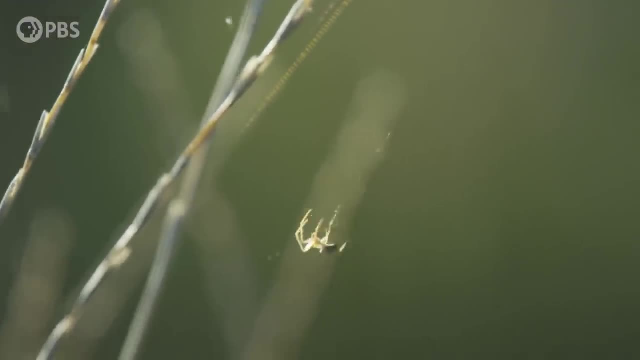 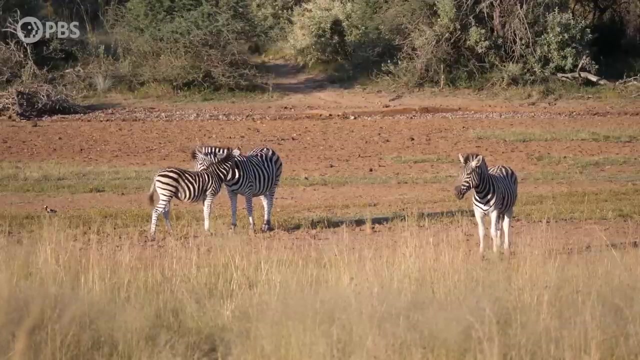 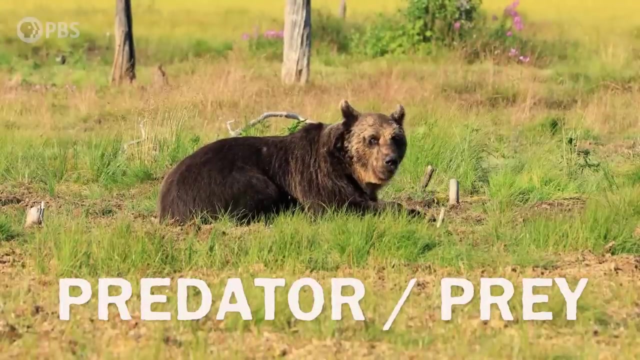 then the same small rip could collapse the entire web And within that ecosystem web. species constantly interact with each other and those relationships have shaped those species' evolution. And some of the most important evolutionary relationships are predator-prey relationships- Who's eating who? Food webs and trophic pyramids are both. 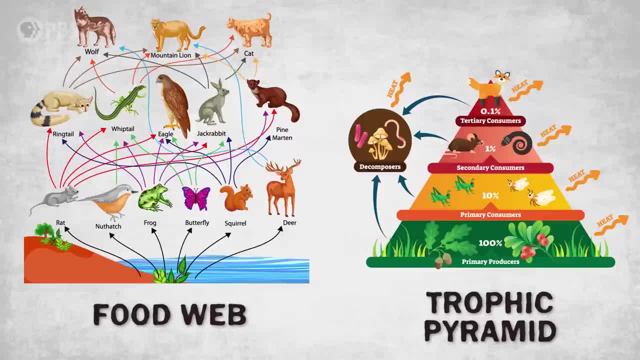 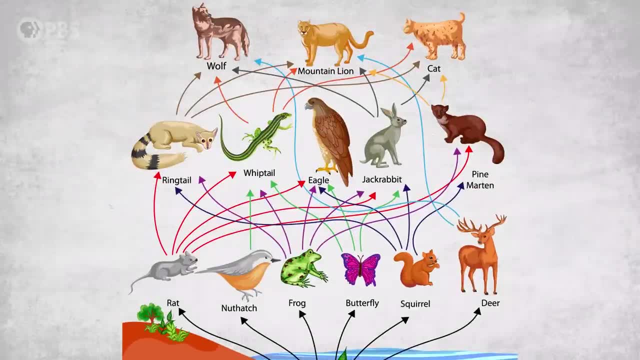 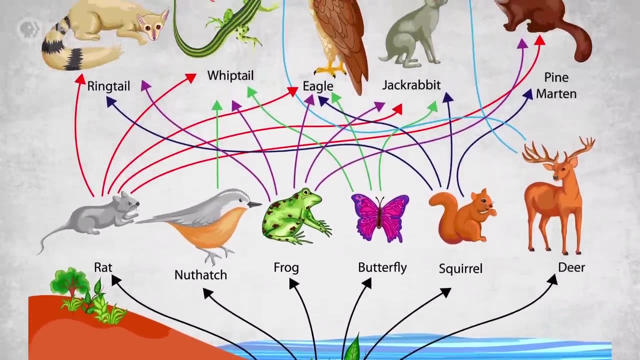 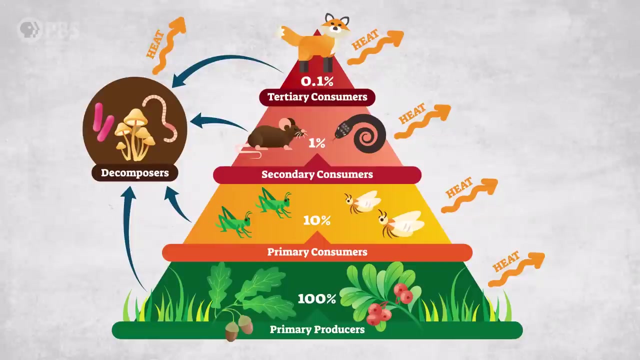 scientific models which represent how predators and their prey interact within an ecosystem, But they emphasize different things. The arrows in a food web map the flow of energy and nutrients within the system, which in general goes from plants to primary consumers to secondary consumers. On the other hand, the pyramid helps to quantify how energy moves between 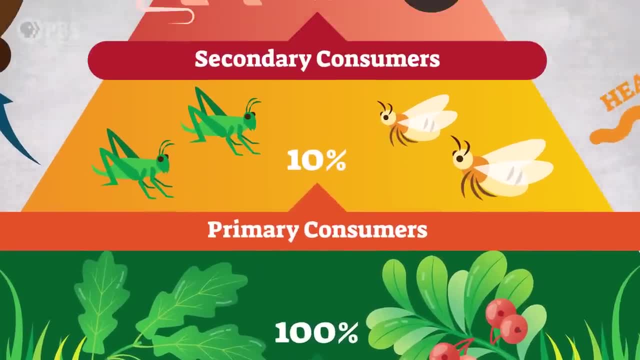 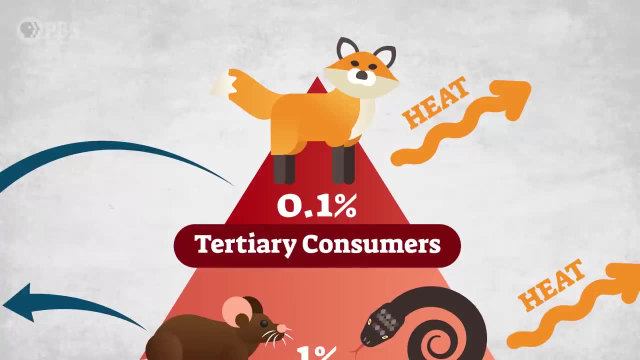 the different trophic levels, from producers all the way up to apex predators, And it emphasizes why there are proportionally fewer species as you move up the pyramid, In other words, why there's always more mice than eagles and why it takes so much grass to make a cow. 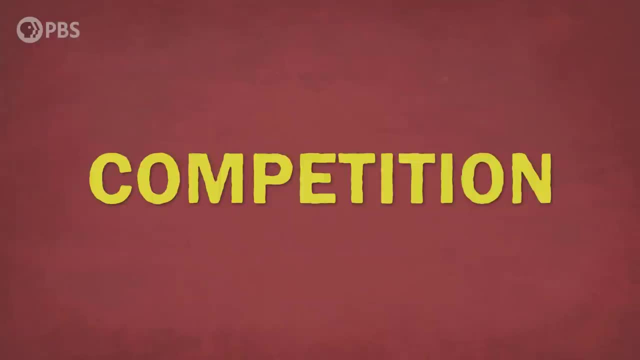 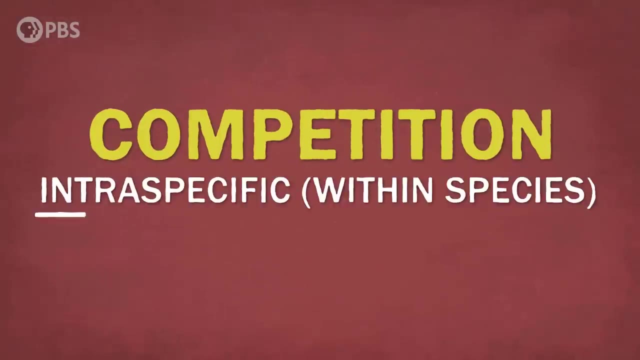 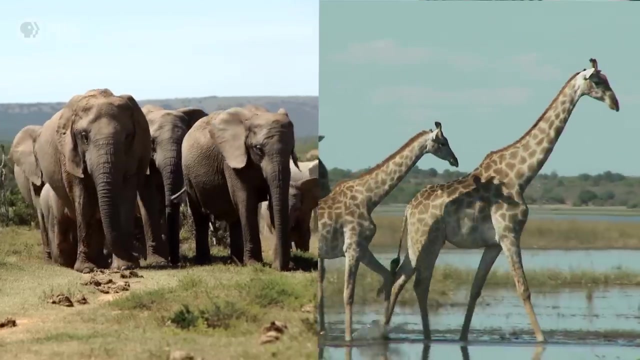 Another important ecosystem relationship is competition. Limited resources like food or nesting sites can cause competition, And this can be within species, intraspecific competition or between different species interspecific competition. Elephants and giraffes may experience interspecific competition for water in an arid climate, whereas two trees of the same 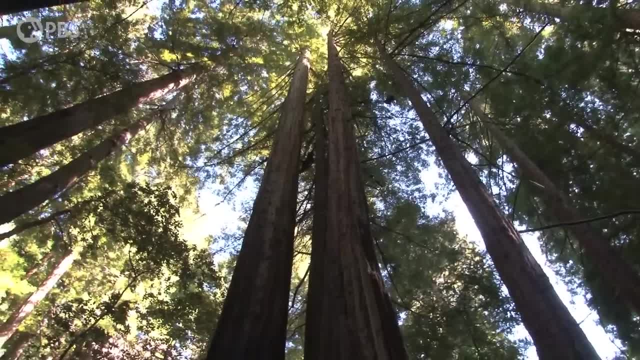 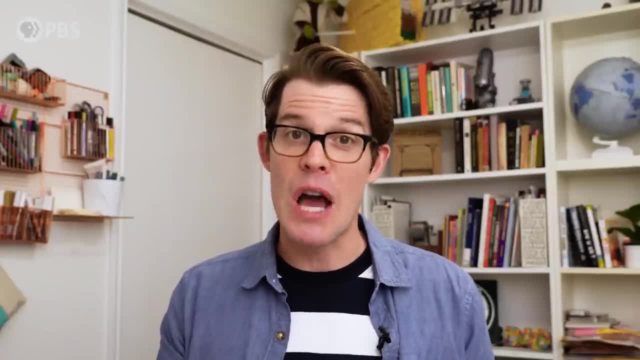 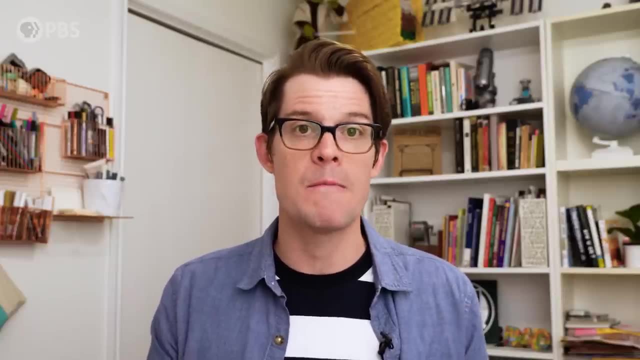 species can experience intraspecific competition for the sunlight that's needed for photosynthesis. These competitive pressures for limited resources are really strong driving forces for natural selection, and individuals with the adaptations to get more resource tend to survive better. A final major way in which different species interact is 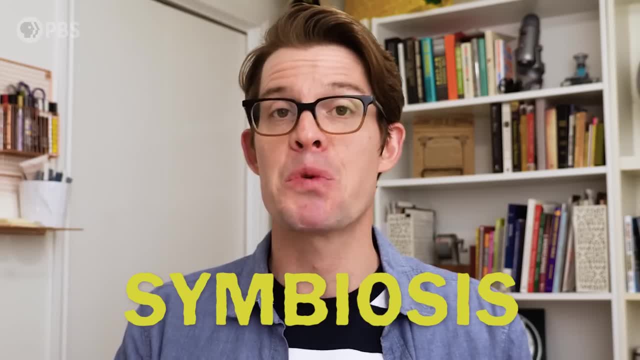 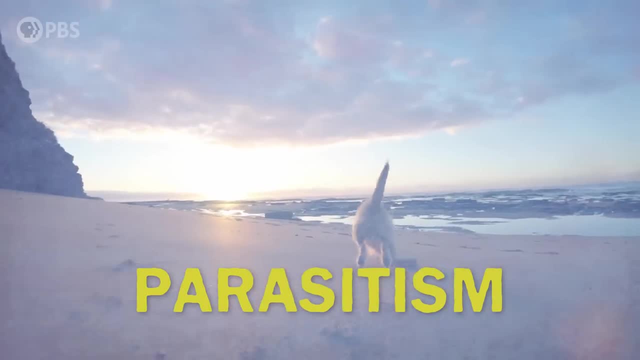 symbiosis. Generally, symbiosis is broken into three categories. one: communicated paracytism, in which one species benefits and the other is harmed, like a tapeworm in a dog's intestine. Two: mutualism: In a mutualistic relationship, both species benefit and this transfer is in reality an inconvenient form of family Yo. 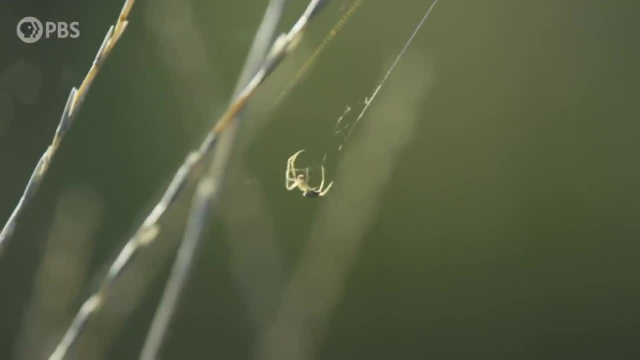 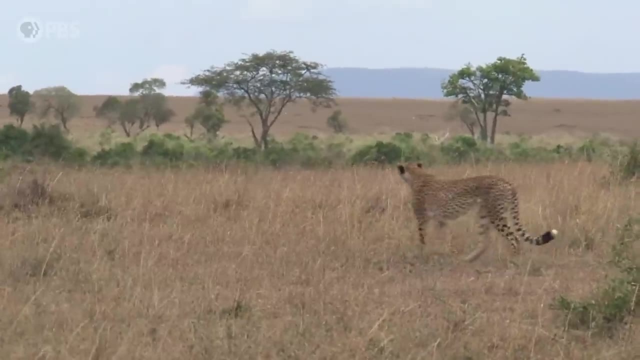 strands that are woven together, But if the web is only made of two or three strands, then the same small rip could collapse the entire web. Within that ecosystem web, species constantly interact with each other and those relationships have shaped those species' lives. So if you're interested in learning more about biodiversity, 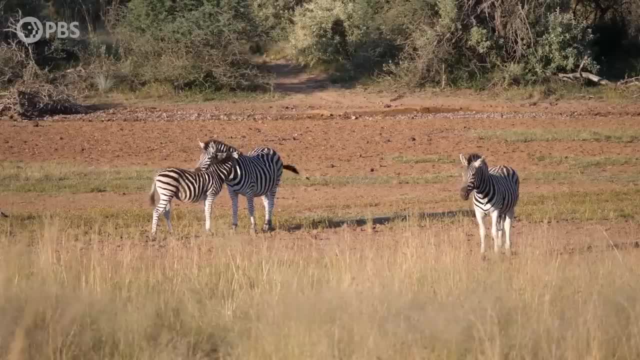 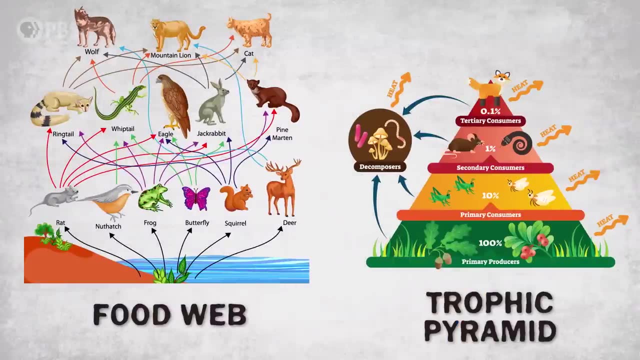 you'll want to check out my video on how to make your own species. evolution And some of the most important evolutionary relationships are predator-prey relationships: Who's eating who? Food webs and trophic pyramids are both scientific models which represent how predators 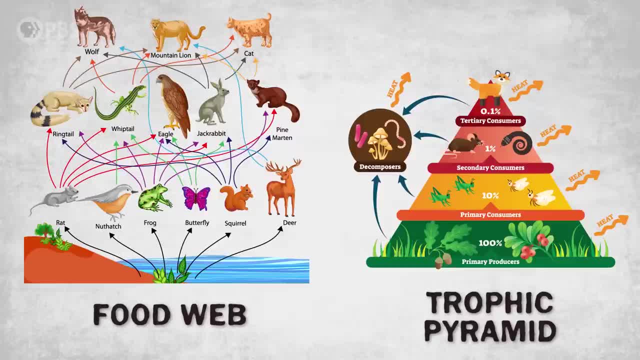 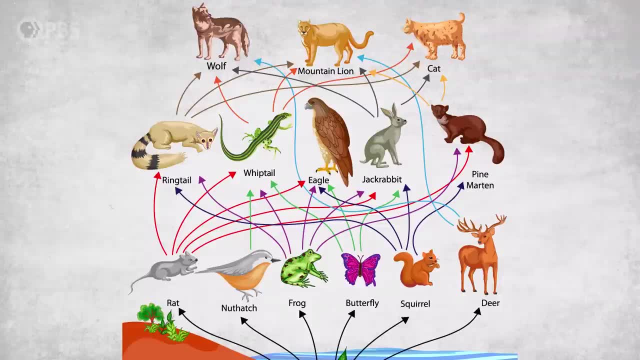 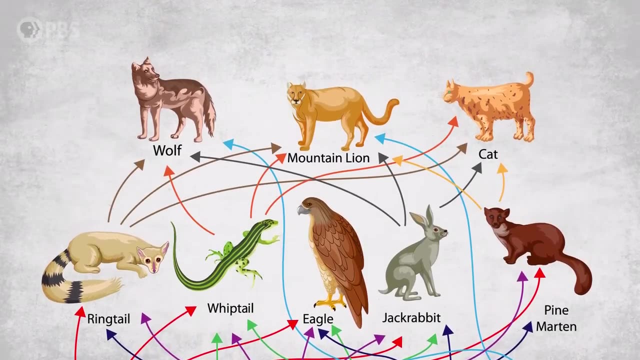 and their prey interact within an ecosystem, But they emphasize different things. The arrows in a food web map the flow of energy and nutrients within the system, which in general goes from plants to primary consumers to secondary consumers. On the other hand, the pyramid helps to quantify how energy moves between 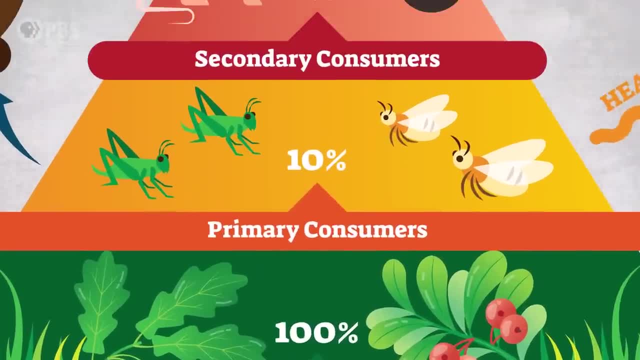 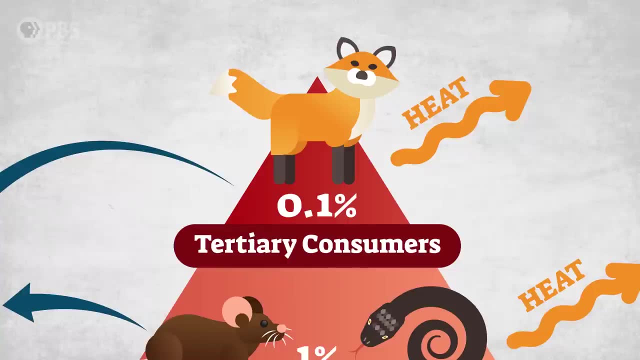 the different trophic levels, from producers all the way up to apex predators, And it emphasizes why there are proportionally fewer species as you move up the pyramid, In other words, why there's always more mice than eagles and why it takes so much grass to make a cow. 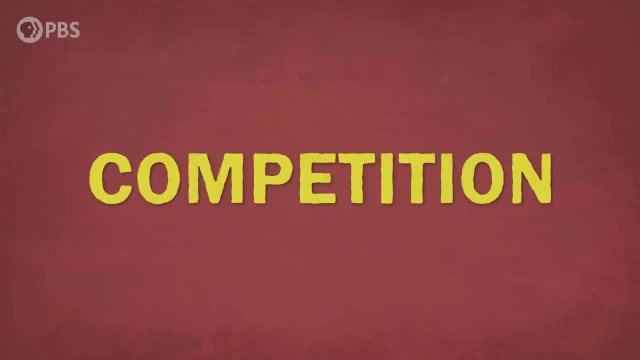 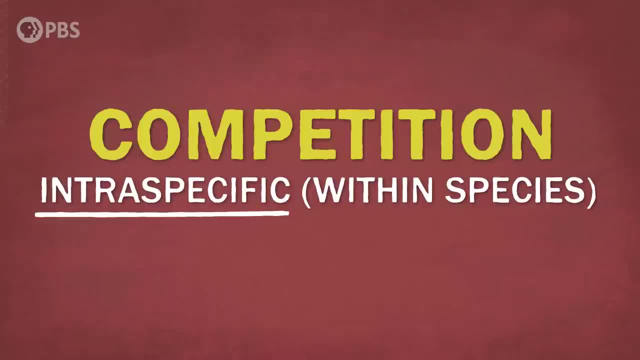 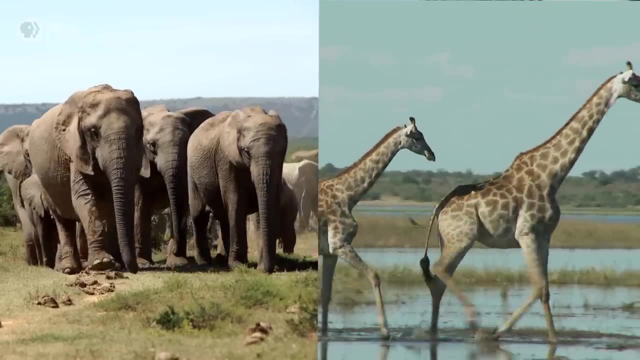 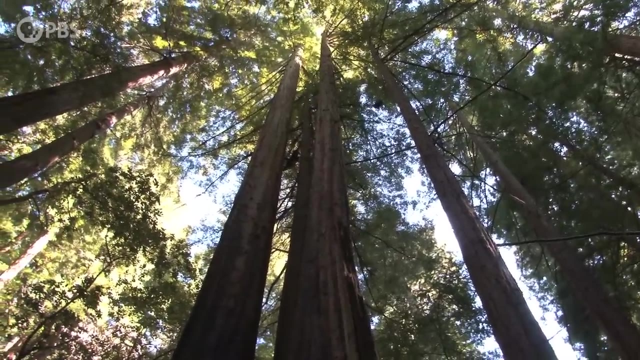 and this can be within species, intraspecific competition or between different species interspecific competition. Elephants and giraffes may experience interspecific competition for water in an arid climate, whereas two trees of the same species can experience intraspecific competition. 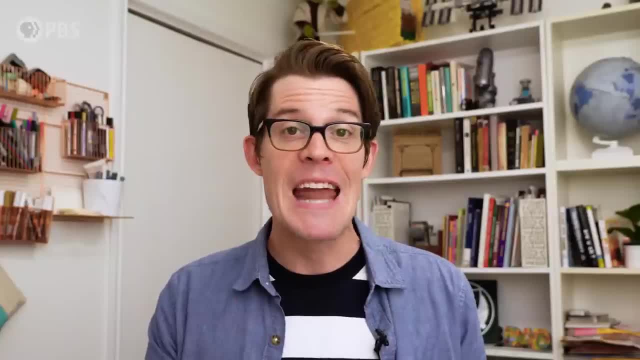 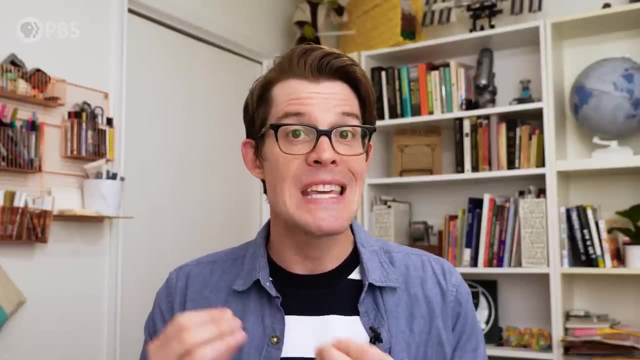 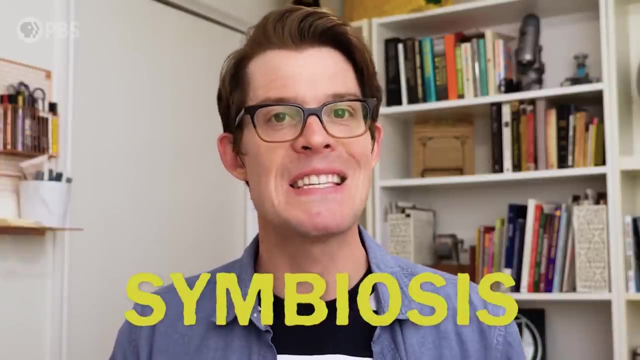 for the sunlight that's needed for photosynthesis. These competitive pressures for limited resources are really strong driving forces for natural selection, and individuals with the adaptations to get more resources tend to survive better. A final major way in which different species interact is symbiosis Generally, 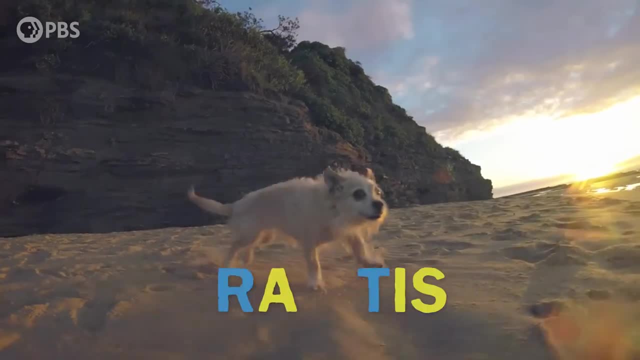 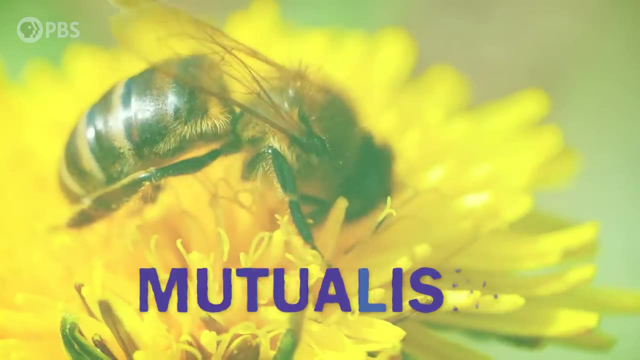 symbiosis is broken into three categories. One: parasitism, in which one species benefits and the other is harmed, like a tapeworm in a dog's intestine. Two: mutualism: in a mutualistic relationship, both species benefit, like bees pollinating flowers. 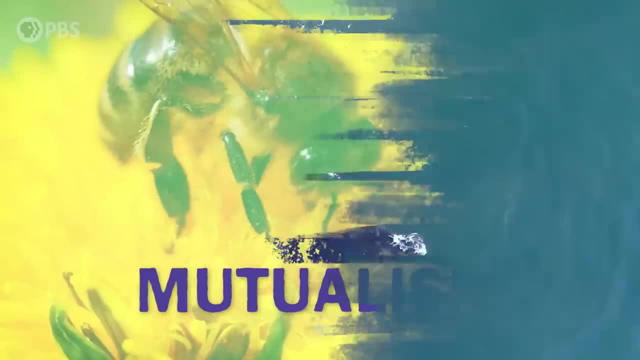 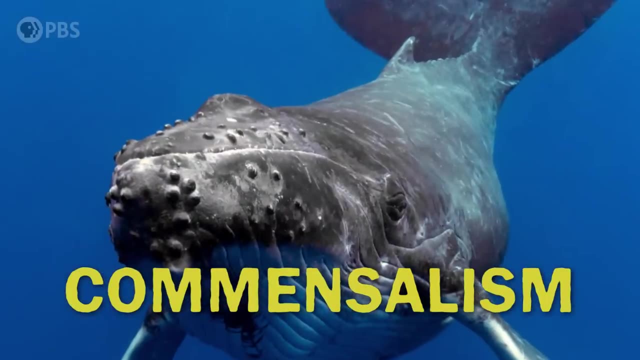 It does the opposite. phenomenal thing: How stays rooming a creature is umpteen natural values- Our benefit, like bees pollinating flowers. and three commensalism, where one species benefits and the other isn't really necessarily affected. Whales don't really care about the barnacles on their skin, but the barnacles rely on the. 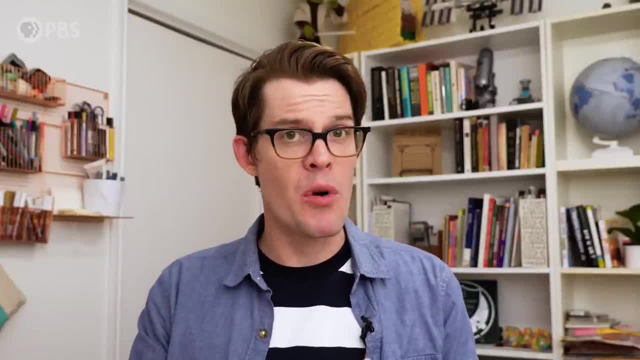 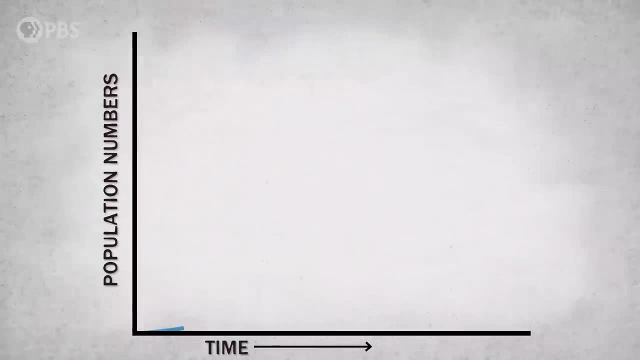 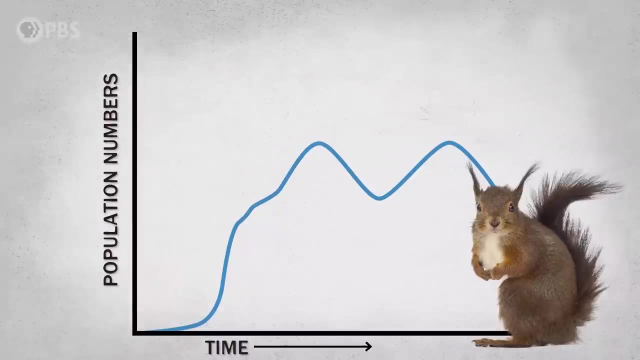 whales for a lot. All these types of interactions—predator-prey, competition, symbiosis—influence how a population grows. Here's a model representing the growth of a population of squirrels in a city park. If we look at how that population changes over time, we see that it experiences lots. 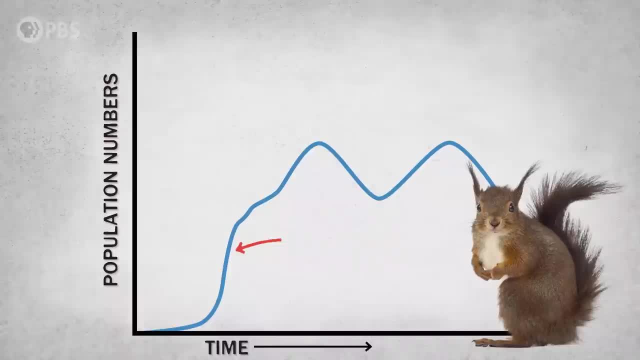 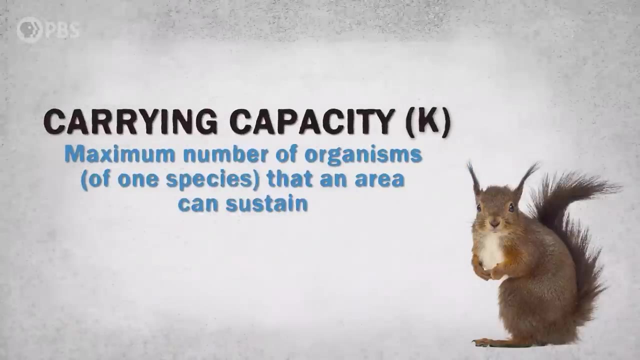 of growth early on, when a pair of squirrels first discover this amazing new park. Then eventually the population reaches its carrying capacity. Carrying capacity, which is normally written as an uppercase K, is the maximum number of organisms of one species that an area can sustain. 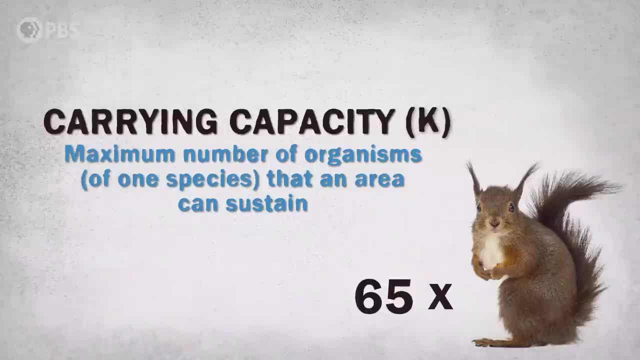 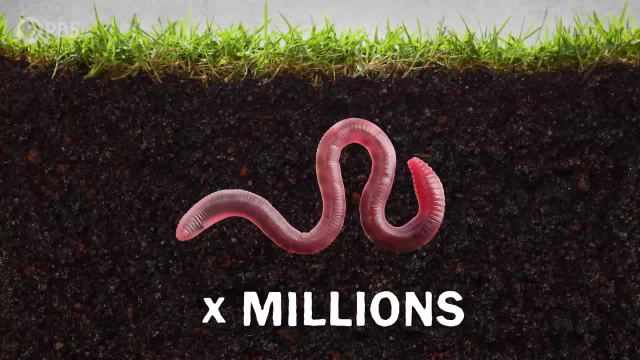 In our city park. here the carrying capacity is about 65 squirrels, But if we head underground the carrying capacity for earthworms is probably in the millions. Food space and the threat of predation help to define a population's carrying capacity. 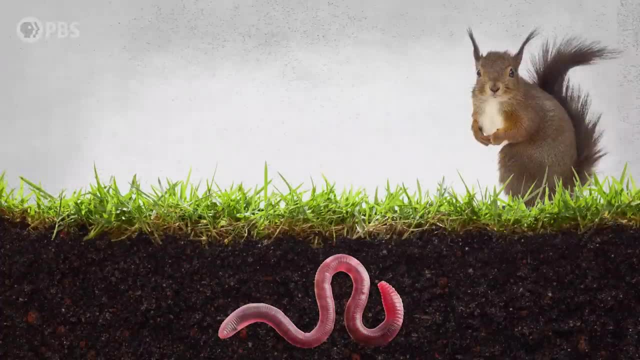 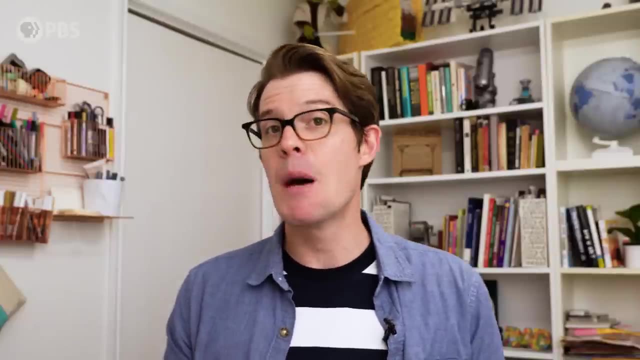 Because squirrels and earthworms require totally different resources. that's why they have such different carrying capacities. On the flip side from population growth or upper limits, when the numbers of a particular species are low enough that it might become extinct, we consider that species endangered. 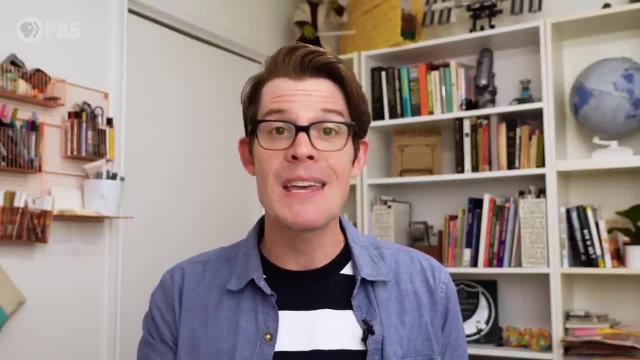 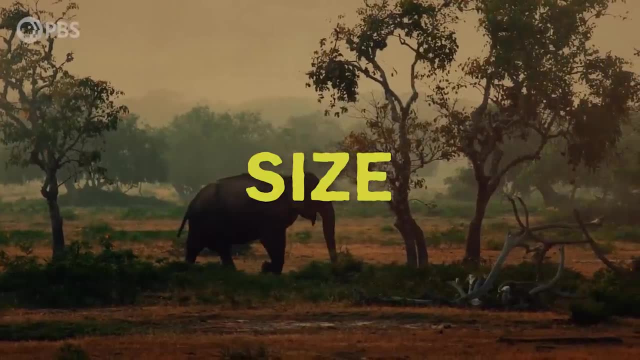 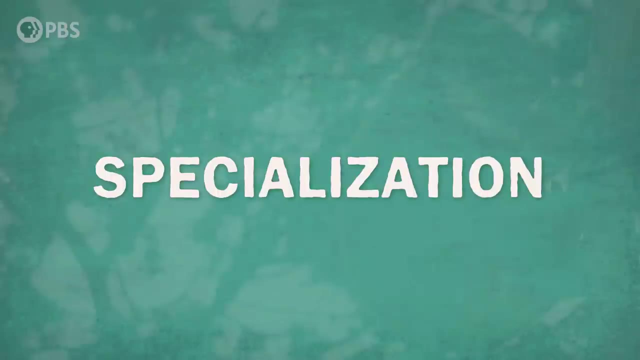 Some qualities make certain species more at risk than others of becoming endangered or extinct: Like size, large organisms with big home ranges and habitat needs, like say elephants or grizzly bears, are at greater risk. Or specialization- super specialized organisms with specific dietary needs or habitat requirements. 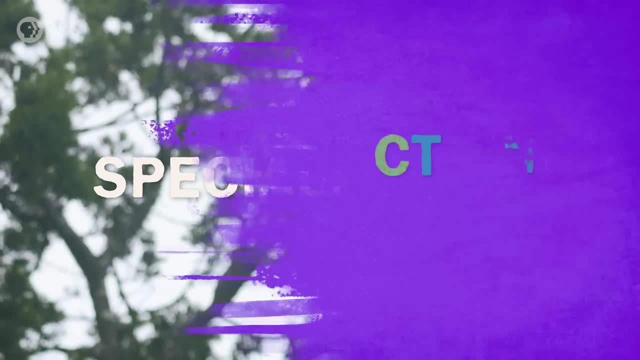 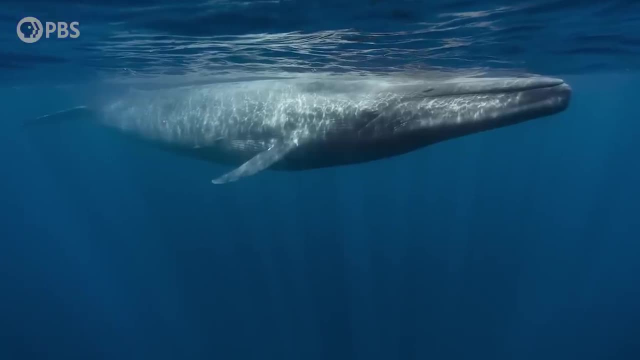 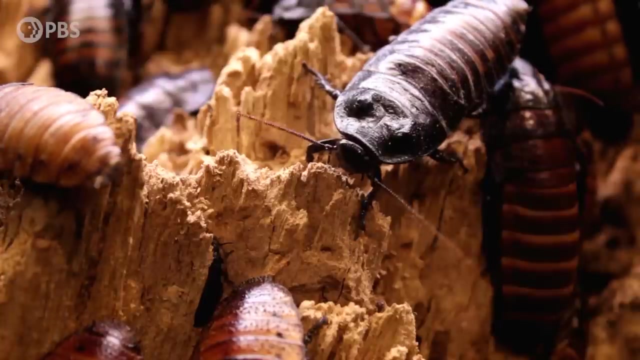 like maybe pandas or koalas, are also at greater risk And reproduction rates organisms who reproduce slowly and require many years of parental care, like blue whales or a mountain gorilla, are also at greater risk, And those species with something like a cockroach, which reproduces early and prolifically. and 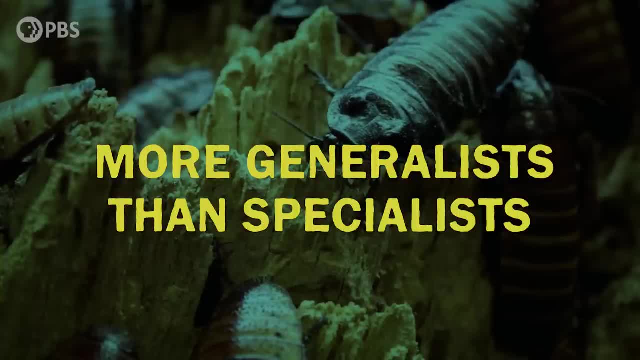 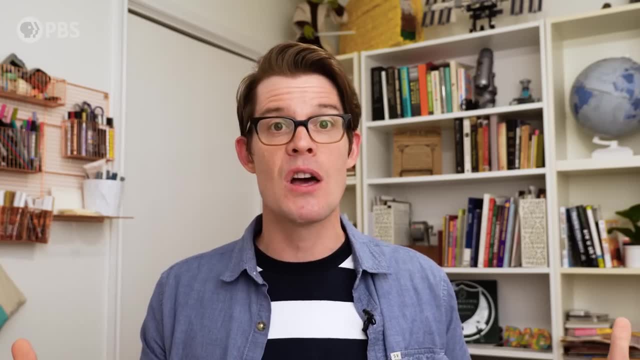 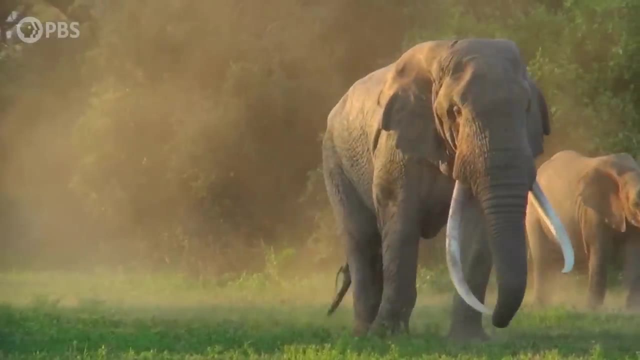 are more generalists than specialists when it comes to diet and habitat. Being able to quickly reproduce is an evolutionary advantage that maximizes the chance that a random genetic mutation will help an individual survive a disturbance. An African elephant, with its much slower reproduction rate and very specialized habitat, does not. 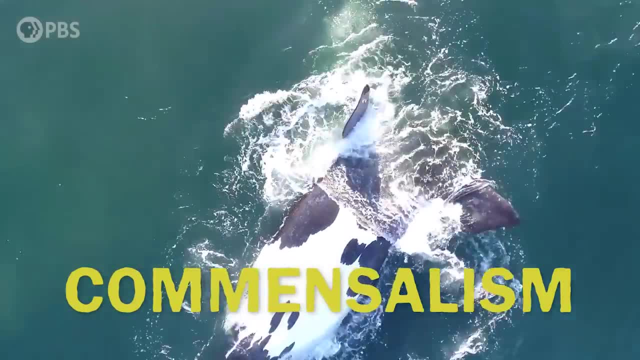 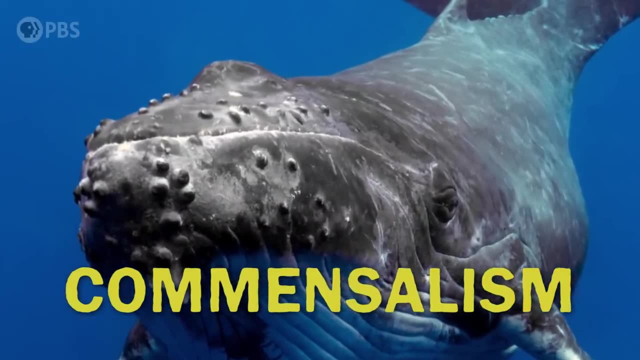 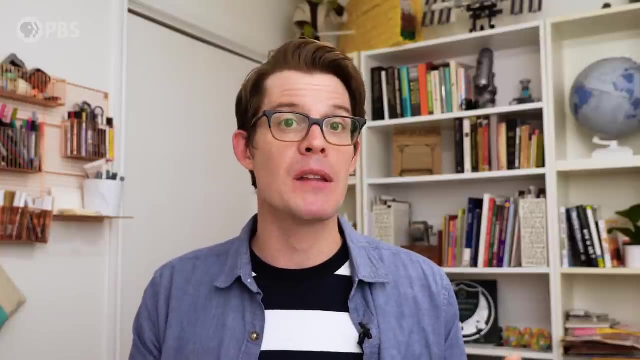 Three: commensalism, where one species benefits and the other isn't really affected. Whales don't really care about the barnacles on their skin, but the barnacles rely on the whales for a lot. All these types of interactions—predator-prey, competition, symbiosis—influence how a population 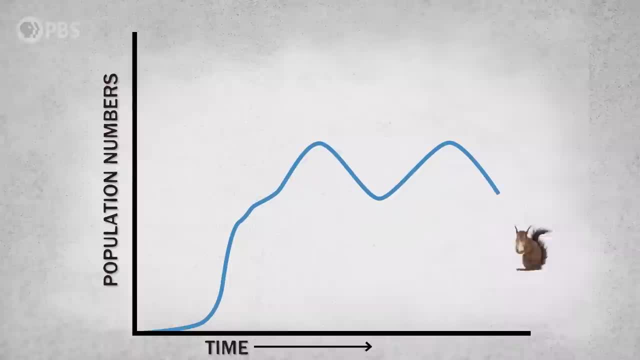 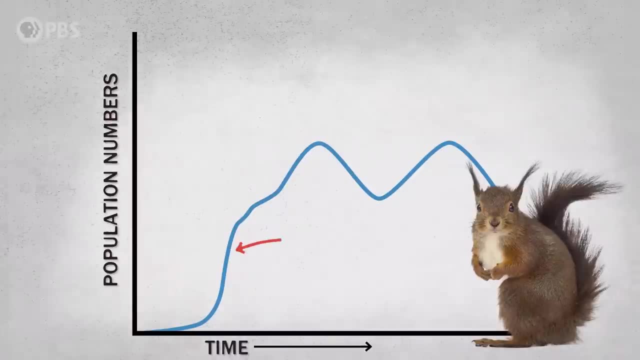 grows. Here's a model representing the growth of a population of squirrels in a city park. If we look at how that population changes over time, we see that it experiences lots of growth early on, when a pair of squirrels first discover this amazing new park. 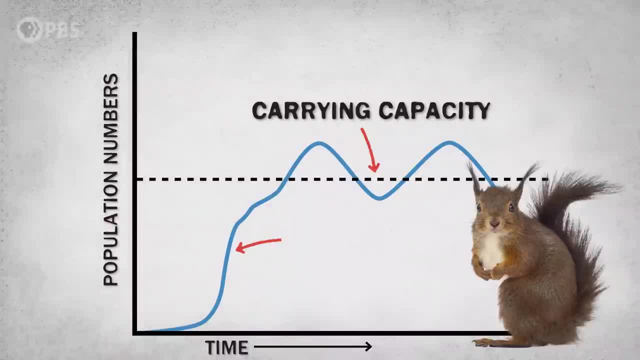 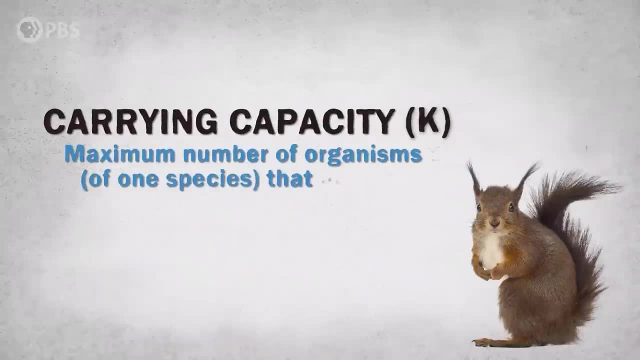 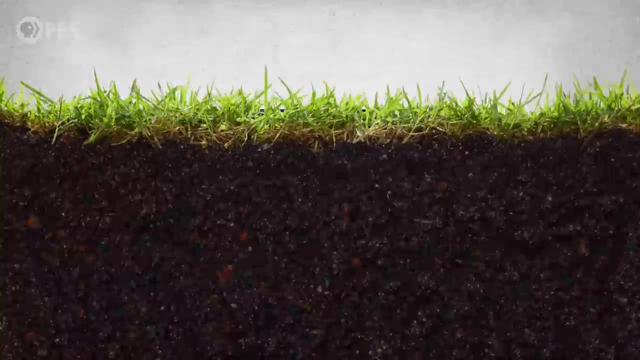 but then eventually the population changes. The population reaches its carrying capacity. Carrying capacity, which is normally written as an uppercase K, is the maximum number of organisms of one species that an area can sustain. In our city park here the carrying capacity is about 65 squirrels, but if we head underground, 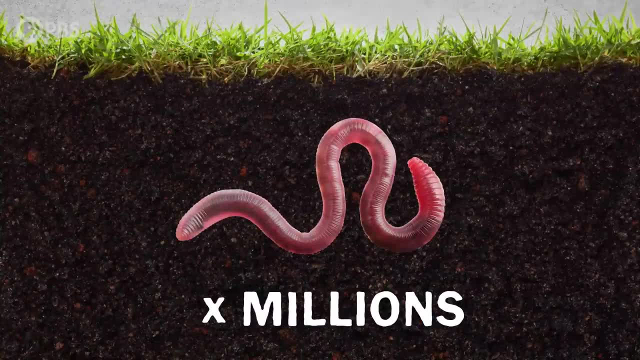 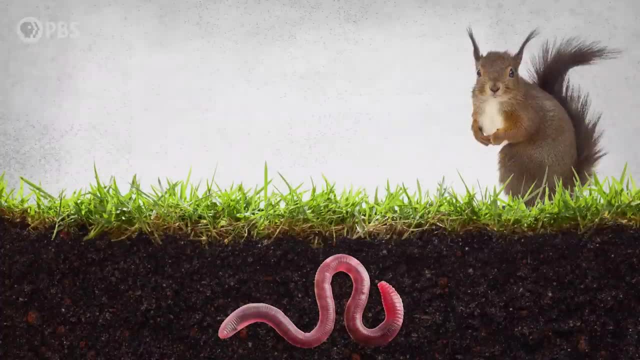 the carrying capacity for earthworms is probably in the millions. Food space and the threat of predation help to define a population's carrying capacity, Because squirrels and earthworms require totally different resources. that's why they have such different carrying capacities. 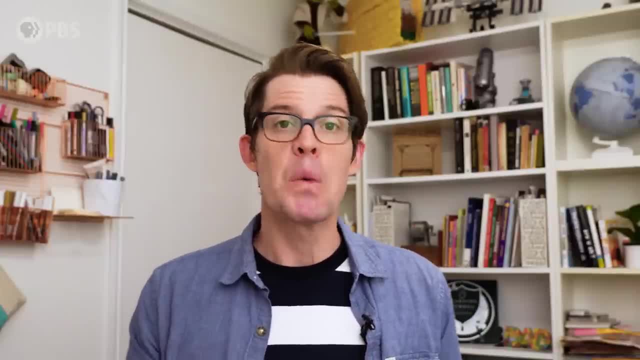 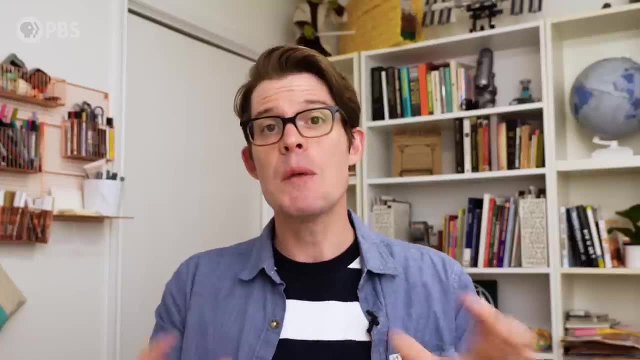 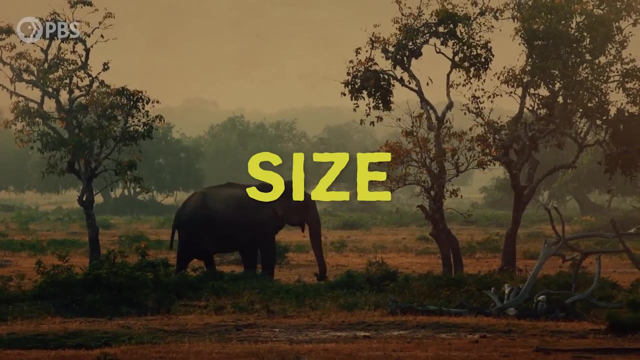 On the flip side from population growth or upper limits. when the numbers of a particular species are low enough that it might become extinct, we consider that species endangered. Some qualities make certain species more at risk than others of becoming endangered or extinct: like size, Large organisms with big home ranges and habitat needs, like say, 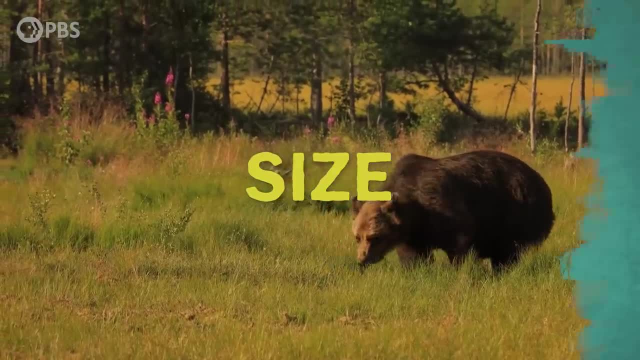 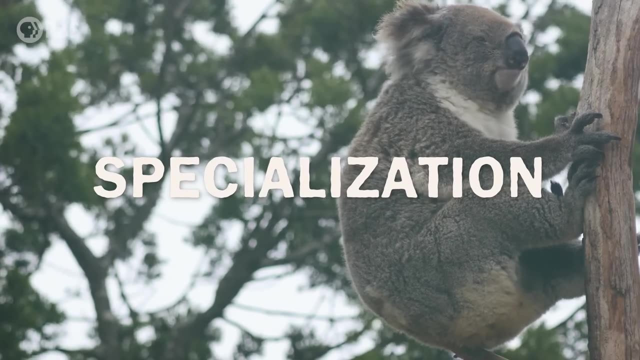 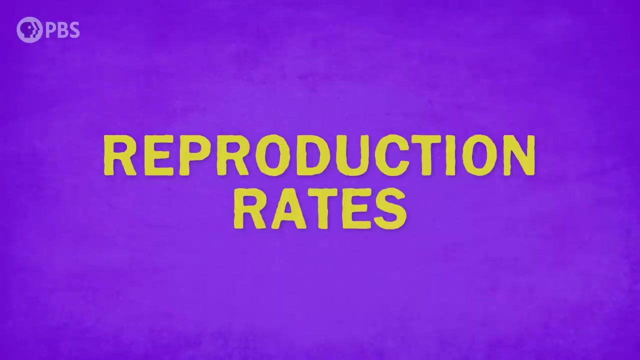 elephants or grizzly bears are at greater risk. Or specialization. Specialized organisms with specific dietary needs or habitat requirements, like maybe pandas or koalas, are also at greater risk And reproduction rates: Organisms who reproduce slowly and require many years of parental care. 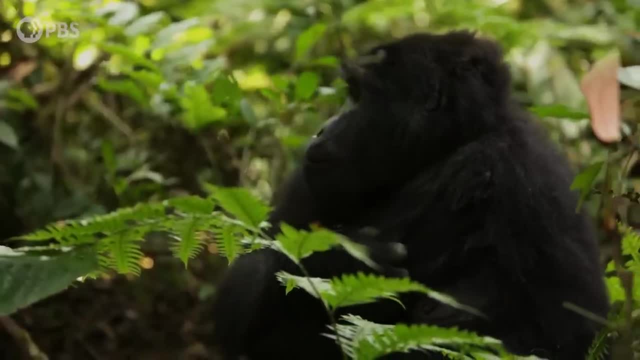 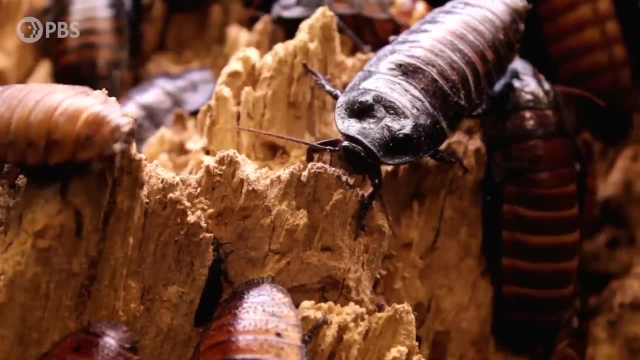 like blue whales or a mountain gorilla, are also at greater risk, Contrast those species with something like a cockroach, which reproduces early and prolifically and are more generalist than specialist when it comes to diet and habitat, Being able to quickly. 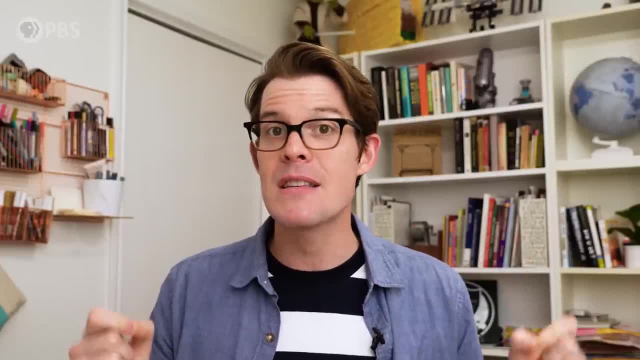 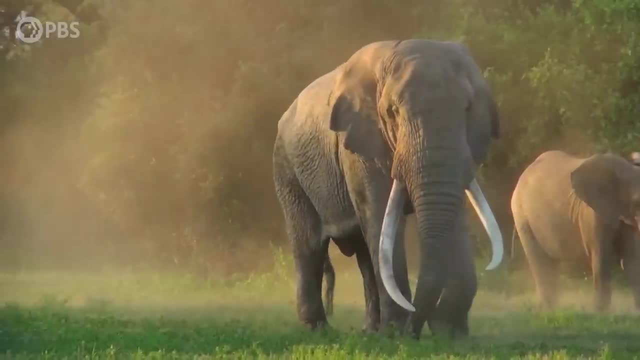 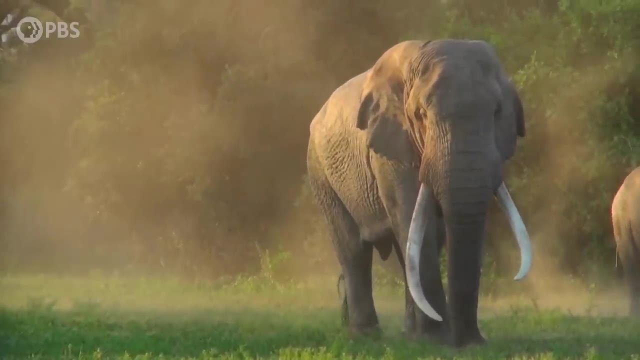 reproduce is an evolutionary advantage that maximizes the chance that a random genetic mutation will help an individual survive a disturbance. An African elephant with its much slower reproduction rate and very specialized habitat does not have that evolutionary capacity for change on a rapid scale. 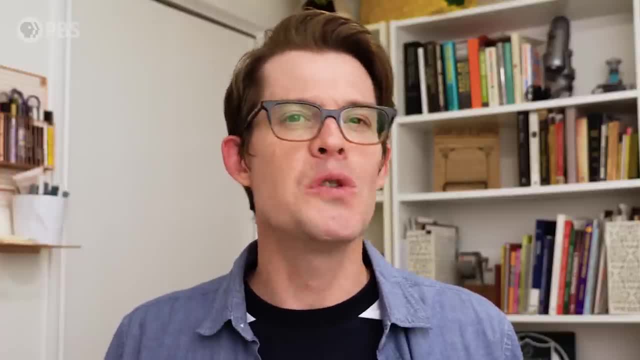 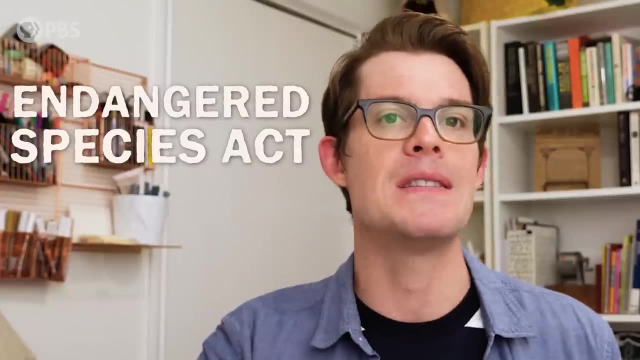 Some species need more protection than others. How do we do that? In the United States, we have the Endangered Species Act, which protects not only the species but also its animals. This is crucial because without its habitat, that species cannot exist in nature. Hopefully. 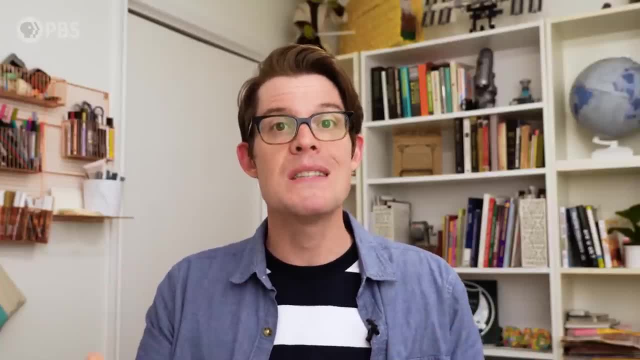 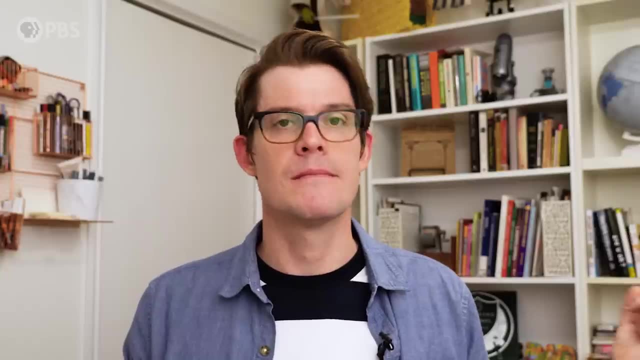 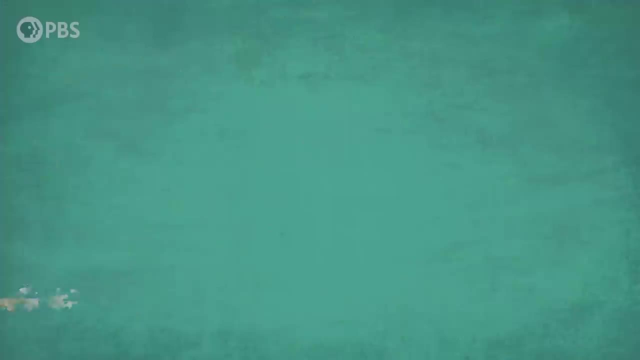 by now I've done my job and showed why it's so important to protect species, habitats and biodiversity. But what are we protecting biodiversity from Us? The main anthropogenic or human threats to biodiversity can be summarized by the acronym HIPCO: Habitat destruction, invasive species population growth. 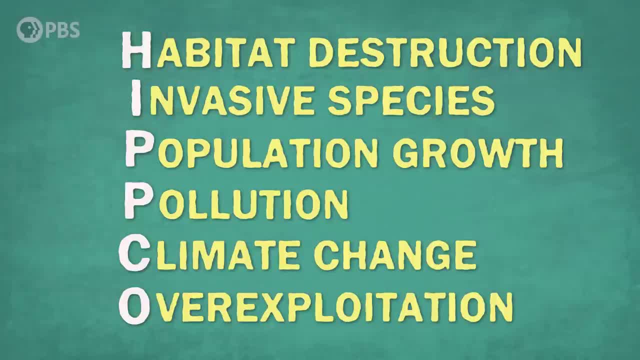 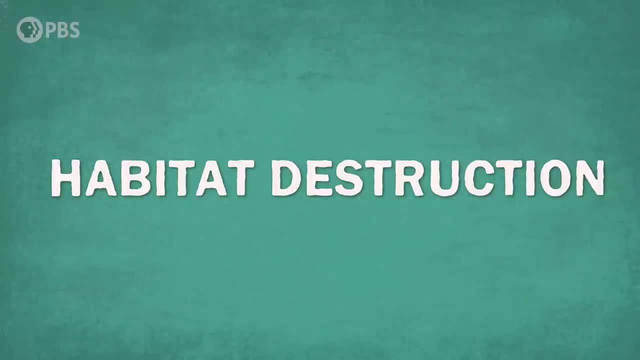 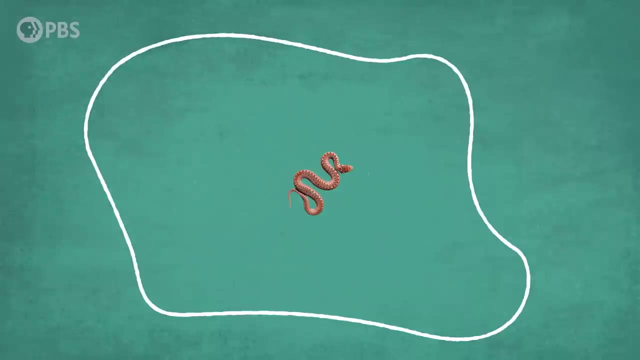 pollution, climate change and overexploitation, Starting with habitat loss. Simply put, if an organism loses its habitat, it cannot survive. Related to habitat loss is the concept of habitat fragmentation. Let's say that this snake requires this much area for its habitat, but then people show up and build a road here, a few houses there. 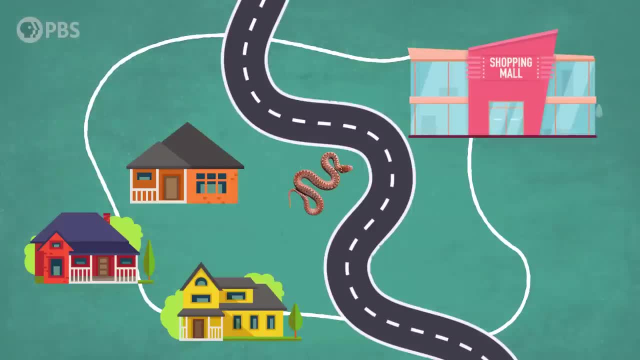 a mall over here. Well, there's still some patches of our snake friend's natural habitat, but they're separated from each other, And this separation in turn reduces the ability of individual organisms to reach each other and will reduce the genetic diversity of the population. 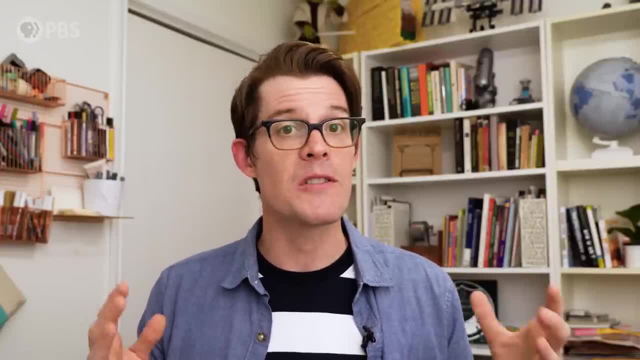 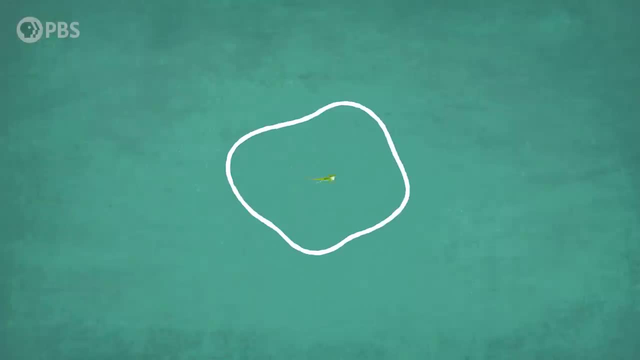 Considering habitat loss and fragmentation, we also need to think about scale. Human land use affects different organisms in different ways. Consider the differences in home ranges between a small anole lizard, maybe no more than 100 square meters, and a grizzly bear. 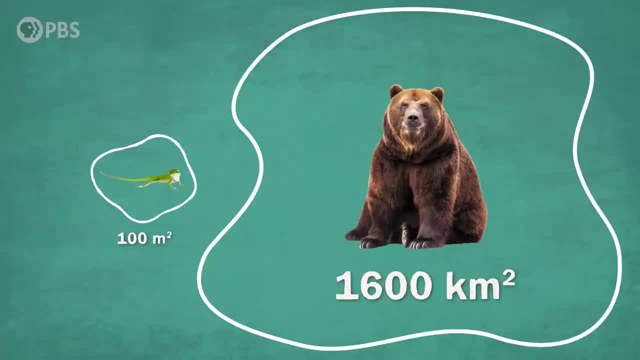 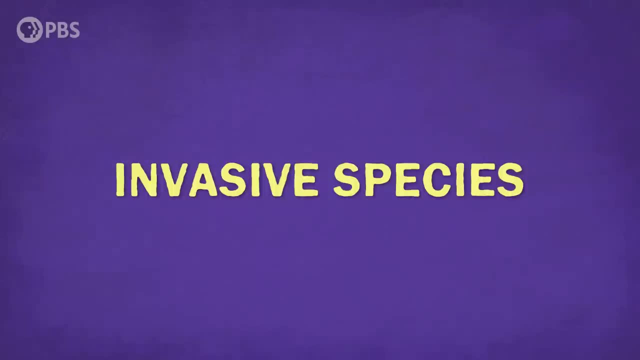 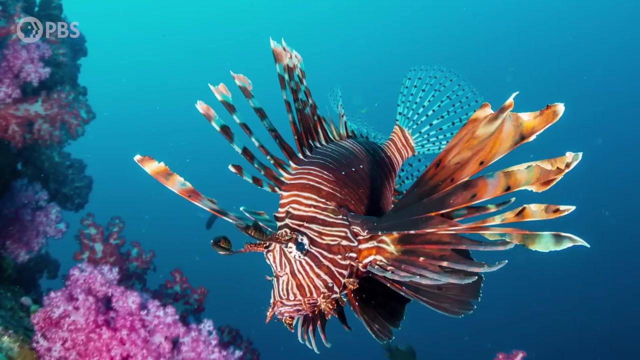 which requires up to 1600 square kilometers of territory. Next, invasive species- Species that are not native to an area but end up there nonetheless, often because of people, are a huge threat to biodiversity: Burmese pythons in the Everglades. lionfish in coral reefs. 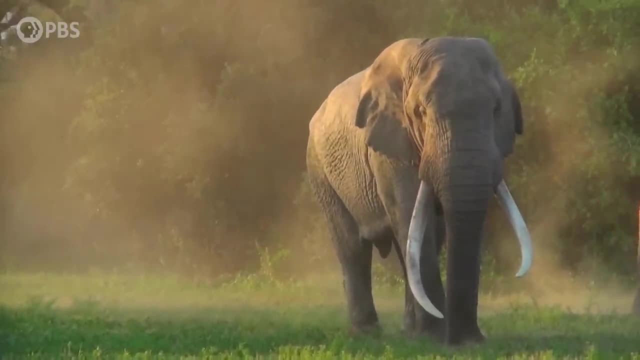 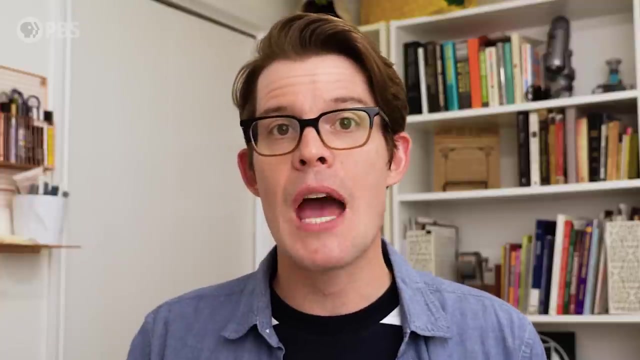 have that evolutionary capacity for change on a rapid scale. So what's the difference? So some species need more protection than others. So how do we do that? Well, in the United States we have the Endangered Species Act, which protects not only the species. 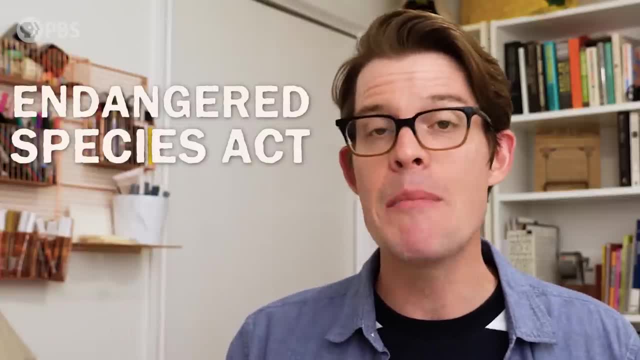 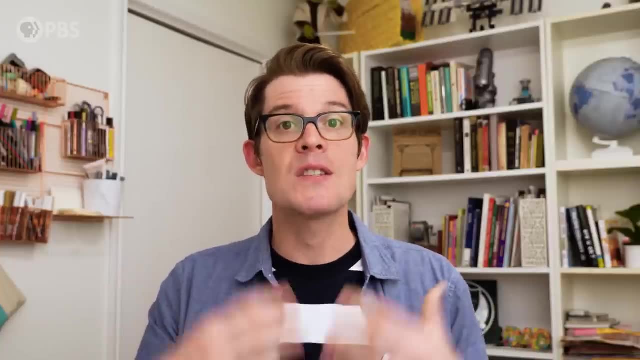 but also its habitat. This is crucial because without its habitat, that species cannot exist in nature. Hopefully, by now I've done my job and showed why it's so important to protect species, habitats and biodiversity. But what are we protecting biodiversity from? 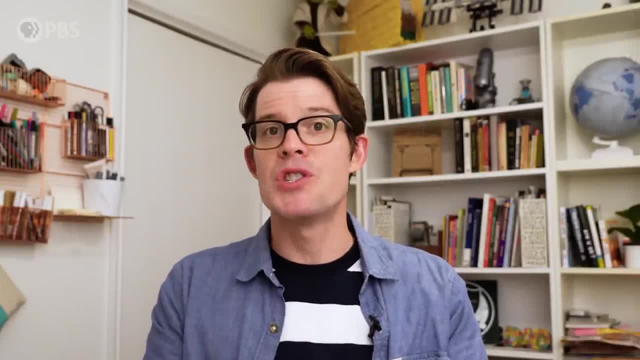 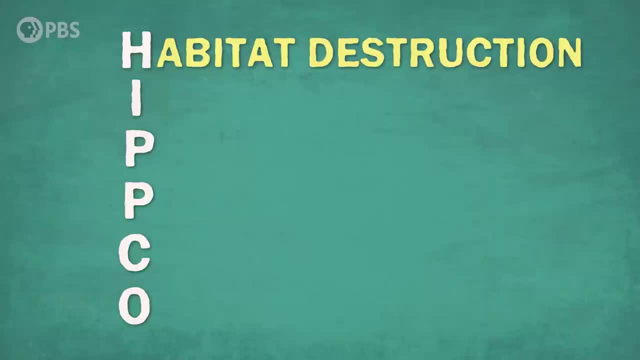 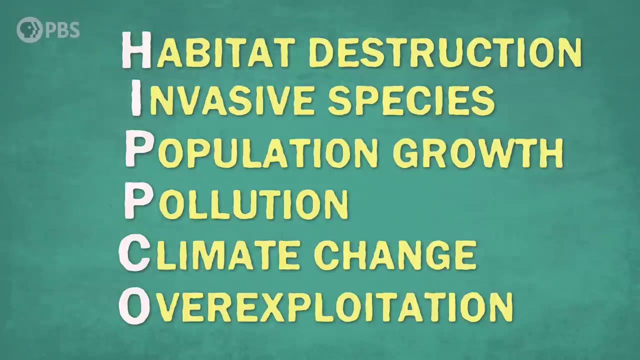 Us Now. The main anthropogenic or human threat to biodiversity can be summarized by the acronym HIPCO: Habitat Destruction, Invasive Species, Population Growth, Pollution, Climate Change and Overexploitation, Starting with habitat loss. Simply put, if an organism loses its habitat, it cannot survive. 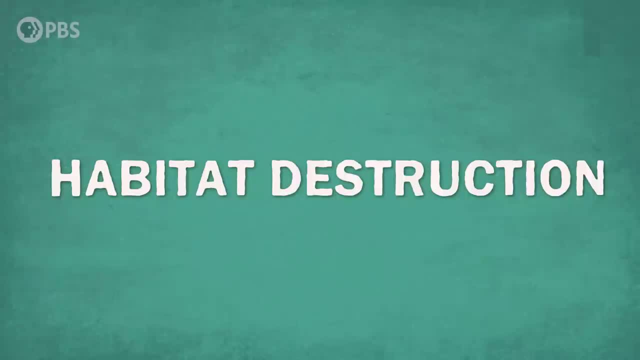 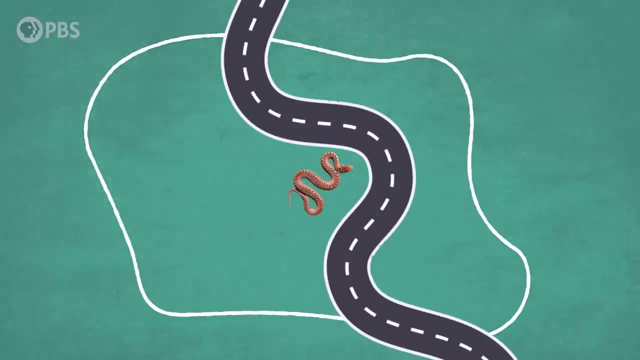 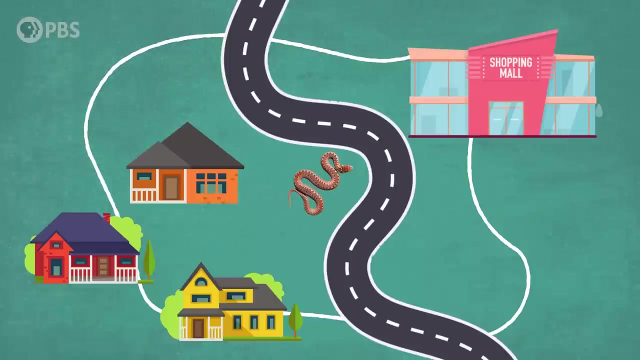 Related to habitat loss is the concept of habitat fragmentation. Let's say that this snake requires this much area for its habitat, But then people show up and build a road here, a few houses there, a mall over here. Well, there's still some patches of our snake friend's natural habitat, but they're. 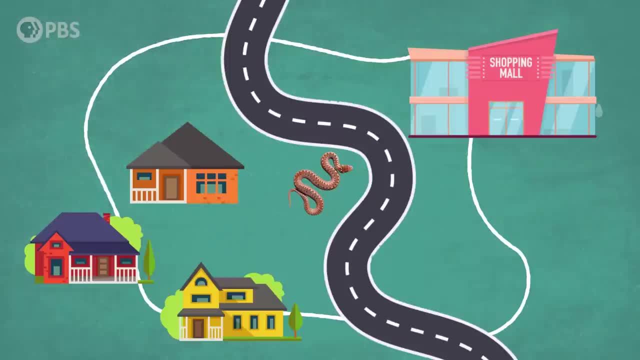 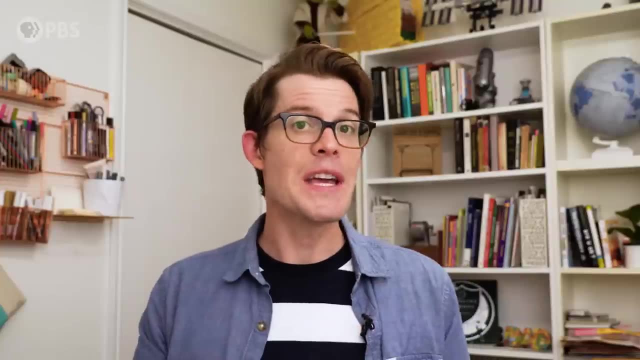 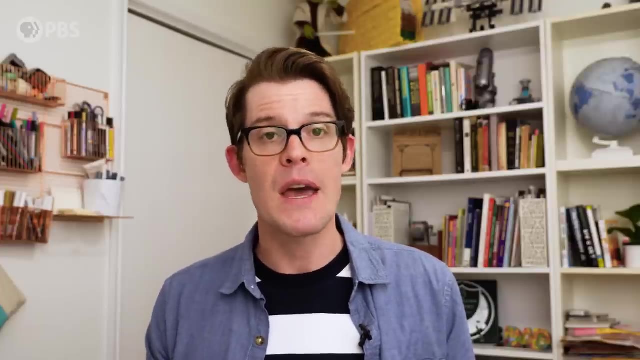 separated from each other. This separation reduces the ability of individual organisms to reach each other and will reduce the genetic diversity of the population. Considering habitat loss and fragmentation, we also need to think about scale. Human land use affects different organisms in different ways. 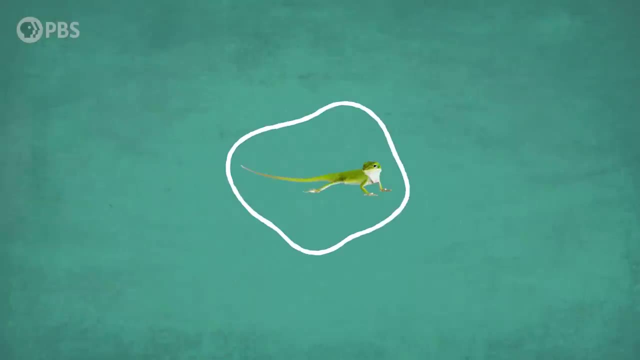 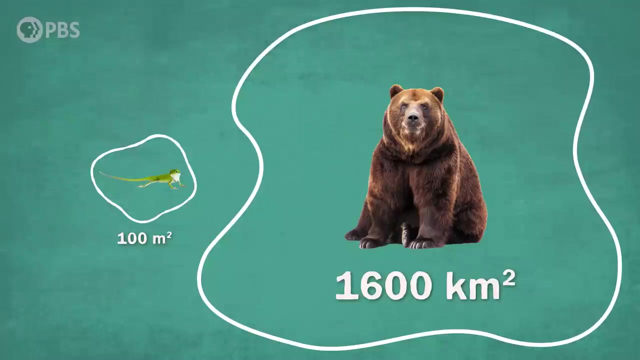 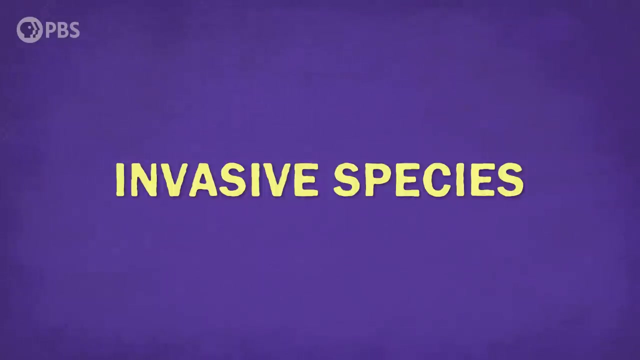 Consider the differences in home ranges: Ranges between a small anole lizard, maybe no more than 100 square meters, and a grizzly bear, which requires up to 1,600 square kilometers of territory. Next, invasive species: Species that are not native to an area but end up there nonetheless, often because of. 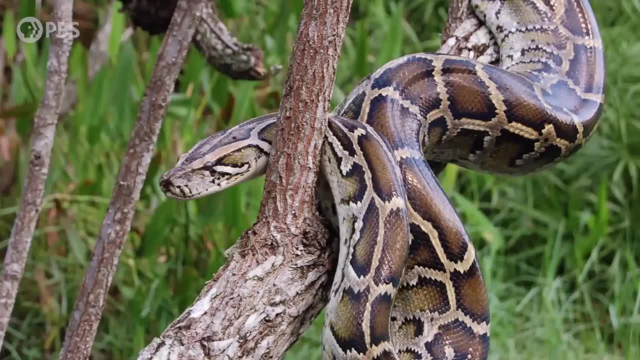 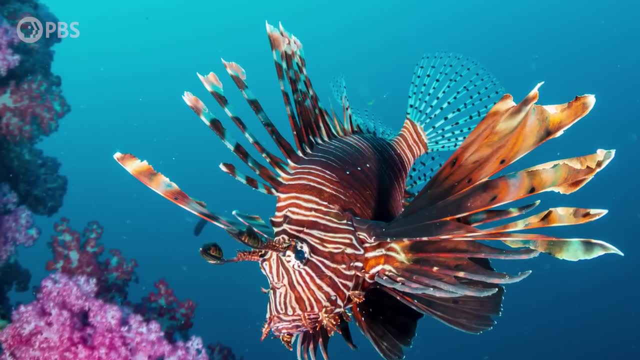 people are a huge threat to biodiversity. Burmese pythons in the Everglades, lionfish in coral reefs- both of those are actually a result of humans releasing their pets. Or even kudzu vines In the southeastern US, an imported plant pet that escaped gardens. 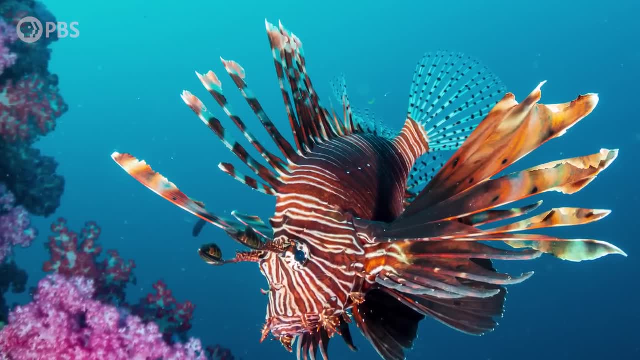 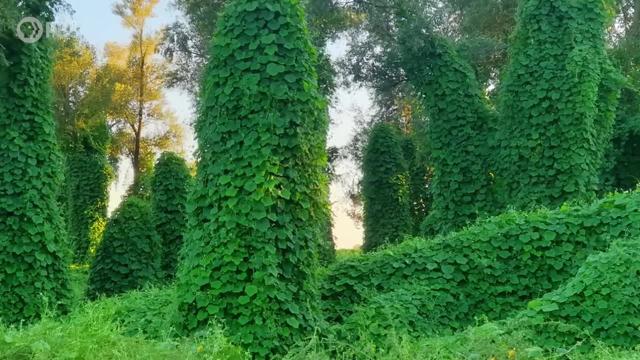 both of those are actually a result of humans releasing their pets, Or even kudzu vines in the southeastern US, an imported plant pet that escaped gardens. These are all invasive species. Because they usually don't have natural predators in their new environments, populations of invasive species can explode. 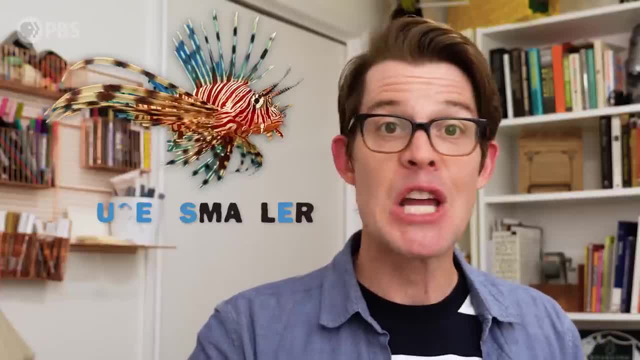 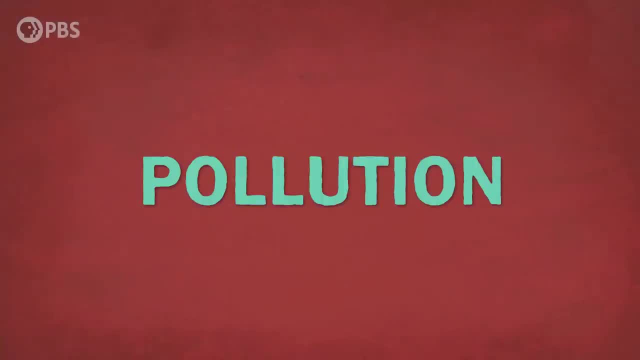 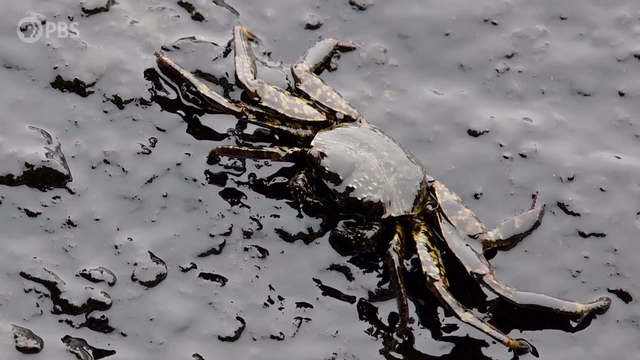 The presence of lionfish can reduce the number of smaller fish in a coral reef by almost 80%. On to pollution, which is both a visible and invisible threat to biodiversity: You can see an oil spill actively harming wildlife and damaging habitats, but a lot of pollution isn't quite as obvious, like sulfur or lead in the air. 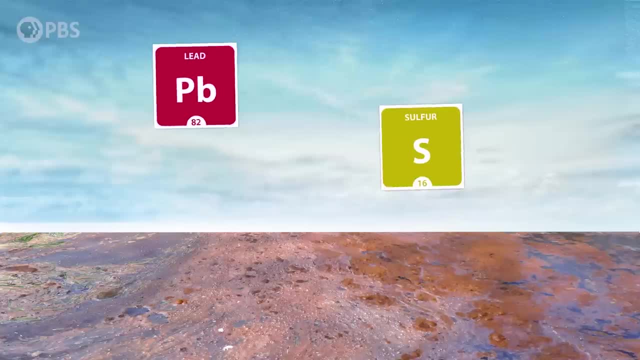 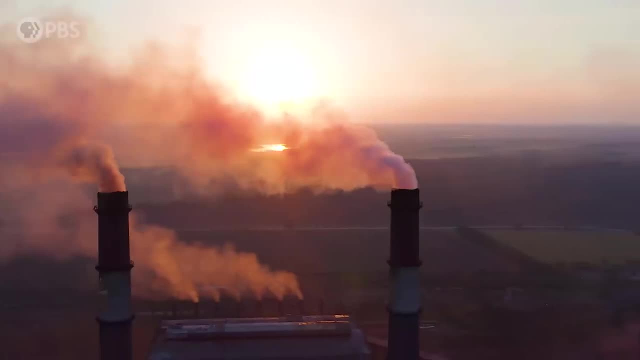 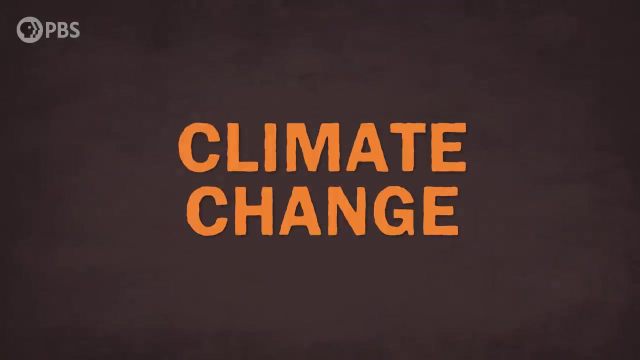 or pharmaceuticals and toxins in the water, But one of the greatest sources of pollution right now is the use of fossil fuels, When burned oil, gas and coal release tons of air pollutants and dangerous greenhouse gases that lead to climate change. Climate change is the focus of this entire channel and it'll get its own episode. 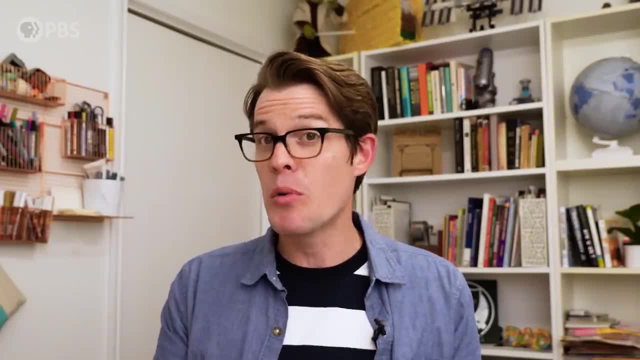 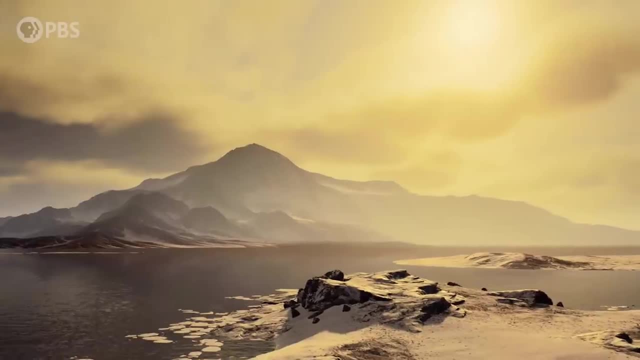 in this series, but I want to point out right now that global warming and climate change are affecting more than human lives. Rising temperatures, more acidic oceans and the many other impacts of climate change are also affecting wildlife biodiversity in a huge way. Coral reefs. 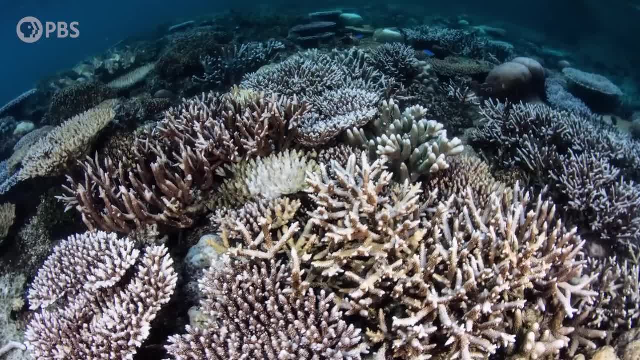 are bleaching at an increasing rate and they're also affecting wildlife biodiversity in a huge way, As warmer ocean temperatures cause tiny coral animals to expel their symbiotic allergy that provide them with the majority of their food After a bleaching event. 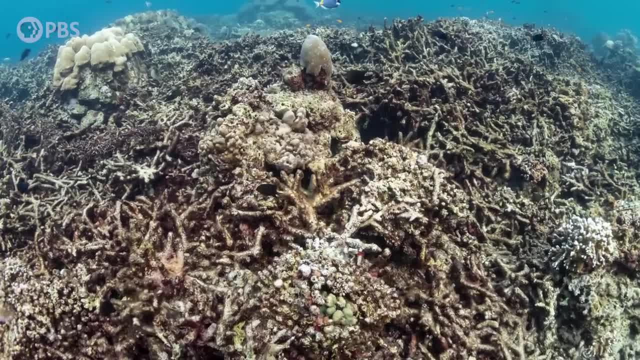 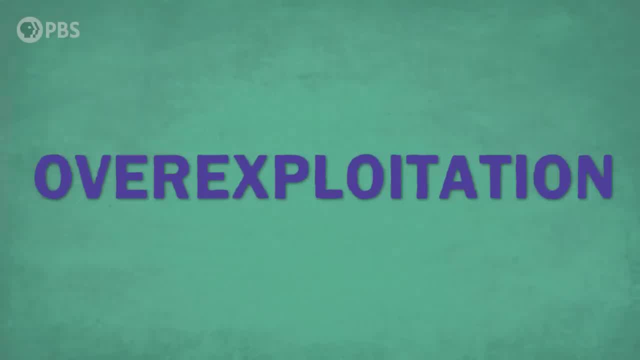 if the algae don't come back, the coral will die. Finally, using living natural resources at a faster rate than they can reproduce is over-exploitation. Catching fish quicker than they can make baby fish collapses fisheries and the related fishing industry that relies on them. 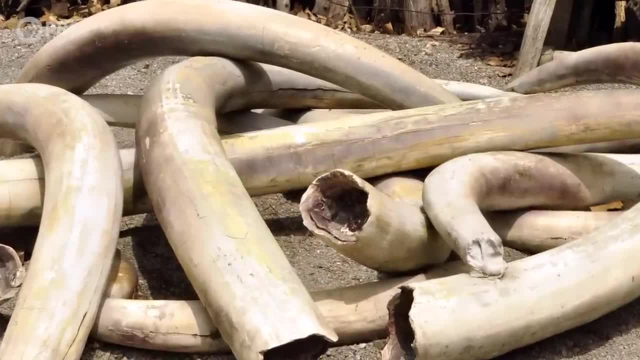 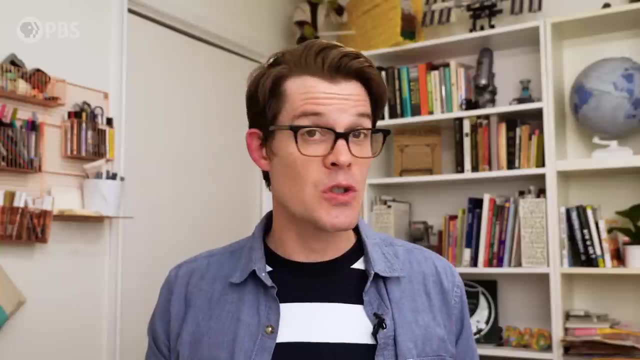 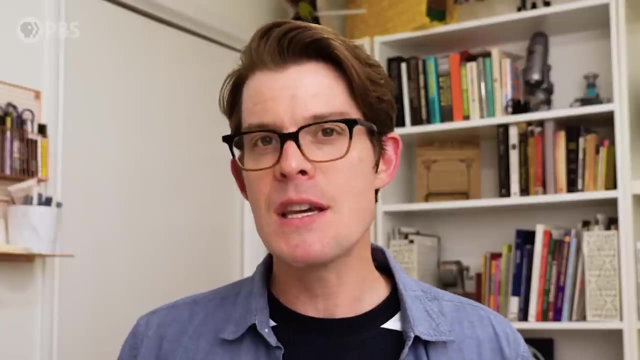 Killing elephants for their ivory will decimate a population quicker than it can repopulate. When environmental science can identify over-exploitation, laws, policies and international treaties can come in to help regulate our consumption of those resources and protect biodiversity. As you can see, environmental science is a large and diverse. 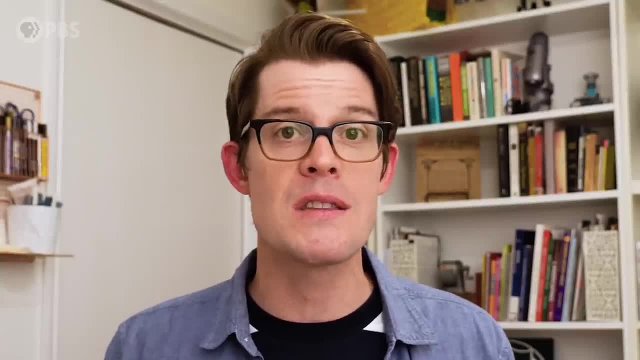 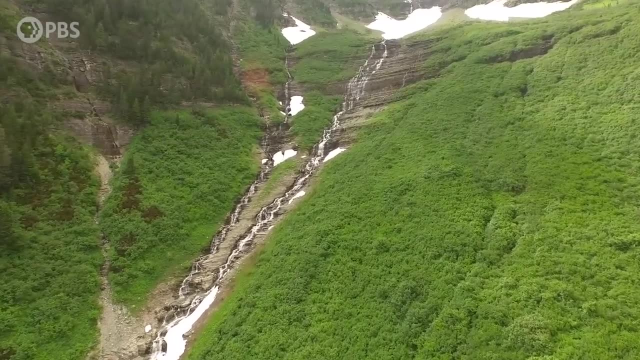 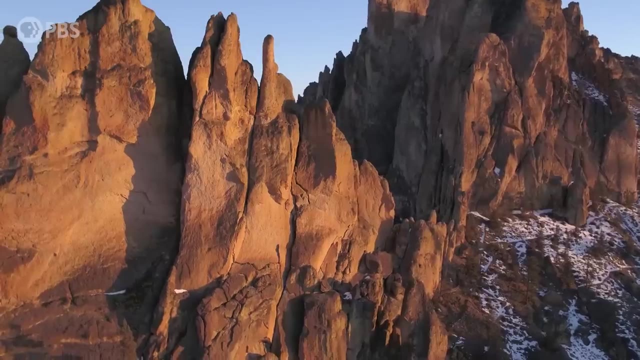 field of study that encompasses many different scientific disciplines at various scales, from the microscopic to the macroscopic, Which is pretty fitting, because the environment itself is this thing that is everywhere, And while one of the main lessons you should take from these videos is that humans are not separate from these natural 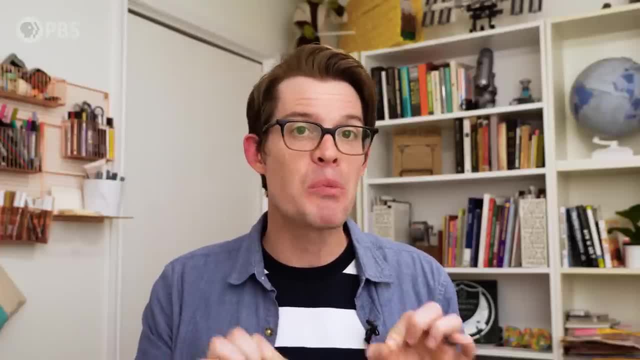 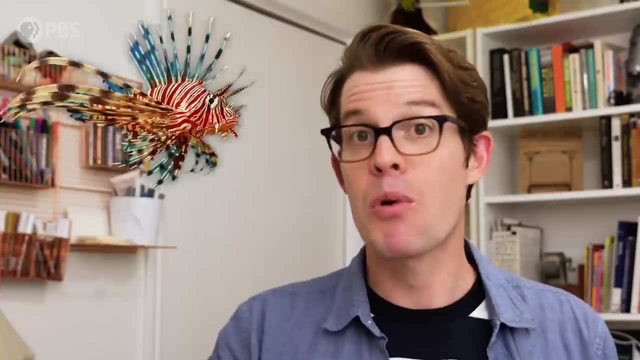 These are all invasive species Because they usually don't have natural predators in their new environments. populations of invasive species can explode and outcompete native species. The presence of lionfish can reduce the number of smaller fish in a coral reef by almost 80%. 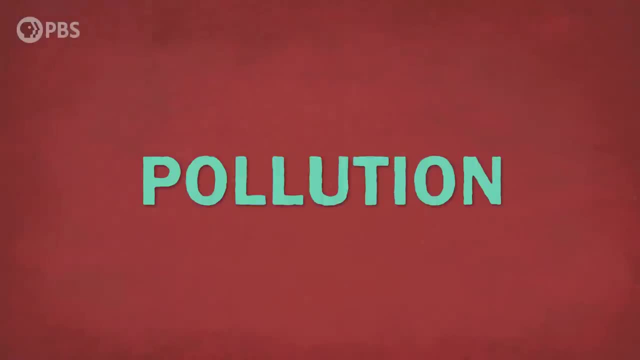 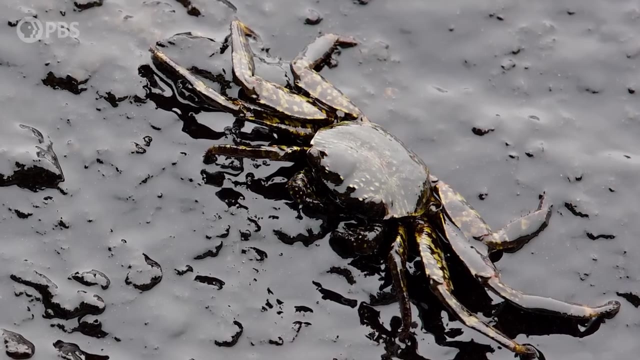 On to pollution which is both a visible and invisible threat to biodiversity. You can see an oil spill actively harming wildlife and damaging habitats, But a lot of pollution isn't quite as obvious, like sulfur or lead in the air or pharmaceuticals. 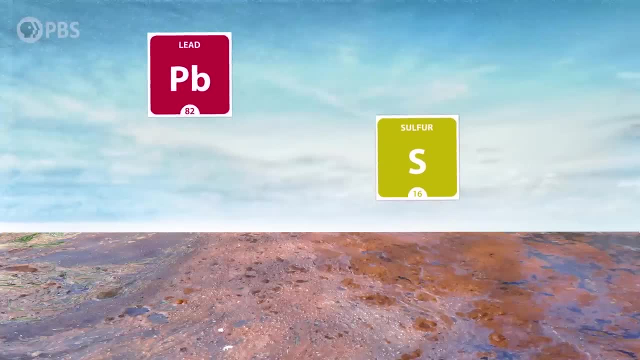 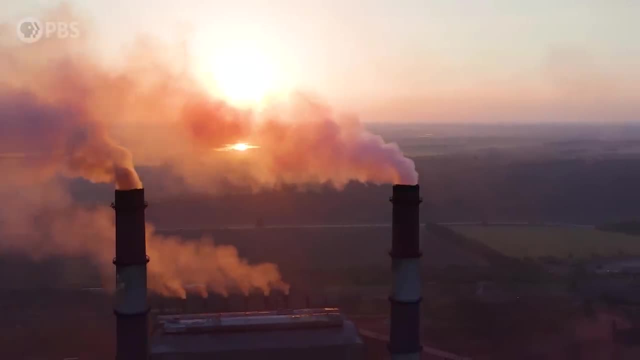 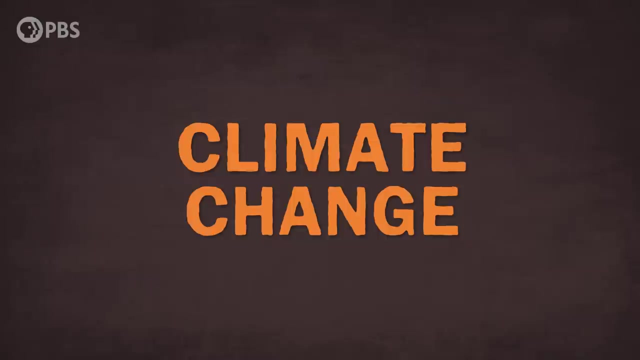 and toxins in the water, But one of the greatest sources of pollution right now is the use of fossil fuels. When burned oil, gas and coal release tons of air pollutants and dangerous greenhouse gases that lead to climate change. Climate change is the focus of this entire channel, and it'll get its own episode in. 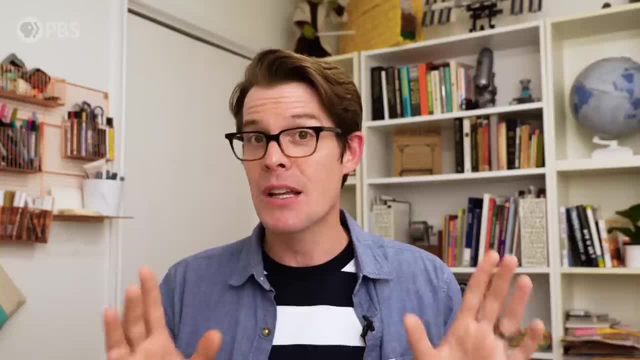 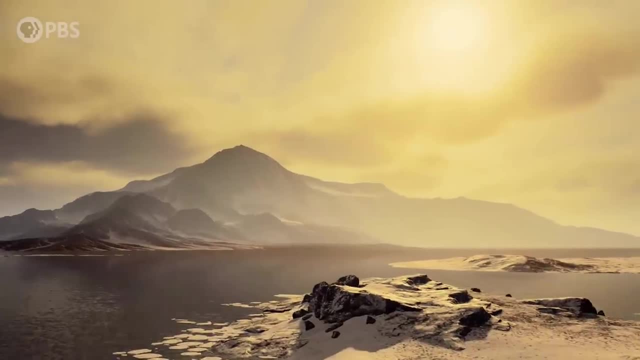 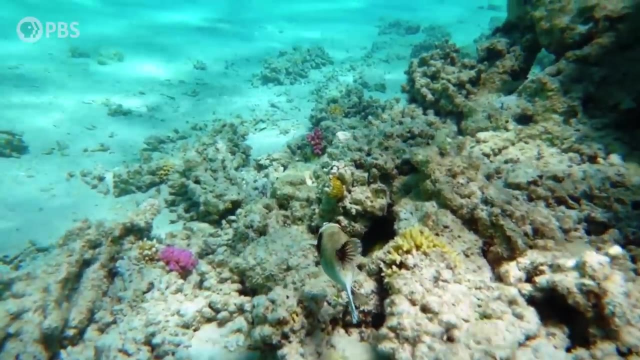 this series, but I want to point out right now that global warming and climate change are affecting most of our lives. Rising temperatures, more acidic oceans and the many other impacts of climate change are also affecting wildlife biodiversity in a huge way. Coral reefs are bleaching at an increasing rate as warmer ocean temperatures cause tiny 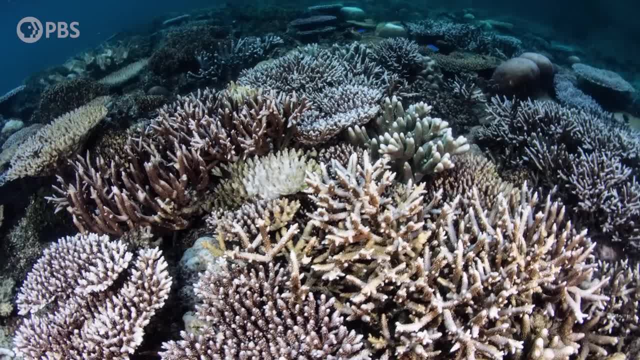 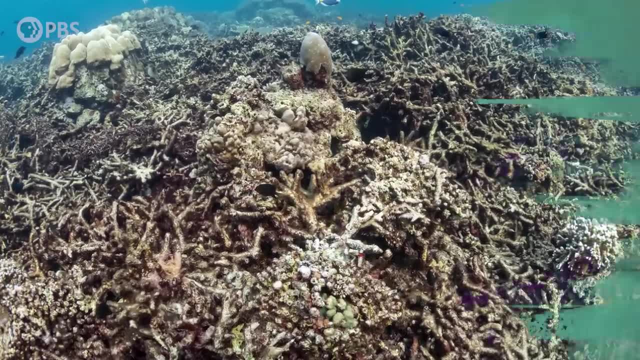 coral animals to expel their symbiotic algae that provide them with the majority of their food, And, after a bleaching event, if the algae don't come back, the coral will die. Finally, using living natural resources at a faster rate than they can reproduce is a 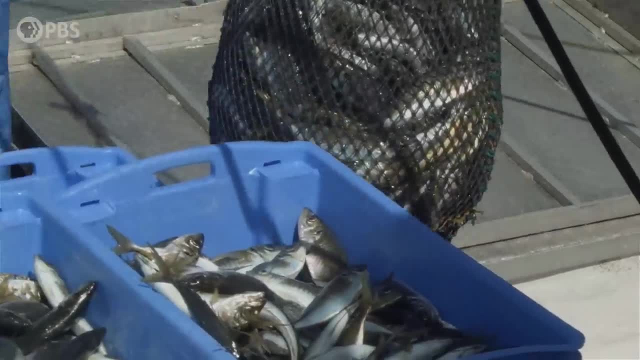 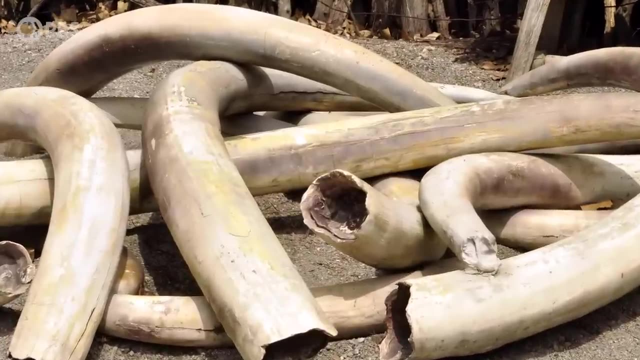 great way to reduce the risk of over-exploitation. Catching fish quicker than they can make baby fish collapses fisheries and the related fishing industry that relies on them. Killing elephants for their ivory will decimate a population quicker than it can repopulate. 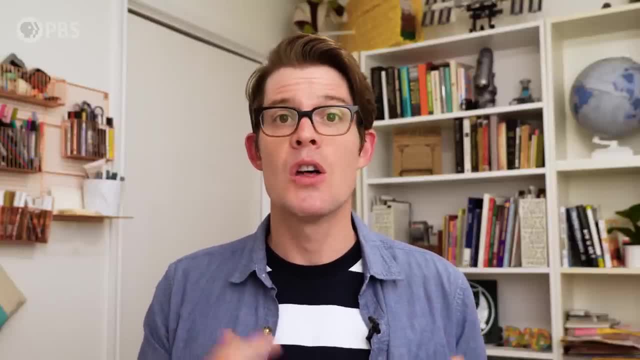 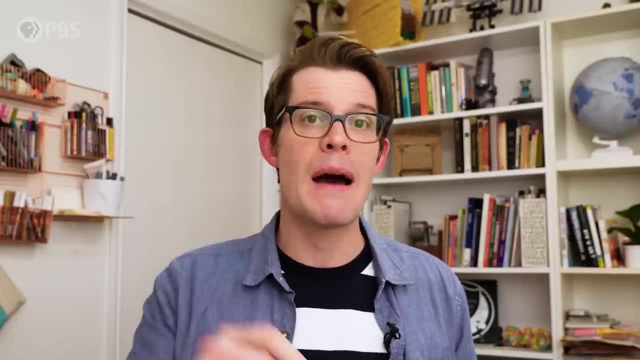 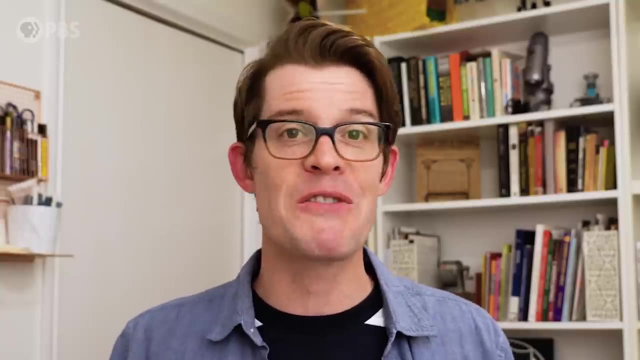 When environmental science can identify over-exploitation, laws, policies and international treaties can come in to help regulate our consumption of those resources and protect biodiversity. So, as you can see, environmental science is a large and diverse field of study that encompasses many different scientific disciplines at various scales, from the microscopic 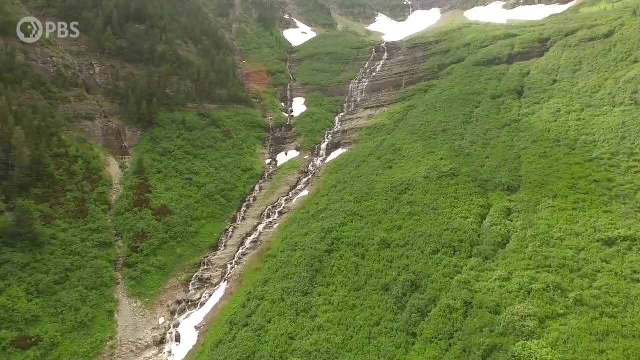 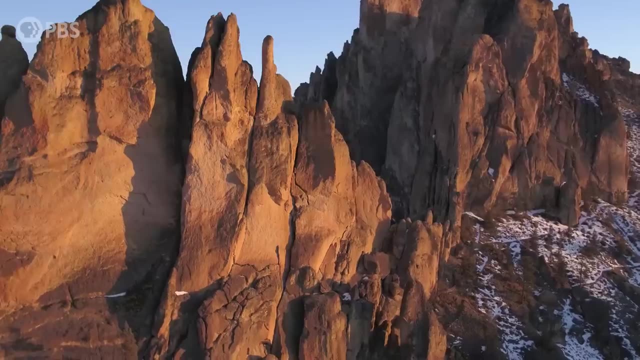 to the macroscopic, Which is pretty fitting because the environment itself is this thing that is everywhere. And while one of the main lessons you should take from these videos is that humans are not separate from these natural systems, we are in a unique position to study them, for.